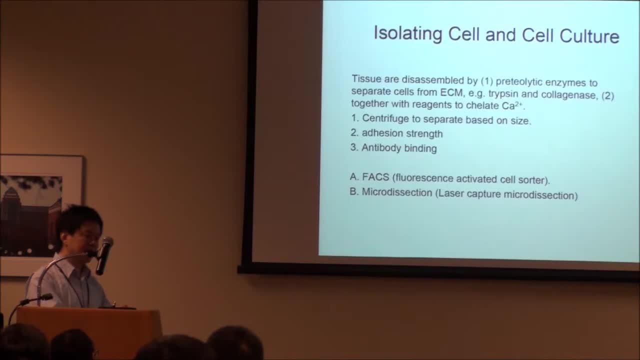 Because we all know, in the body all these cells are attached to a lot of matrix proteins and connect to each other as well. right, How do you select and separate these cells? This is the first step. So these enzymes can, They can digest the cell membrane receptors so that they can be detached from the extracellular matrix proteins. okay, 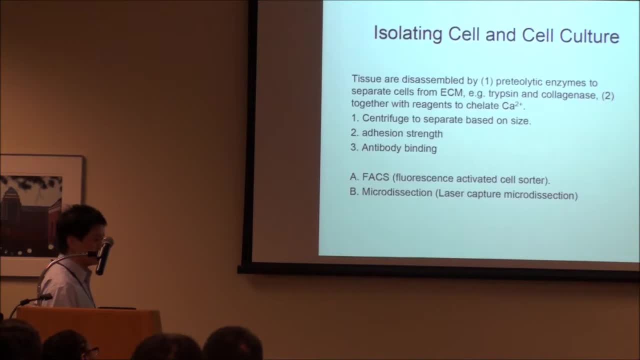 And when you add these enzymes- usually when you're doing cell culture- you probably know you usually also add so-called chelators for calcium. Why people add a chelator for calcium? Mainly because you know the cells connect to each other, right? 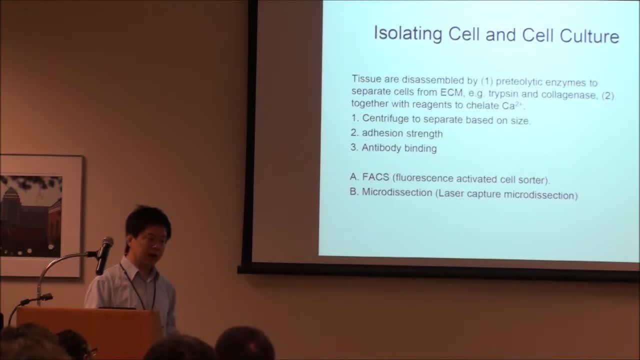 You have to detach cells from each other, And calcium is a major molecule So it helps the cells to connect to neighboring cells. So if you chelate calcium then the cells will detach from each other. okay, So this enzyme will detach the cell from the matrix and the calcium chelator will detach the cell from each other. okay, 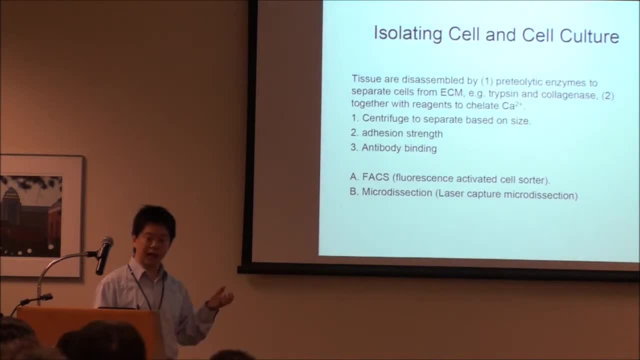 So with these two things together, the cell will become isolated, single cells. okay, So this is the separation. After you separate and detach, all the cells become single cells. You still need to collect a specific type of cell you're interested, right? 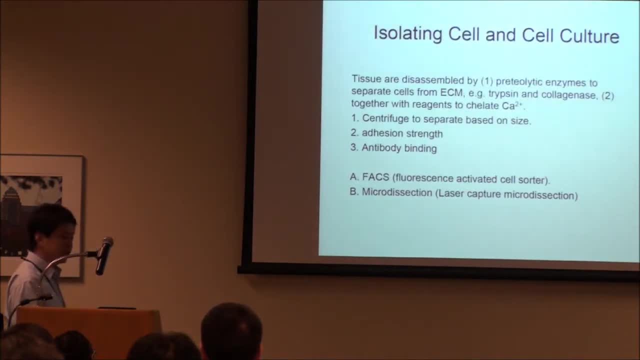 And usually that's the several. you know technology people use. One is centrifuge, so-called Basically based on different type of cell size, okay, Or maybe their weight. you can use centrifuge with different speed and you can collect different type of cells. 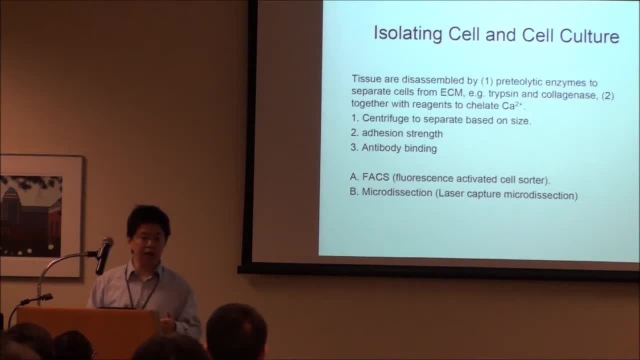 Second is adhesion strength Because it's already known, many different cells, they have different adherence strengths. So if you culture, for example, into the dishes for different times, the different type of cell will attach to the surface. For example, for five minutes, probably fibroblast will stick okay. 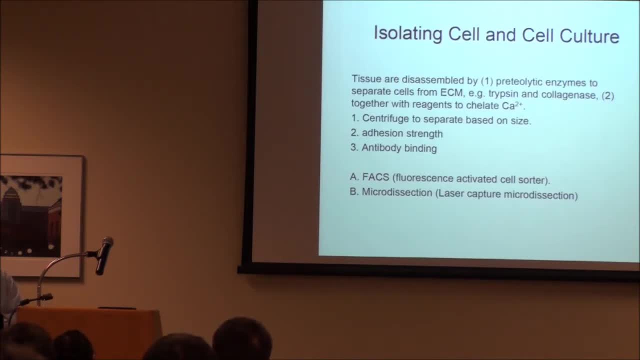 But other blood cells will take longer. for them, to you know, adhere on the surface So you can wash away. for example, after five minutes you wash away, the other type of cell will be gone, Only fibroblast will be collected. okay, 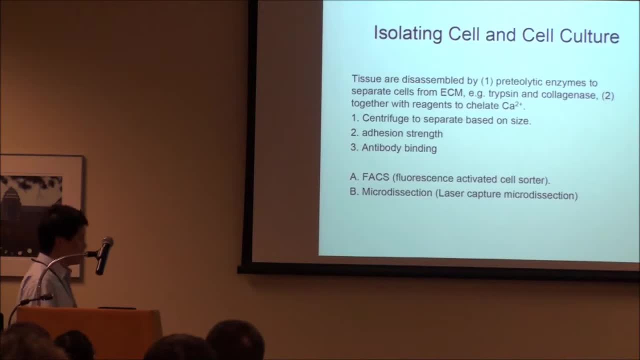 That's based on adhesion strength. But all these, like the first one or two. the methods are not that specific Because a lot of cell, different cell type, their adhesion strengths could be very similar. So, five minutes you probably collect two or three type of cells. 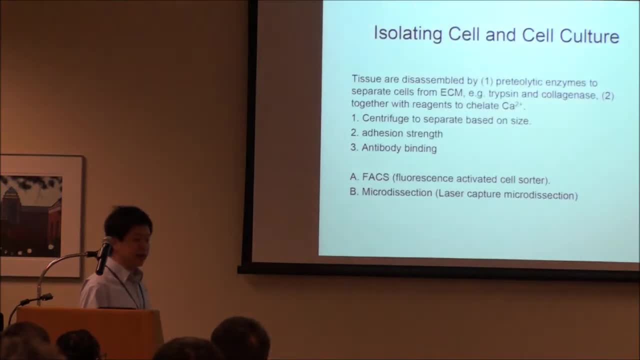 And the most accurate one is so-called antibody binding. If you already know certain specific cell type you are interested and you know this cell type is expressing specific protein on the surface, you can use antibody to bind to it right. Attach antibody to a bead if you do centrifuge and this specific cell type will be pulled down. 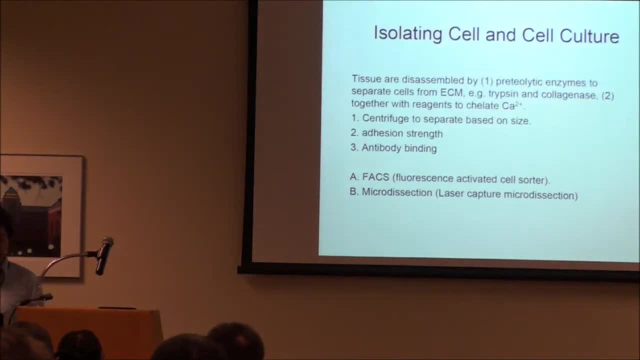 Okay, So that's called antibody binding And that's more specific. You can pretty much target a specific cell type you are interested. Okay, So these are general principles, how to isolate cells, to purify cells, And these are the specific technology or machines you can utilize. 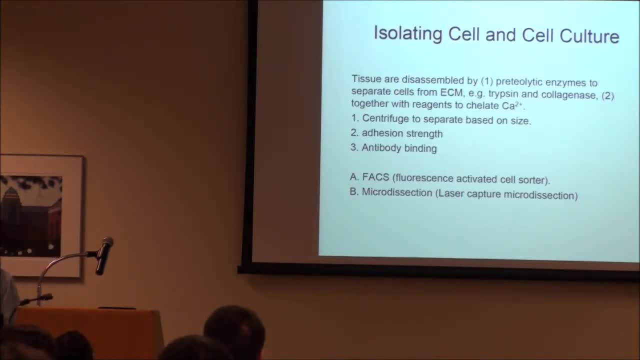 One is called fluorescence activated cell sorter. Okay, How many people already heard about this FACS machine to purify cells? Okay, Very good, There are already, people know. And the second I'm going to talk is about microdissection. 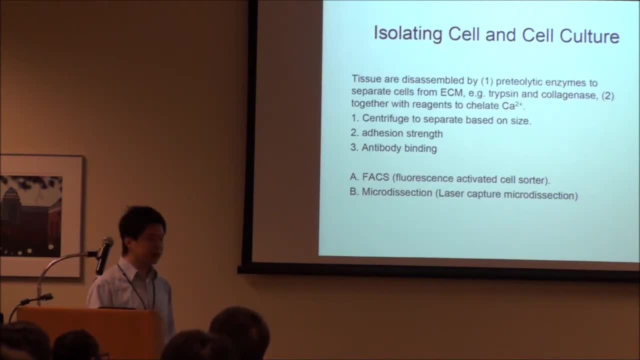 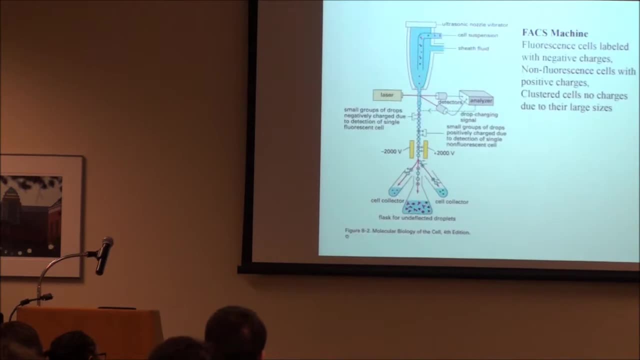 Okay, Basically, this utilizes laser power to cut the tissue and capture a specific group of cells. Okay, So this is the fundamental mechanism for FACS machine to work. Okay, So, as we discussed right now, you know how to add a different reagent to separate the cells. 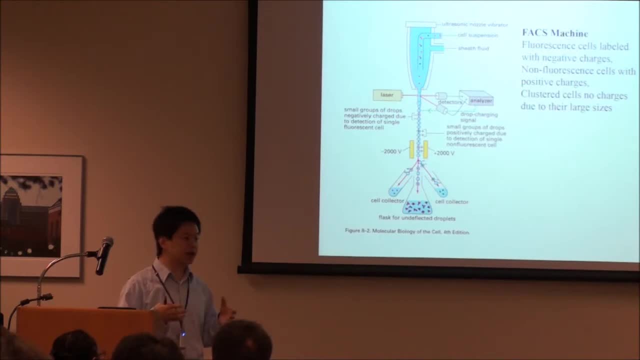 so that they become single cells. Okay, So you collect the whole population of the cell And you can even add antibodies to label a specific cell type. you are interested, Right, And how do you select these specific labeled cell type? For example, we already have antibody with different fluorescent colors. 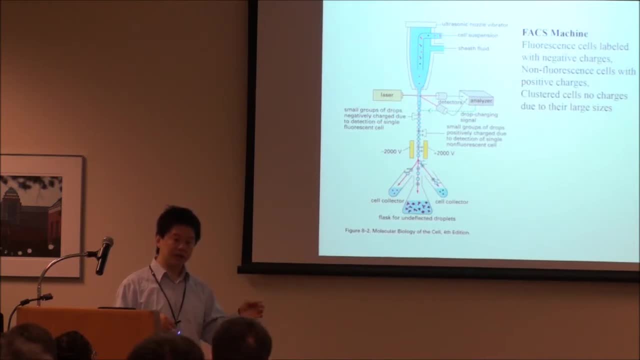 Right To label the specific cell types. How do you separate them physically? That's the FACS machine comes to play. So what you can do, you can have this reservoir system And you can fuse in the cell suspension. Of course it's a mixture of different type of cells. 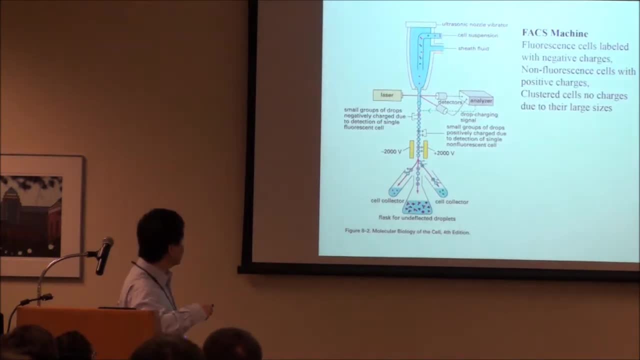 Right After you, directly, you know, purify from tissue And there's a so-called sheath flow. Okay, It's wrapping up these, you know tubes And these will have start a flow passing through these long, narrow channels. 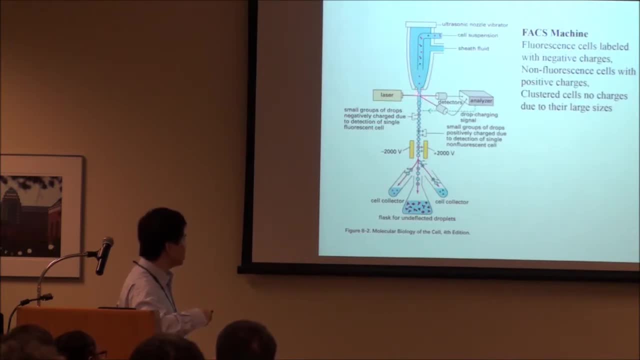 Okay, During this pathway there's laser shining continuously on this line. on this point, Whenever there's a cell pass here based on the antibody labeling you already did, Right, If it's labeled with specific type of antibody, you are interested. 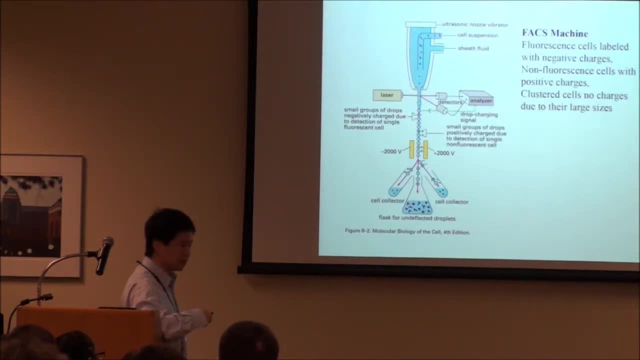 it will label with different- you know- charge. Okay, Whenever there's detection of antibody, it will label with a charge at this point, Okay, Because the flow and the distance are all precisely controlled. Okay, When you detect a cell, you are interested. 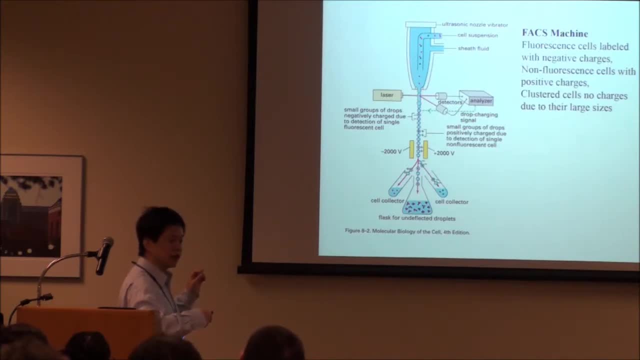 at this point it will tell: based on the color or based on antibody it detected, it will design specifically A specific charge. Okay, So now, after you pass this point, the cell type you are interested is already labeled with specific charge. 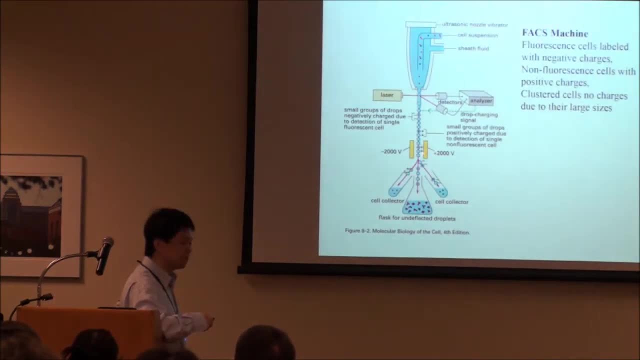 Okay, And they will pass this. you know electrode field: Okay, So you can imagine if they pass it, the specific charge of the cell will be go to different. you know tubes, Right? For example, if the cell you are interested is charged with negative charge. 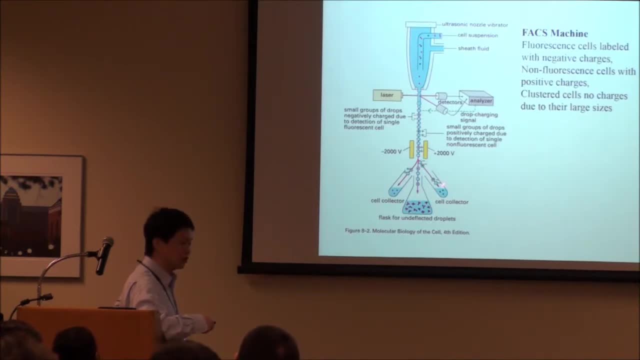 it will go to this. you know, right tube. So you basically collect the specific charge, The specific cell type. you are interested already. Okay, All the other things. if they are not charged, they will go to, you know, the central so-called waste tank. 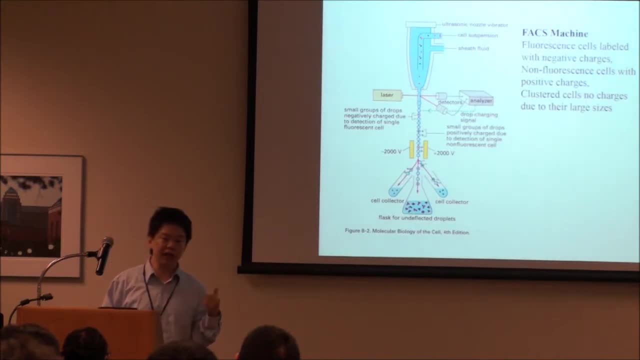 Okay. Is it clear for the mechanism How you can utilize a fax machine to collect cells? Question: Is there any limit of the size of the cells that can be separated using this process? Yes, of course. So this will depend on the size of these. you know nozzles. 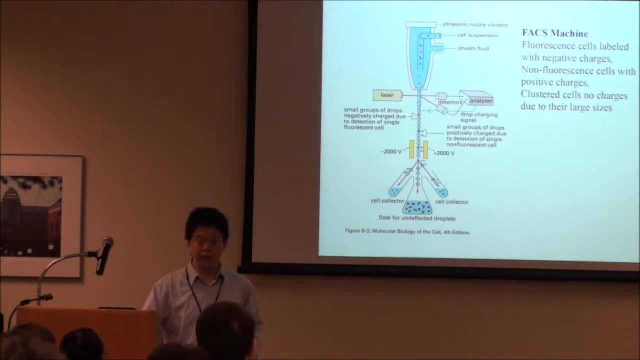 Usually like 10, 20 micrometer will be no problem, But if it's too big, like 100, maybe it will be difficult. It will be stuck in the middle sometimes. So what you are saying is that you are using the laser. 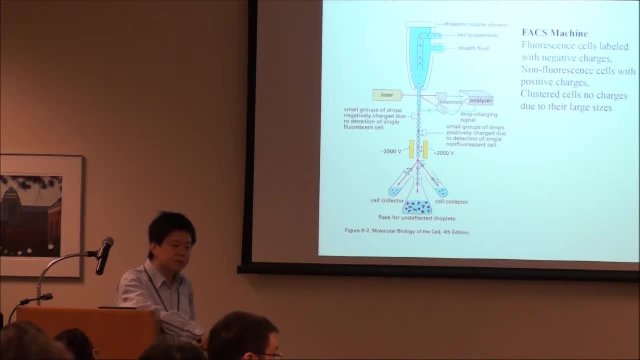 to ionize the antibody with which you label the cells? No, No. So basically, laser is only serving as a detector. Okay, So laser, for example, will shine right And you can see antibody labeling and color labeling And it will tell this. you know? detector analyzer. 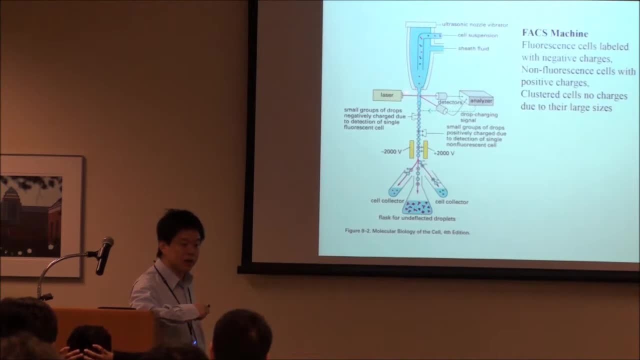 It tells: okay, there is a cell coming with specific, you know, antibody labeling And when they pass through and reach this point it will be assigned a specific charge. So the charge and the laser are separated. This laser is detector and this is, you know. 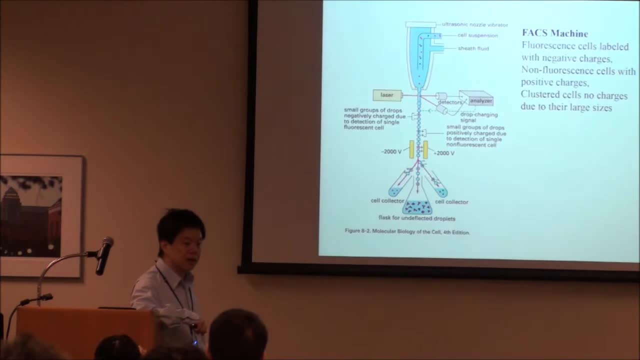 application site for the charges. Is it clear? Because this distance is fixed right And the flow rate is fixed, So is the antibody fluorescent. Yes, you can do that Exactly. I'm trying to understand the meaning of the word fluorescent. 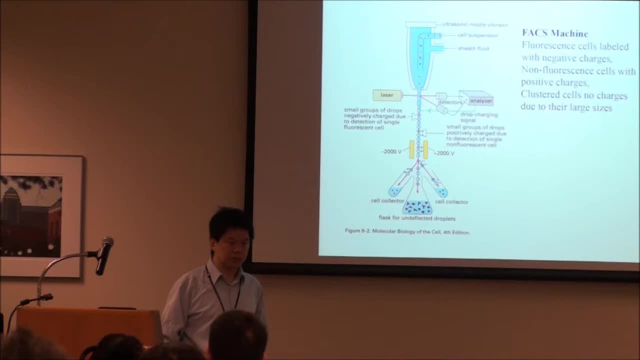 Where is the fluorescence in this whole process? Yes, Antibody can be attached to fluorescence. That's the easiest way. So whenever laser detect a cell with fluorescence, Okay Right, Antibody, And it will tell this site to apply a charge. 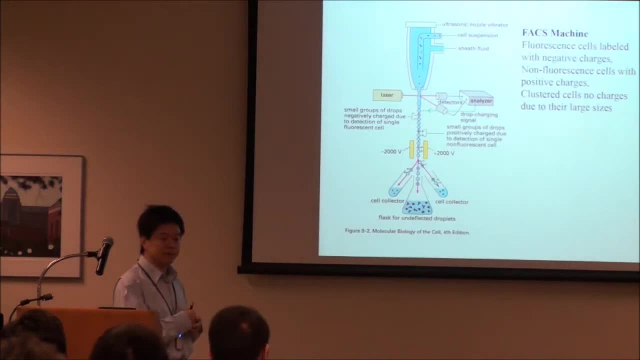 Then you know this cell has to go to a specific tube. Okay, Can you attach nanoparticles and use them with the flexible? Oh yeah, That's a perfect idea, Although it's not, you know that popular yet, but definitely it can be. 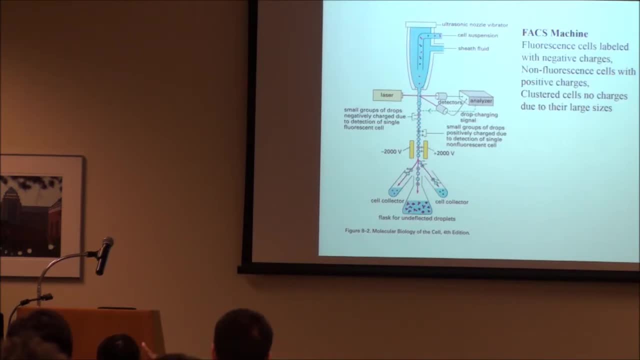 It can be done. Okay, With the effects machine. you think of the nanoparticles in itself. Is there a size limit? Oh yes, There's 10, 20 microns, So nanometer will be no problem at all. So when laser like identify the certain cell, 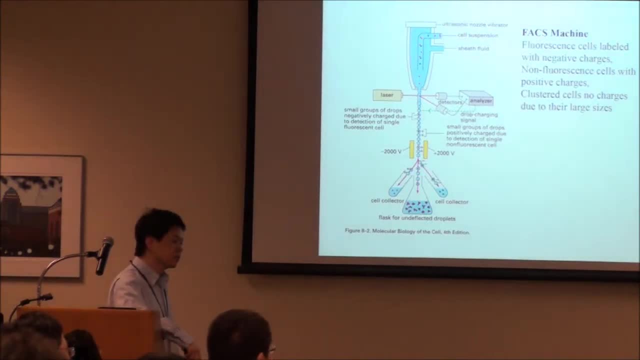 it will label, for example positive charge, And then it identify it detects some other type of cell. it just put negative charge. You can do so If you have multiple. you know colors, For example one specific cell type using green color, right. 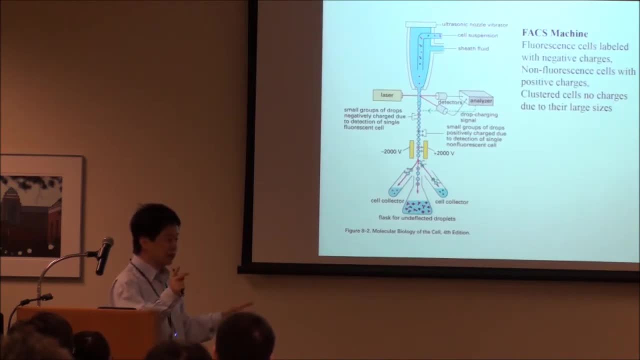 Well, another cell type uses a redder color. for example, Two antibodies right, Two different antibodies, And when they go through these laser detect and find out green, it will give negative charge. If they see a red, they can give a positive charge. 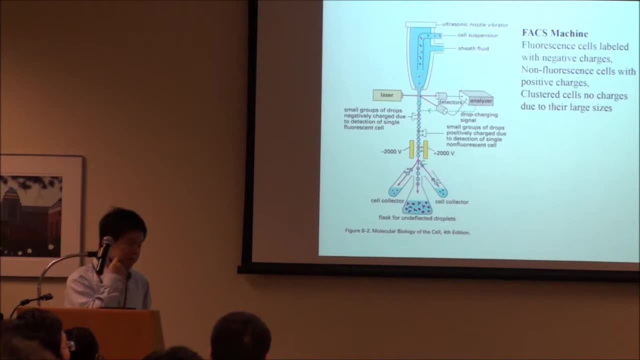 How about like two type of cell mixed together? Oh, you mean you want to collect two type of cell together? Yeah, I mean you have. you want to like separate the cell, but they are mixed together So when laser detect they can detect like both. 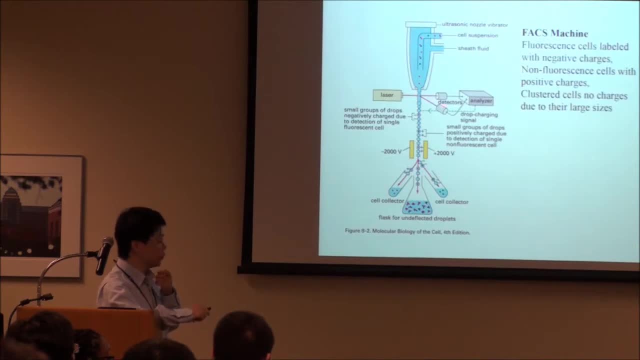 And then like: how do you determine? how do you? Yeah, if you know, for example, there are two cells stick together, green and red together, right, It would detect. okay, it's a yellow color, for example. right, 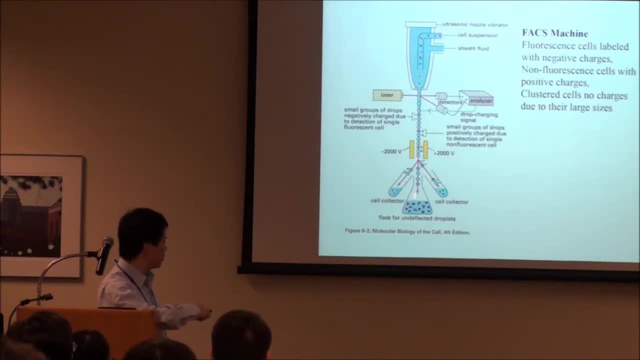 Mixed together And they will not apply any charge and go to, you know, direct to go there. Okay, Only the single cell with purity will be collected. Okay, thanks, Okay. So the application of the sorting of the cells is. 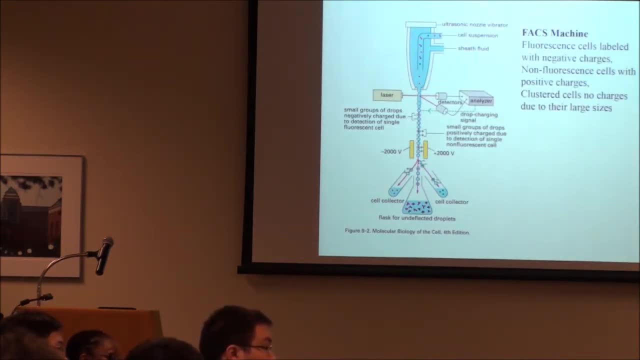 is it for cell count or is it for analysis afterwards, Because I'm considering it as far as like: is the charge sufficiently high where it can damage the cell, or is it? is the cell still viable afterwards? Of course, cell will survive. 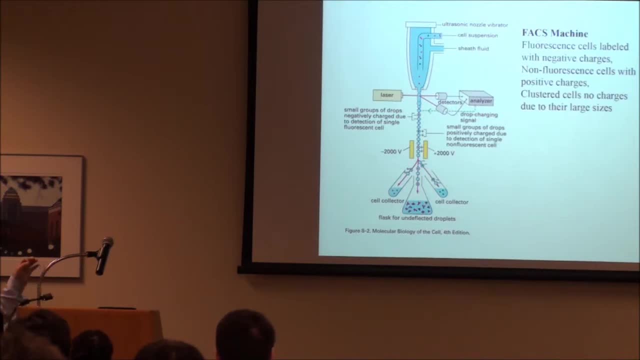 Yeah, That's the way you can, you know, identify and collect the specific type and continue to culture them. Yeah, There's another question. So, in terms of the detection of the other cells, like the laser is it? is it the steady-state spectrum that you're talking about? 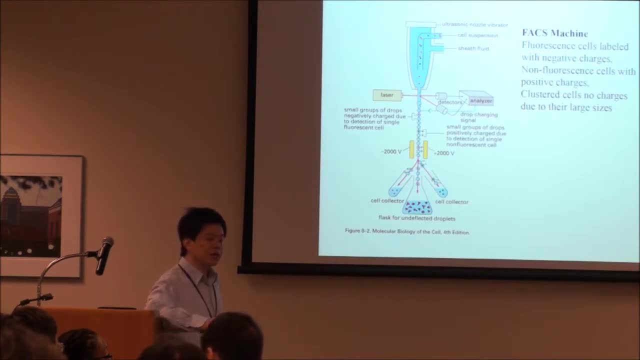 or is it the light-resolved signal based on the measurement there? Can you speak louder? Sorry, I didn't get So. when you attach a specific charge to one of the cells, Yes. What kind of signal are you detecting at the detection time? 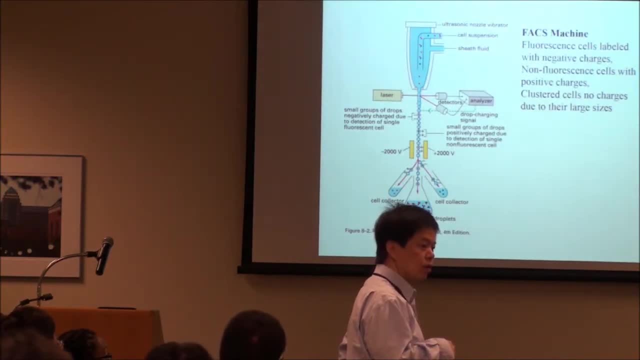 Is it like a steady-state spectrum or like a light-resolved signal? Oh, okay, Of course you can do. if you have a spectrometer you can detect spectrum, but most of the time it's just, you know a filter-based, you know camera. 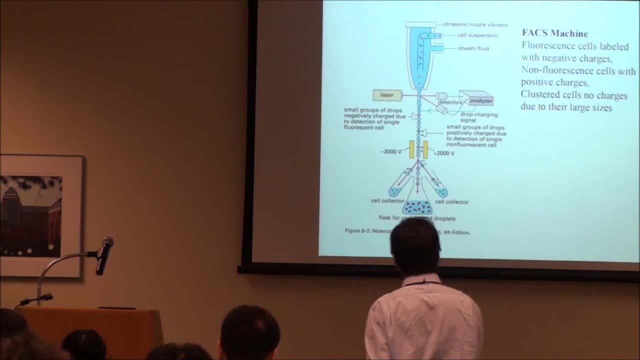 You can direct see the color. basically, How about the width of the channel, This, this channel? Yeah, This is about like 20, you know, or 50, you know, You can adjust, in fact, these snoozles. 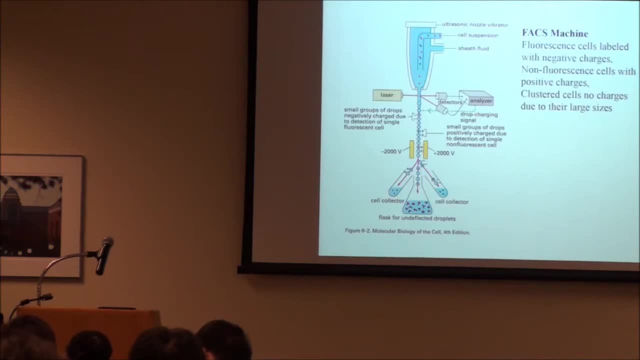 Adjust the size of these snoozles. So you must know the size of the cells as a priority. In general, you pretty much have pre-knowledge in terms of the cell size, yes, But you know the. Since you have this, you know adjustable size, right. 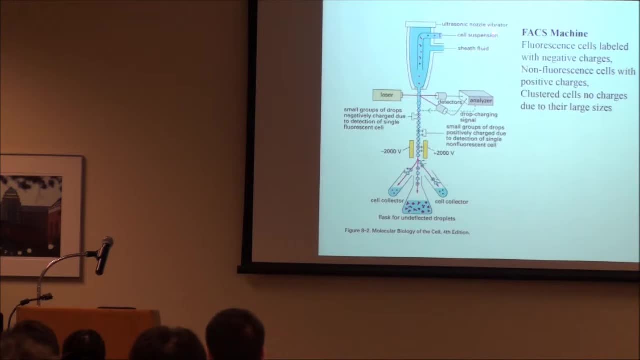 and you know some kind of- you know- knowledge of the cell population. in terms of the size, you can adjust nicely. you know Pretty much. you know. if it's micrometer range, no problem at all. Okay, Any more questions? 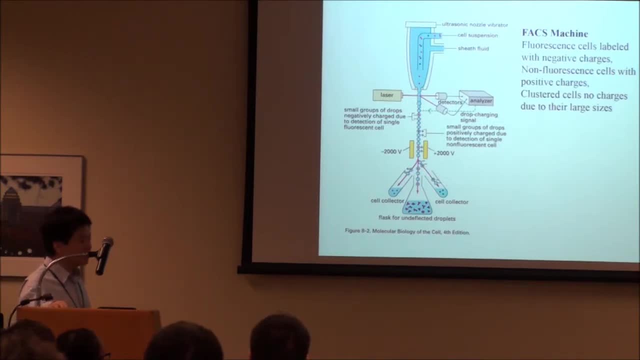 Why did you put the ultrasonic vibrator? What does the ultrasonic vibrator? Oh, basically, you know, just want to break, You know, because sometimes cells are sticky. Even you add the calcium, even you add these enzymes, right. 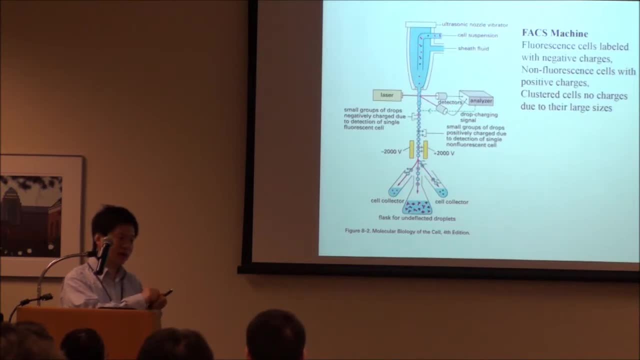 they are separated from each other, But sometimes, you know, membranes are still sticky, Okay, So you know, if you have some vibration to maintain their separation, Okay. Okay, All right, I'm glad So I can move on right. 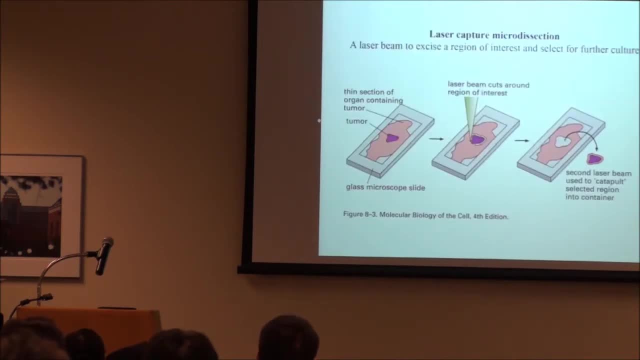 Yes, Okay. So another way is for some specific cell types, like Marina told you, right. so for some cancer cells, they, you know, grow together to form like a tumor type of thing, right? And in these cells, you know, basically, 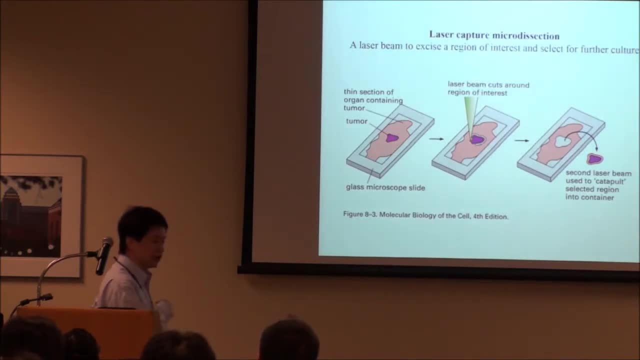 these are tissue sections. So for some specific tumor cells, if you are interested, study them. What kind of you know molecule signaling are going on in these cells? You want to study them right, And there's one way you can easily do that without you know. 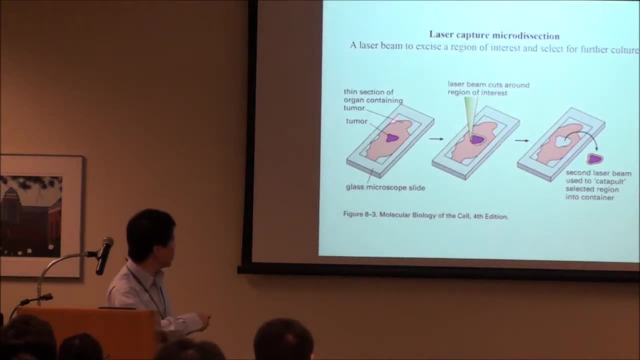 these complicated dots, you know, because majority of cells are not tumor cells. Only these specific confined regions contain tumor cells. So there's one way called laser capture, microdissection. Very simple: You can use a laser just to cut it. 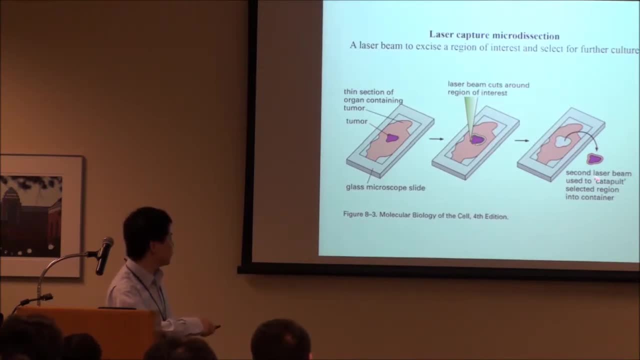 Okay, And using this laser again to flip over to another dish And then you can start to grow these purified tumor cells and then study their functions. Okay, So this is because you know, as you can imagine, if you use the traditional way. 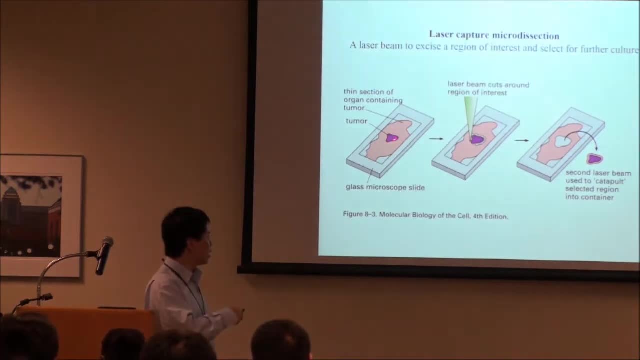 you mixed up like this is probably, you know, one percent of the cell over the whole tissue, right? So that's a waste of the antibody or other technologies, right, Because you're only collecting this very well confined cell population. 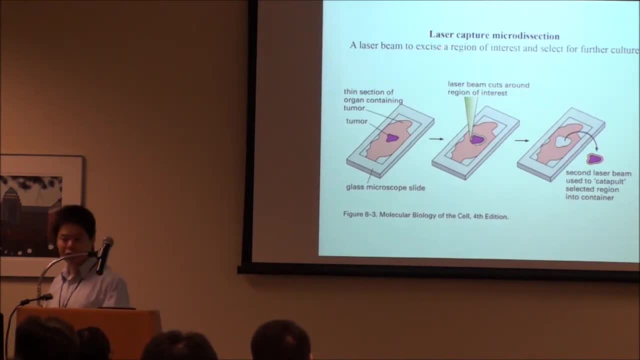 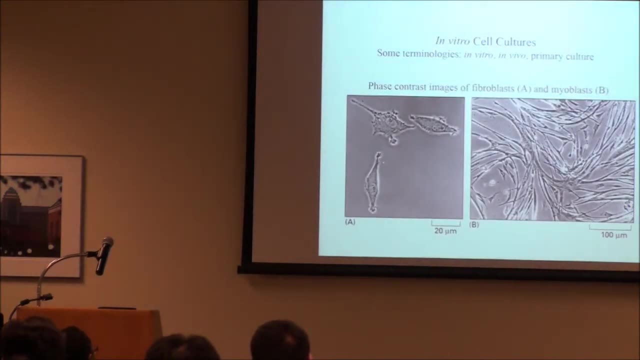 So laser capture dissection becomes more, you know, economic and efficient. Okay, So that's another way to purify cell populations. Okay, So, after you go through all these, you can easily collect the purified cell types. That's what you get in the laboratory most of the time, right? 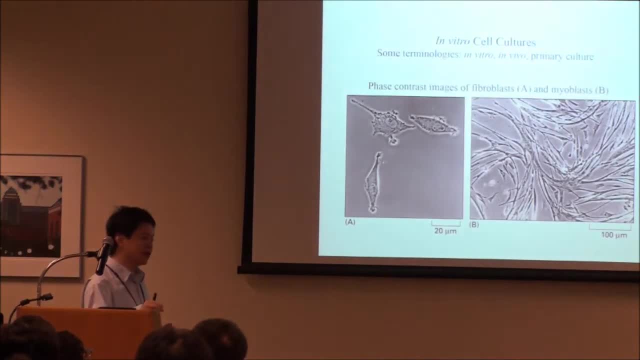 You are capturing all these specific cell types, Although you probably didn't really, you know, know how these cells are obtained. I'm telling you that's you know, like if you buy cell line from ATCC. that's how they did it. 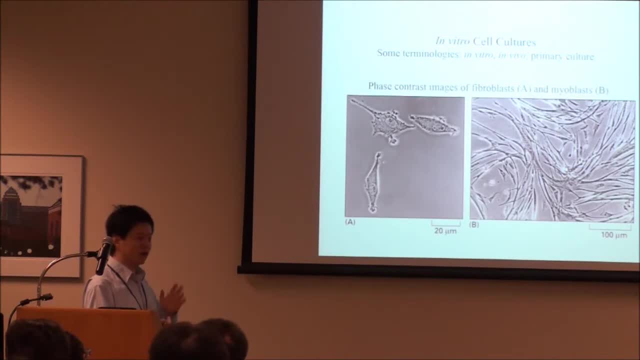 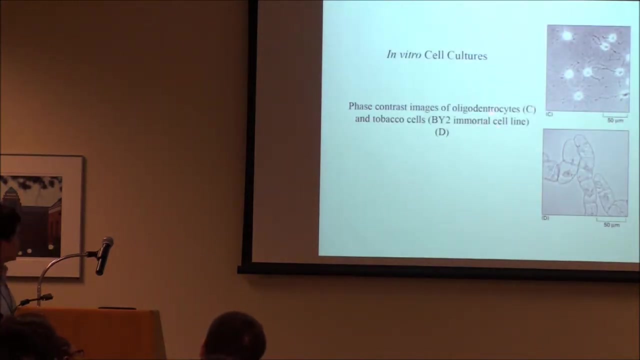 Okay, Through this fax machine sorting or laser dissection, you know. So when you capture it, you can see these different, purified, different types. This is fibroblast, This is the myoblast, They have very different phenotype, And this is oligodendrocytes and the tobacco cells. 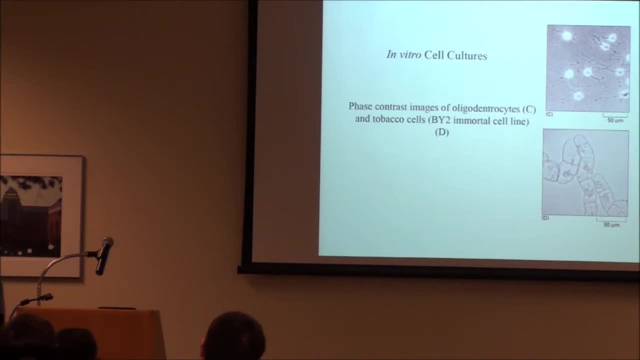 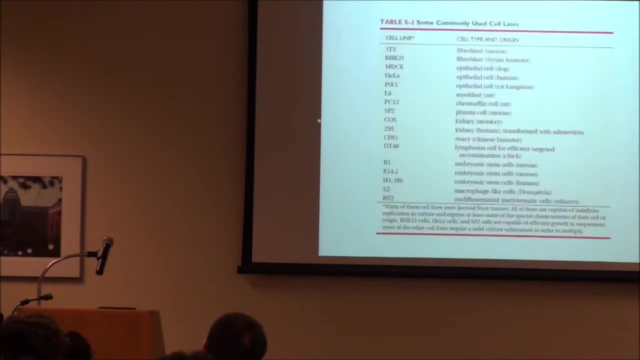 Okay, Now you have purified cell types, You can really, you know, harvest these cells, study the protein population in these cells, These different cell types. Okay, I think I just also listed the different, you know, cell types. 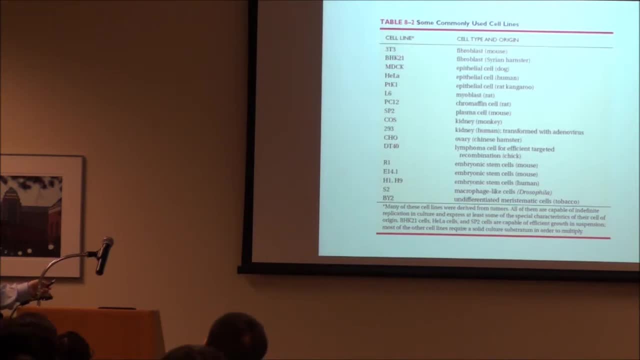 I think most of you probably are working with some of these cell types, such as 3T3 cells. basically these are fibroblasts. MDCK also are epithelial cells from dog, Healer cells, you know, epithelial cells from human. 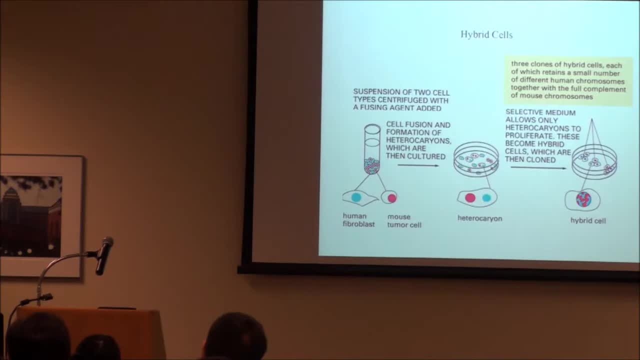 Okay, Besides these purified cell types, there are another cell type I want to introduce. is called hybridized cells. Okay, So it's a phenomenon that if you put two different cell types together, if you add specific chemicals, they can have some- you know, very interesting and weird phenomena happen. 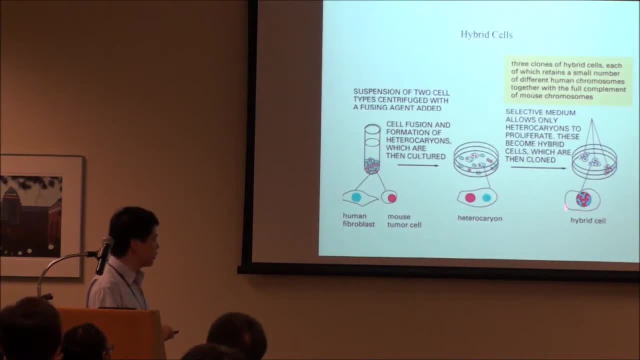 These two cells will be fused together and their chromosome eventually will be integrated to become so-called hybridized cells. Okay, You know, most of the time this will not happen, right? This is a very rare case. You have to use chemical to induce that. 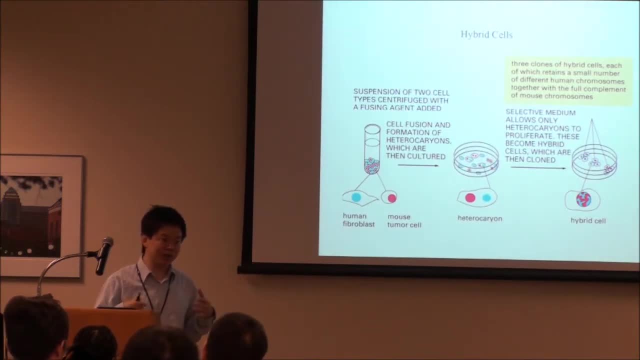 Otherwise we will be in trouble. right, Our body has different cell types. If they all merge together and become one cell type, we are doomed, right? So this is a specific and very rare occasion, but this exists, Okay. 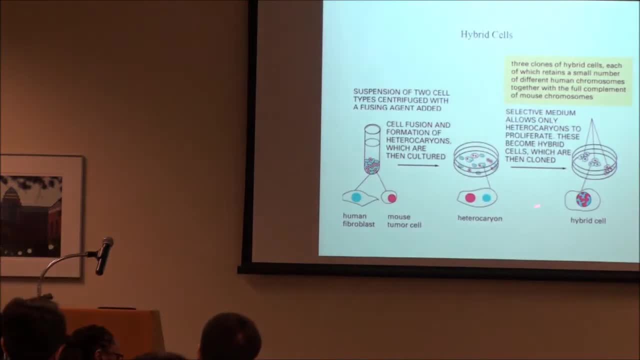 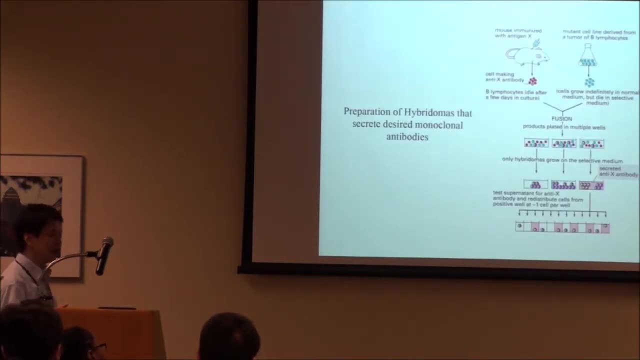 If you introduce specific chemical environment, they can do that. So this cell type has very unique feature and you can utilize to do some very interesting and cool stuff. One way is to basically produce antibody with very efficient or economical way. Okay, 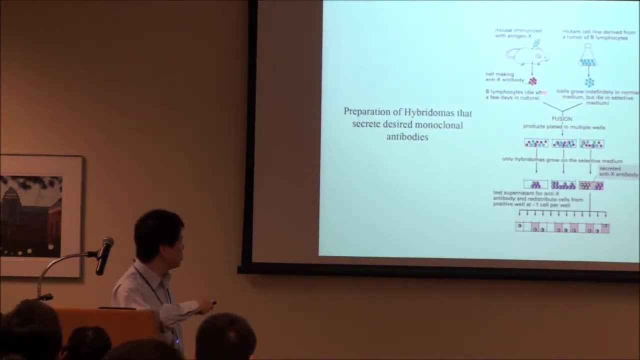 So if you want to produce antibody, that's typically what you have to do: You inject antigen right into a mouse and then the mouse will start to go through immunoresponse and produce antibody right. That's a typical, you know, antibody production process. But, for example, these cells which produce antibody, called B lymphocytes. they die quickly. Okay, Basically you have to collect antibody from these B lymphocytes, but the yield will be very low because they die quickly. You can collect with a very short time window. 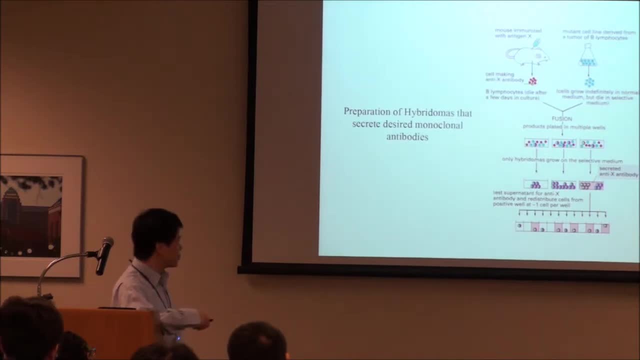 Okay, And the number is limited And people found out there are another cell type, which is tumor cell type or mutated cell type in this lymphocyte tumor. Okay, And these cells, they can grow forever, indefinitely, infinitely. Okay. 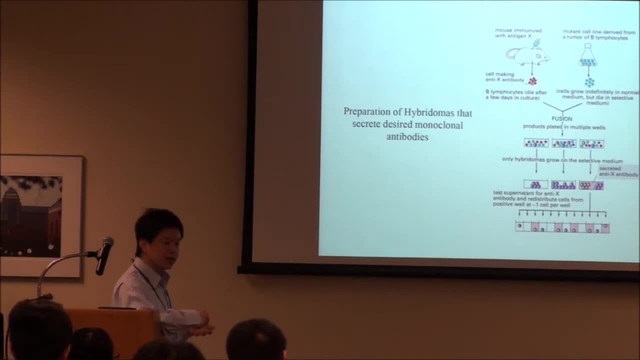 And if you can put these two cells together and induce and create hybrid cell, okay, and some of the cell, they will become hybrid cell and they can continuously produce antibody you want. Is it wonderful These cells will never die and they can keep producing antibody you want? 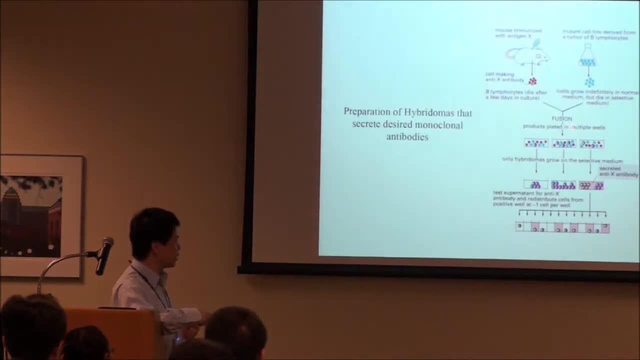 Okay, And this cell is very interesting. You can, you know, separate all these different cells and add some selection- you know medium- so that you can get a tube which contain only these hybrid cells. They will always grow, Okay. 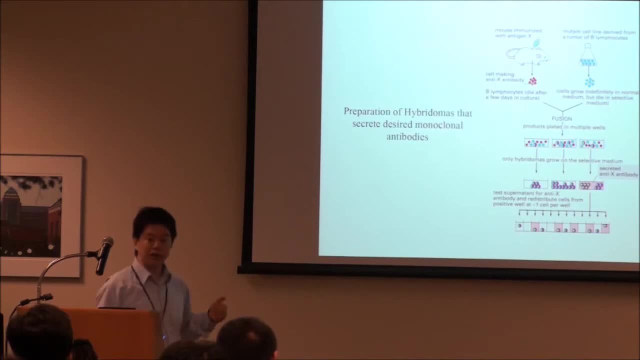 And they can always produce antibodies. Okay. So this is the way people are producing antibodies with much, much more efficient way- Okay, Utilizing hybrid cells, Please. What's the proportion of the cells that becomes hybrid cells? It's very low. 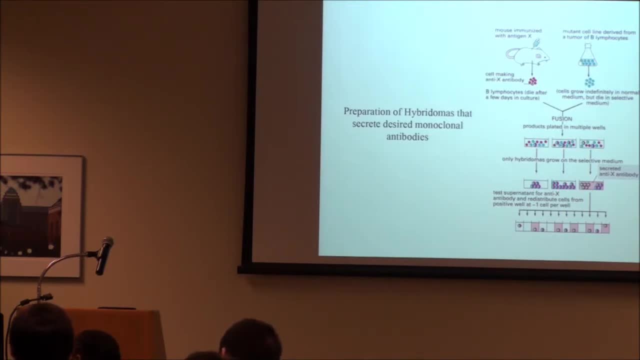 Probably 1% or below that. Okay, But it's still much more efficient than just having mice to produce Definitely, Because, after you know, using this selection medium to select these cells, you can culture them and grow them forever. So you can like a big tank, right. 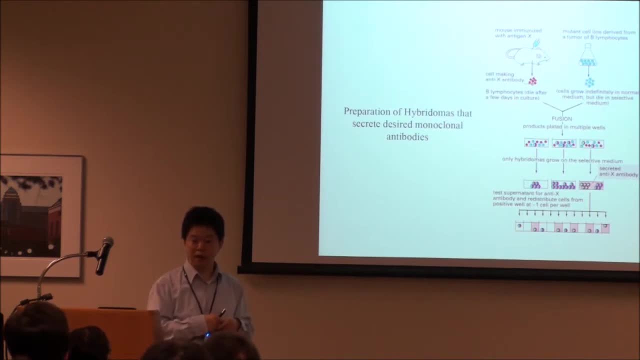 to grow them and they will continue to produce antibody. Okay, Instead you have to go through this mouse, kill the mouse and select, like microliter or the antibody you know every time, purify them. So that's really painful and low yield. 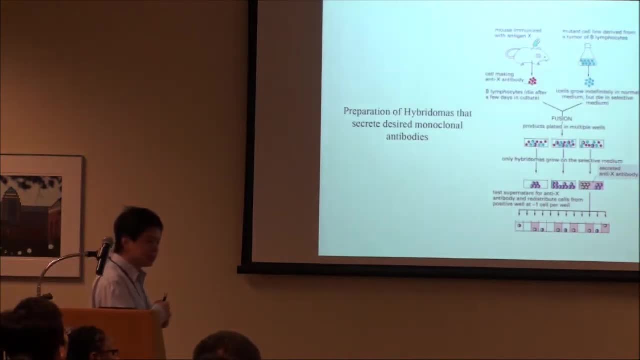 Okay, Is there any like clinical research to prove that those antibodies created by this way is not like, will not induce cancer? right, It's exactly identical antibody: The antibody you collect from the mouse versus antibody you collect through the in vitro. 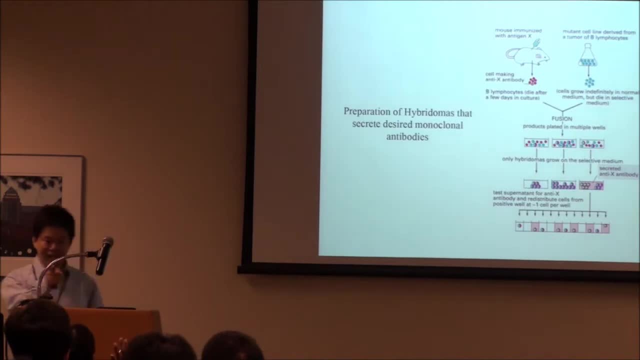 they are identical, Okay, Right, Okay, You first. then I have a confusion about the function of the antibody-antigen relationship. I misunderstood something somewhere, like when I thought that the antigen provided the binding site for the antibody. 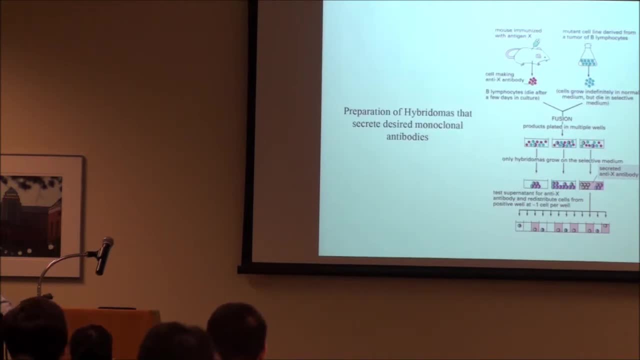 like, the epidermal growth factor receptor was the antigen and the anti-EGFR was the antibody, And so when we target the growth factor receptor, the anti-EGFR would bind to that site. I didn't know that antigens create antibodies too. 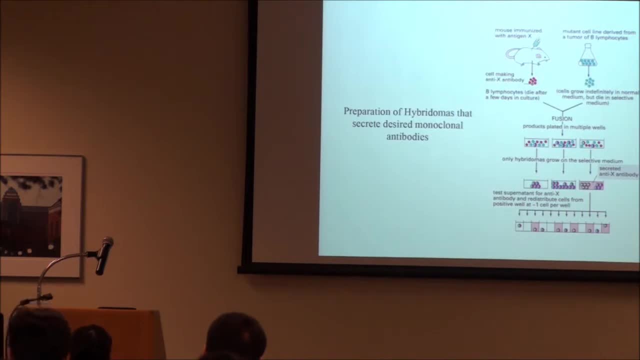 Is there a dual function or is there a misunderstanding on that? Okay, So this is, of course, not necessarily how to call this technology right, But basically, whenever we have antigen, go to the body right, this B lymphocyte will be the one. 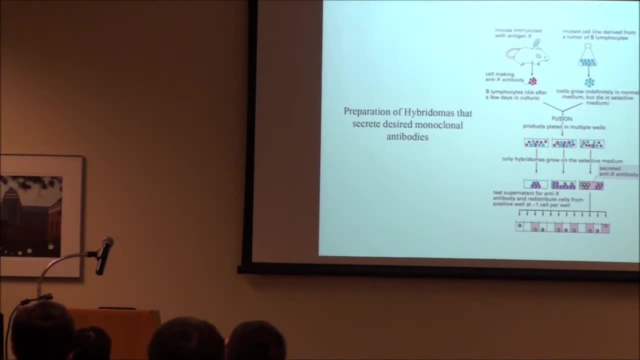 trying to recognize this antigen right. So they will start to synthesize antibody on the surface of this lymphocyte and recognize this antigen and grab it right. And this is how you harvest this lymphocyte: to collect antibody on the surface of this lymphocyte right. 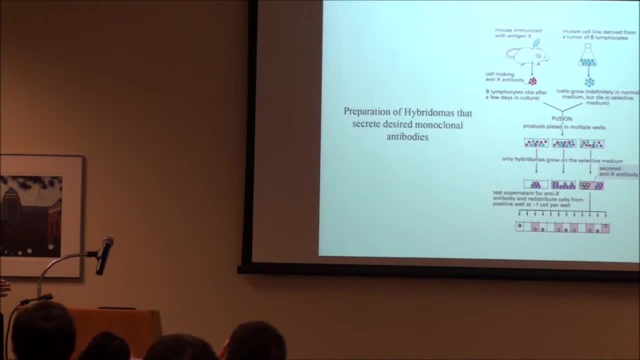 But because in animals you only have limited number and limited time to collect them, the yield is low. That's why you want to create that. Okay, Okay, Sure. Has there been any study where they've tried to maybe implant these hybrid cells? 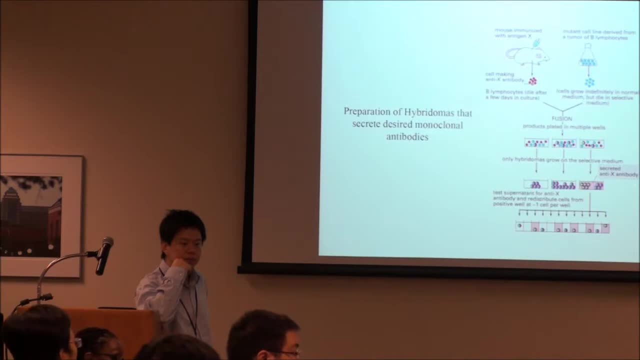 for sustained drug delivery, like anti-EGFR production inside cells inside the body, and are they viable inside the body or do they need, like some special media and stuff like that, where they would only grow in vitro or not? That's a very good question, I think. 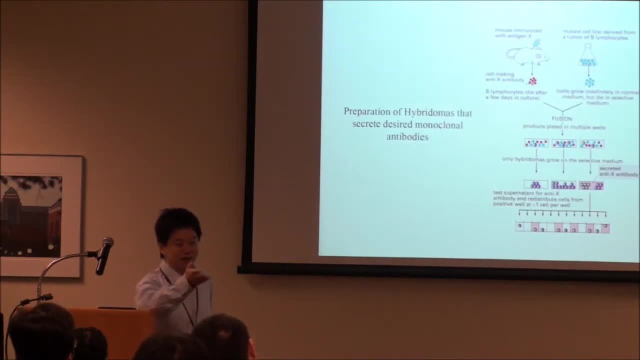 I don't know actually, So maybe people are thinking about it. That's a very creative way, you know, Although I suspect, though, these hybridized cells, because they are derived from tumor cells- right, they may be pretty, you know. 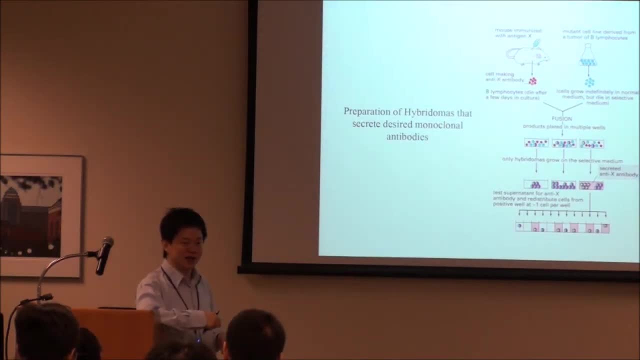 you know, cancerous If you embed into the body, may not do you know, good things for the body. So I'm not sure. but I don't know whether people are doing that, But that's a very creative way to utilize this technology. 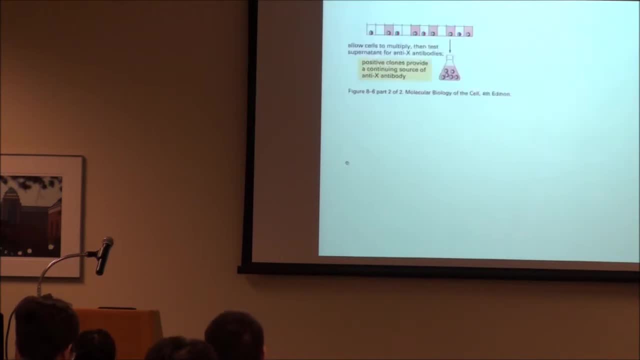 Okay, All right. So we'll move on, And this is okay, just to show you. you know that's. you know modernized technology. you know to produce large-scale antibody. you know conveniently, All right. 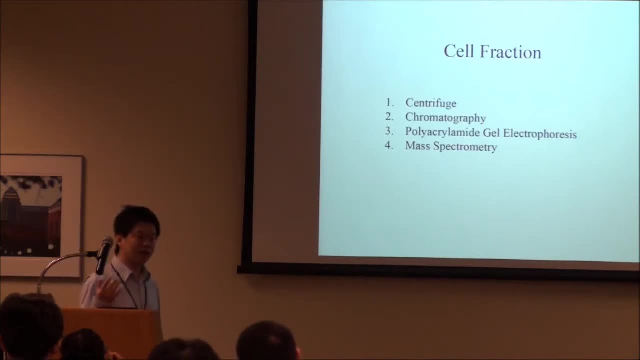 So now we know how to purify cell types, how to create these weird or interesting cell types. How do we study their functions right? How do we study the proteins, molecules in these cells, in these purified cell types? Okay, And this: 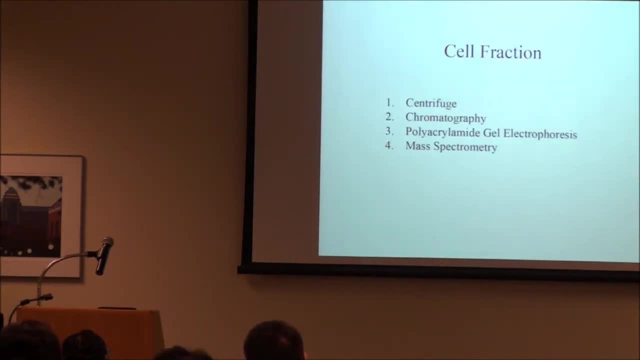 I'm going to introduce a couple of technologies people utilize nowadays. right to study them. One is the so-called centrifuge, Because in the cell body, you can imagine, although the cell is purified, right, but there are probably millions of different kinds of molecules. 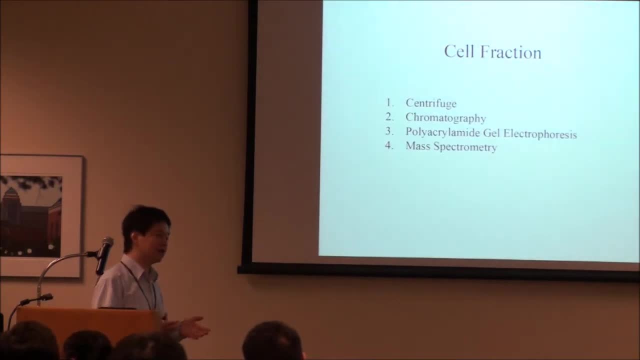 proteins in these cells, right. How again, do you separate them and collect the specific type of molecules, type of proteins to study their functions? Okay, So we have centrifuge chromatography and polyacrylamide gel electrophoresis. 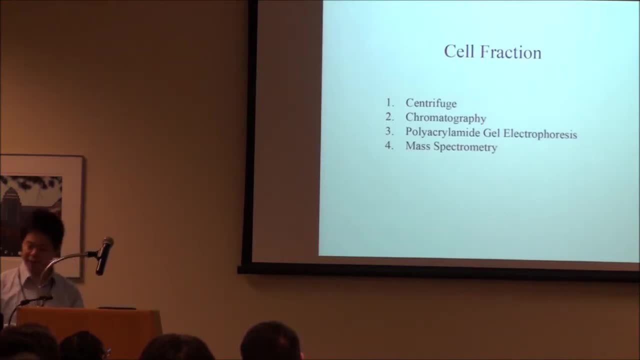 and mass spectrum will be the one we are going to introduce. Okay, First, the centrifuge. Okay, this is a typical machine. so-called the ultracentrifuge can generate really, you know, high speed. This actually if you are working in the lab. 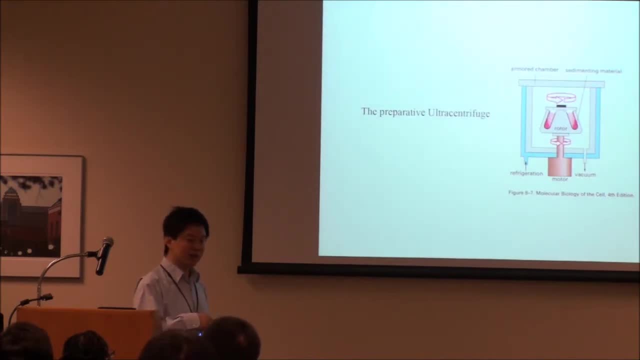 you have to be very careful because we heard some horrible stories Because speed is so fast. you know, if you are not correct the balance, this rotor, it can go off and generate huge force and this whole thing will just fly up. 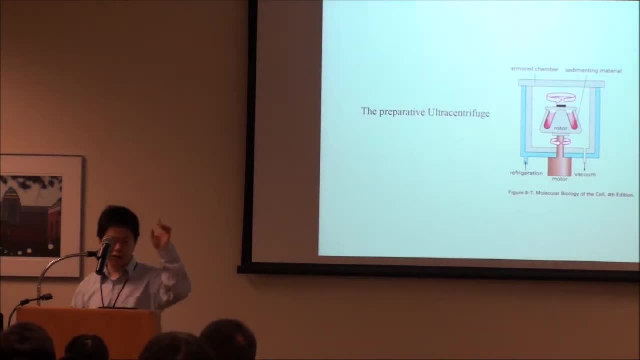 And when I was in UCSD as a graduate student- you know the floor upstairs- I heard some horrible story. This student didn't carefully balance the tubes and the rotor just fly up and it just damages the ceiling. Okay, 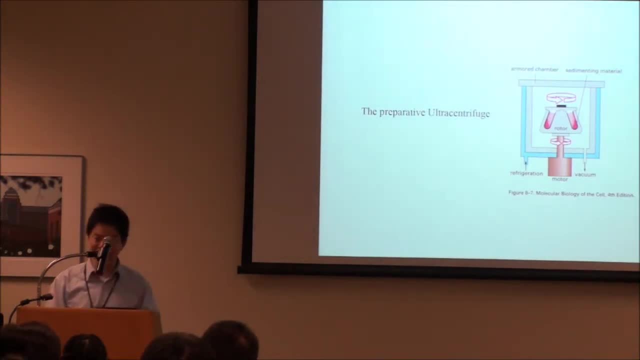 You can imagine how much force it is Okay. So this the principle is: after you collect these cells, you destroy the cells using detergent right to break apart the cell and collect all the proteins, and you use high speed to separate. 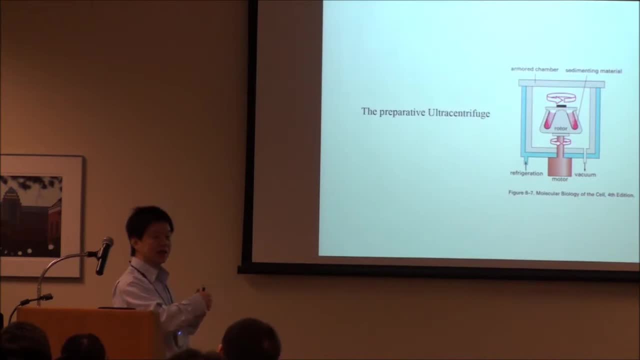 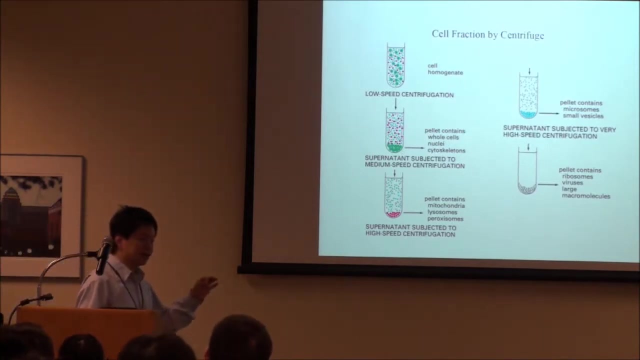 different population of cells, based on their size, their density, okay, And the separate, the proteins, based on their size and the density, Okay. So this is basically the different speed to collect different kind of, you know, intracellular, you know. 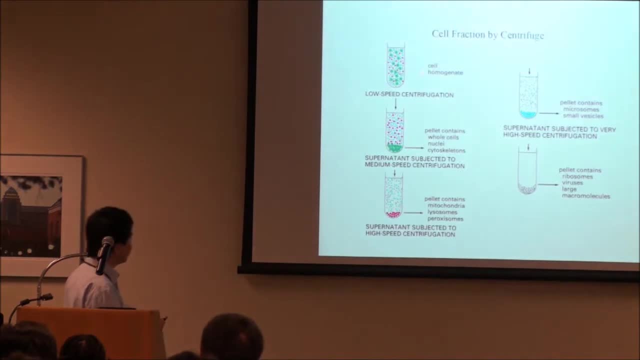 organelles or proteins. Okay. So, for example, if you use a very low speed centrifuge, firstly, of course, kill the cells right using detergent to break the membrane, collect all the proteins and load into the tube. 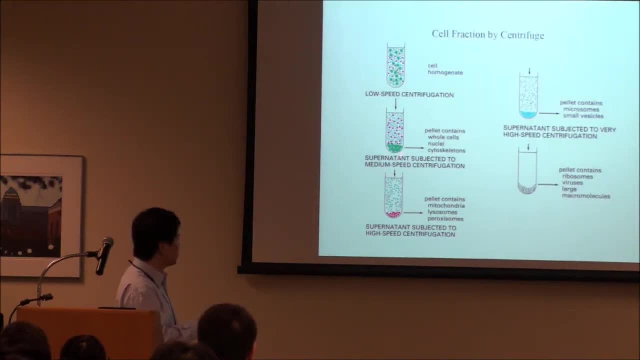 and centrifuge If you use a low speed. the bottom part, which is the pellet, mainly contain a lot of organelles like the Golgi complex right endoplasmic reticulum and some acting filaments. 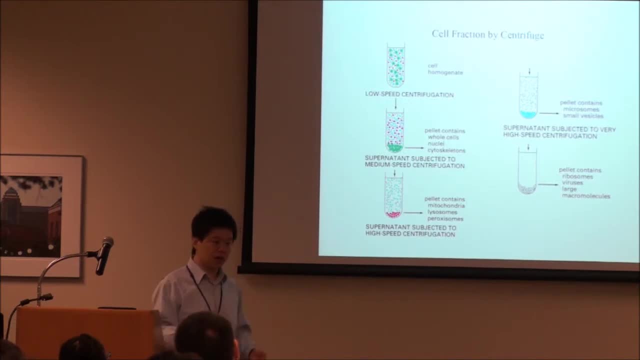 okay, cytoskeleton nucleus, all will be piled down. Okay, So this is the first layer. you can collect certain part of cell. Okay, Now you take off the supernatant, which will contain some small organelles like lactosone. 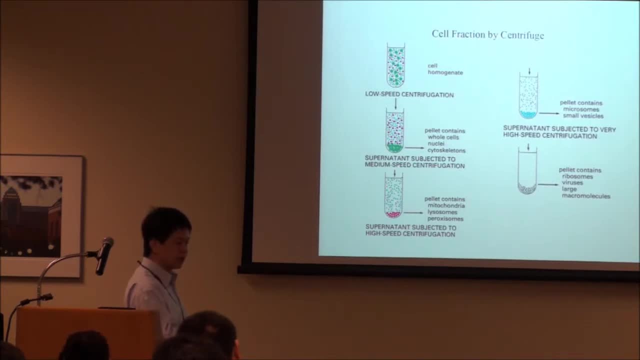 all these and increase speed. Okay, You collect another layer which contain like mitochondria, lactosone, pyroxone. Okay, And in this supernatant you can collect this supernatant again and apply a further enhanced speed. 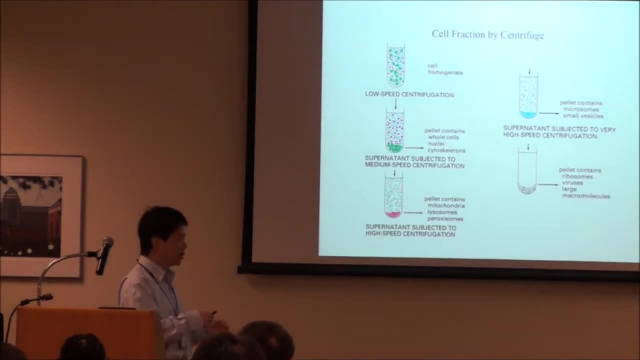 to centrifuge. Okay, Now what you got is macrosomes and small vesicles. Okay, And you collect supernatant again. apply to so-called another tube and apply ultra-centrifuge speed, really high speed. Now you will collect. 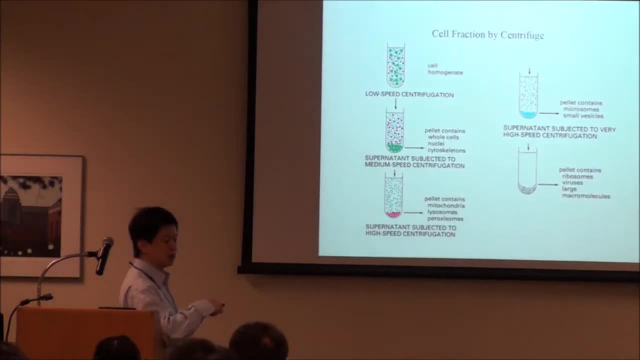 this supernatant again apply to so-called another tube. now you will collect this so-called macromolecules, ribosomes and this supernatant. What will be left in the supernatant in general after all these steps of centrifuge? 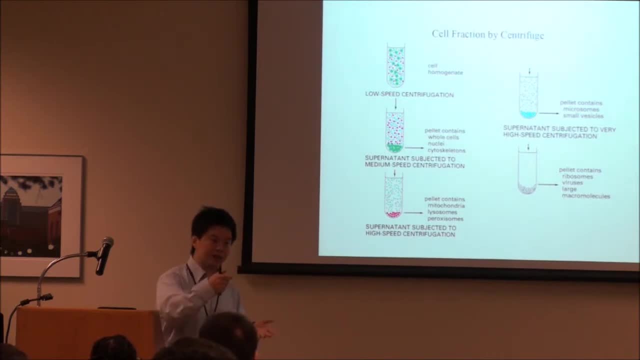 Question: Cytoplasm, Cytoplasm and some molecules, right Separated molecules in the cytoplasm. Okay, And then if you collect this supernatant you can really study, you know, the relatively small molecules or molecule complex. 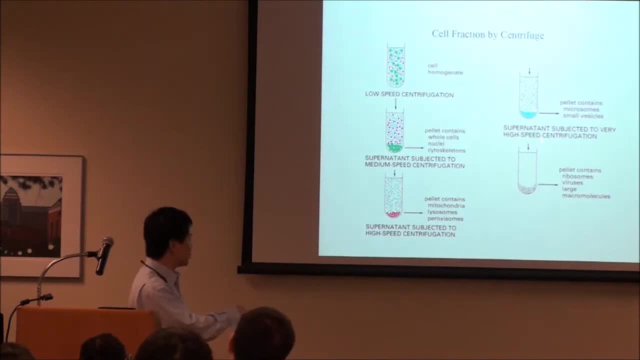 Okay, Right, The majority, the big ones, have been separated, purified from different steps of centrifuge speeds. Is it clear, so far, Okay. Is this manual process and also, how long does it take to get to the Get to this step? 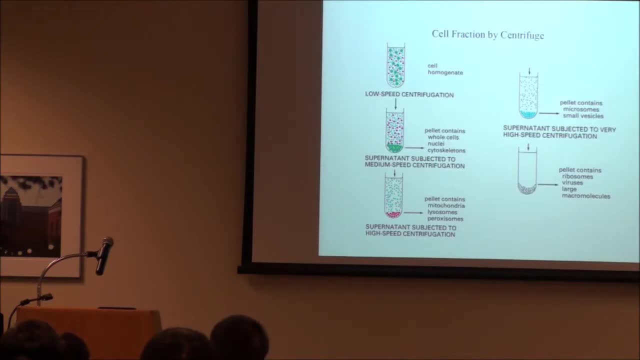 right. Probably, you know, one day or maybe two days, Like this ultra-centrifuge you usually have to do like overnight. Yeah, because you know the size is so small, so going down is very, very you know. 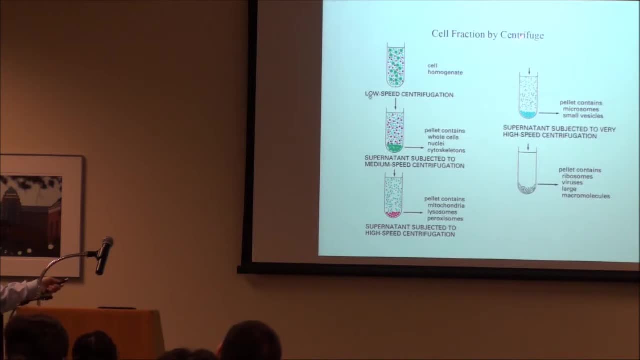 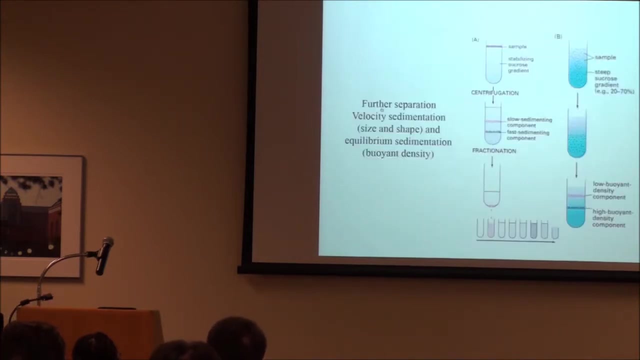 slow, Okay, But anyway, going through these different speed of centrifuge you pretty much separate the cell body complex right Into different populations, right, Large complex versus small molecules. Okay, So these are the centrifuge Another way. 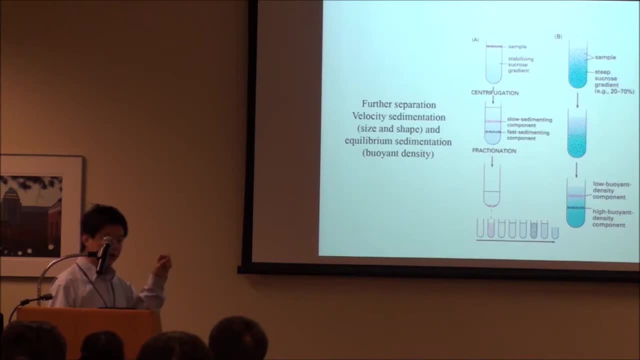 you can also utilize this: after you centrifuge different sections of the cell body, you can also use so-called- you know- sedimentation, either velocity or equilibrium sedimentation, For example, if you apply a collected pellet. okay, on top of this. 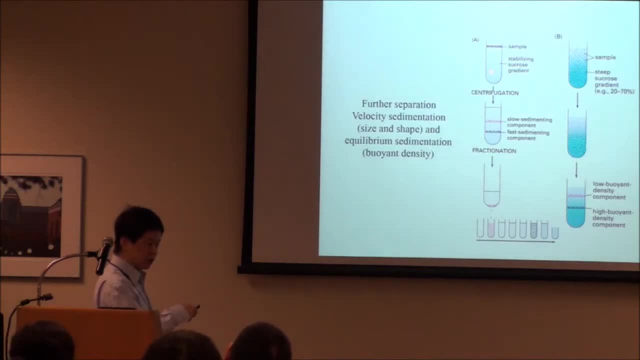 sucrose gradient solution. this is a relatively shallow you know sucrose gradient. you can apply centrifuge and then you can separate these different you know molecules. or you can create relatively sharper gradient of the sucrose and apply centrifuge and you can separate. 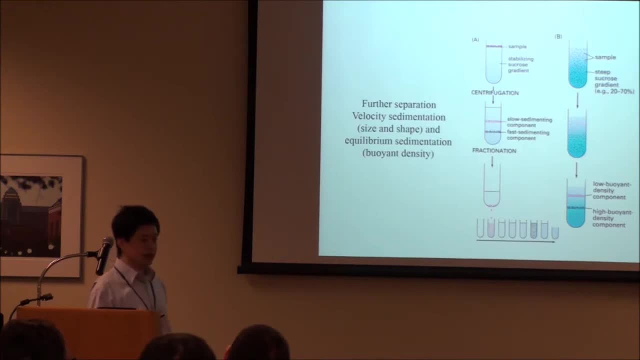 these molecules different molecules based on their buoyant density. Okay, So in this tube you can already see. you know different molecule will be located at different position, right, If you punch a hole on the bottom and collect different fractions. 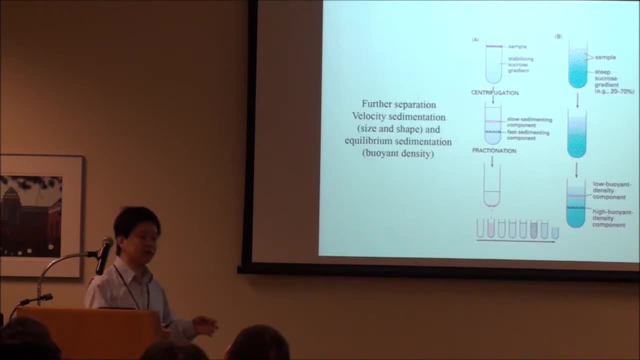 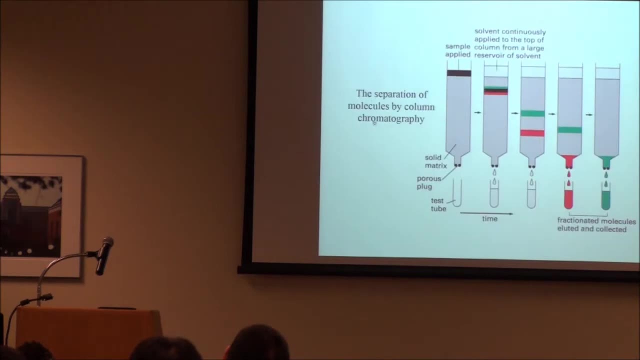 you will know, for example, this group of the different molecules in this tube. okay, So you separate different population of molecules by this way. Another way: you don't use sucrose gradient, you use so-called column. So what's inside? 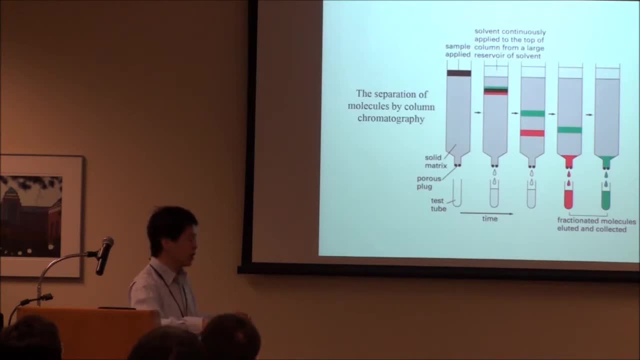 this column, These are basically beads, okay, And you apply this mixture of the molecules on top and let them go through using gravity, through these beads column- okay, And different molecules during this process, different size or shape- okay, And because they are, 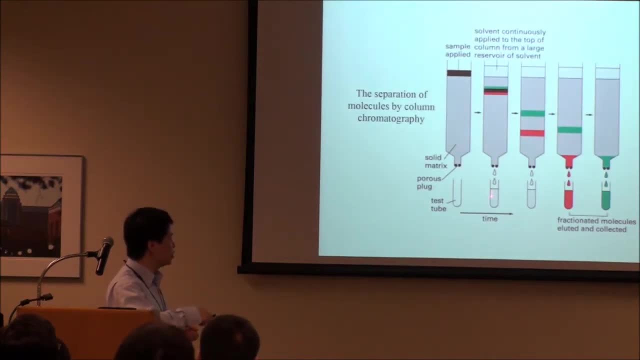 separated. if you collect, you know this solution flow through at a different time, you can collect different population of molecules. Is it clear? This is so-called you know chromatography. okay, And this chromatography can be designed using different ways. 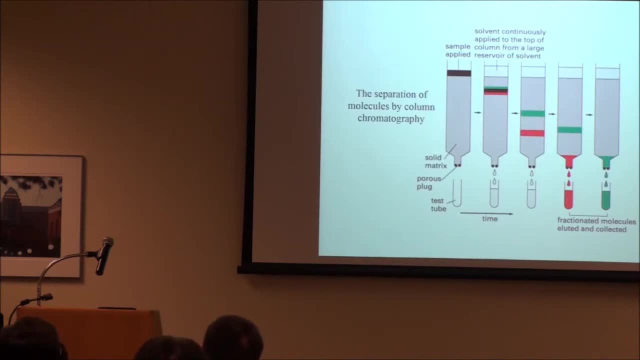 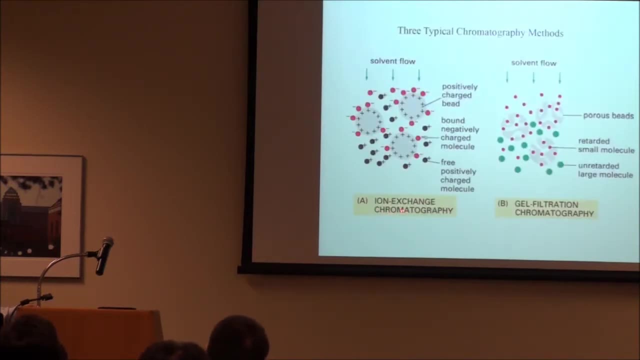 Basically, you can modify the beads so that you can separate different type of the molecules. okay, You can other using so-called un-exchange chromatography. Basically, if it's un-exchange chromatography, that means the beads in this column are charged. 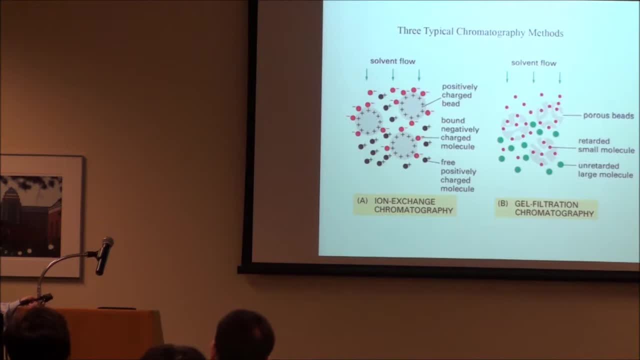 okay. For example, if they are with positive charge, you can imagine the molecules with negative charge will be relatively sticky to the beads right. Right. Molecules with positive charge will be flowing through faster, Is it clear? So the molecule? 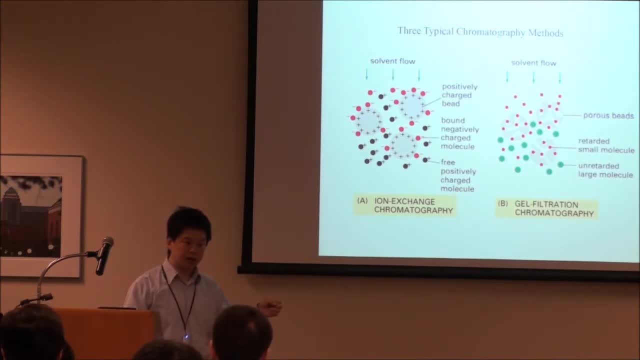 with positive charge will be collected earlier, right, If they go through, and the molecule with negative charge will be collected at the late stage because they have become stickier to the beads. okay, That's called un-exchange chromatography And second type. 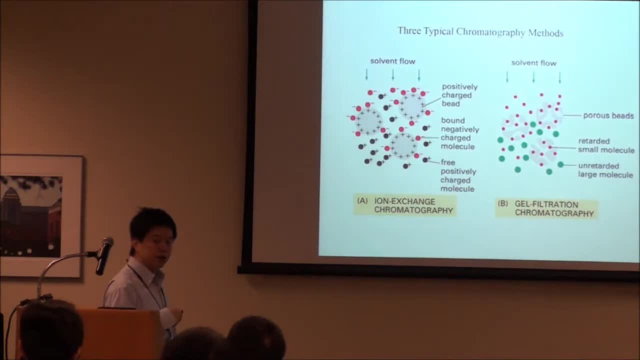 is called gel filtration chromatography, So for gel filtration chromatography. basically the beads are like sort of like broken. you know cavities on the surface of beads. So small size of molecule will be trapped. okay, They will not. 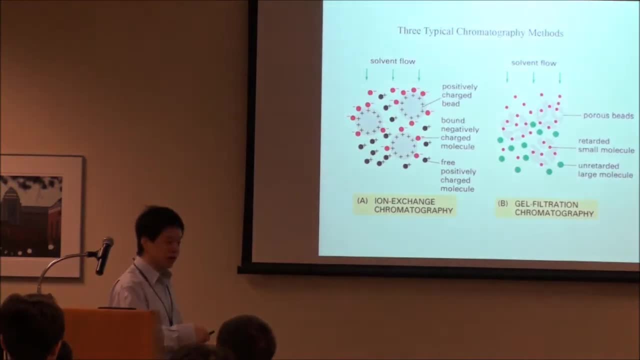 flow through as fast as this big molecule, because this big molecule cannot be trapped in these cavities, So they will be collected faster, okay. Small molecule will be trapped and eluted later. okay, So by this gel filtration chromatography. 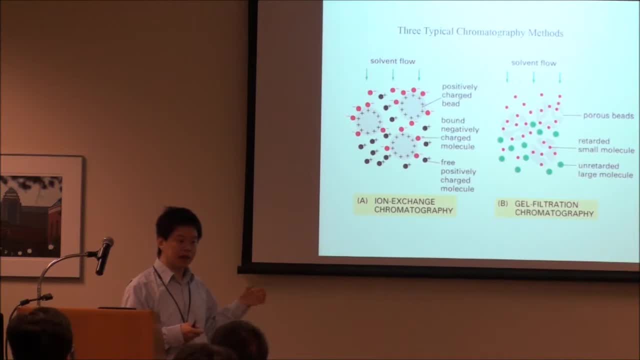 you can separate molecules by size, right: Large size molecule collected first. small size, collected later. Question: What is the size of these beads? Good question, I don't know. actually, Obviously they have to be larger than the molecules. 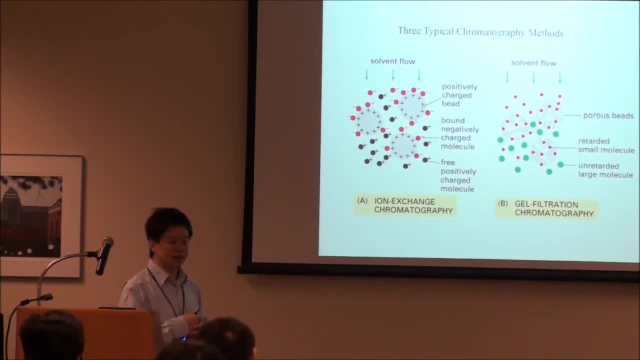 Yes, but in general it should be like nanometer 20, 50 nanometers- That's a little bit larger than the molecules, but close to the size of molecules, okay, And but these are not, you know, as you can imagine. 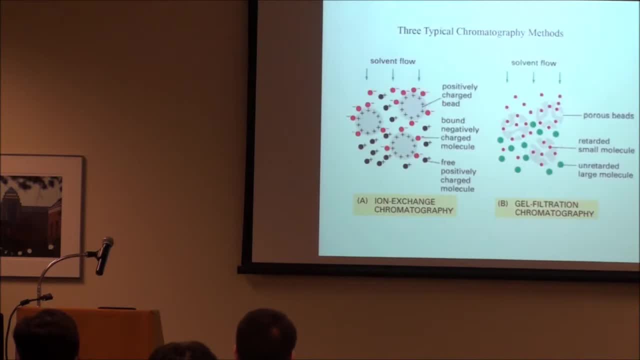 right, Many molecules. let me see many molecules, although here we only show different, like two kinds of molecules, but many molecules. they have similar size or they have similar charge. So these are not very precise separation right. 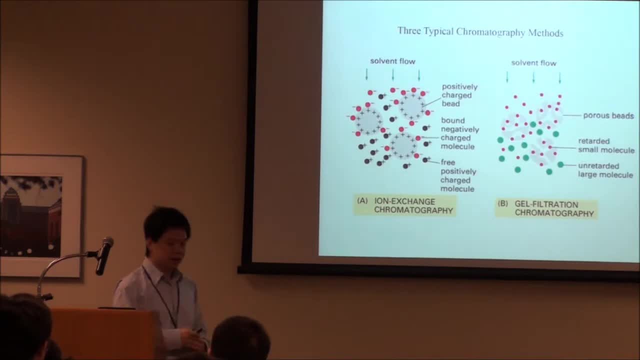 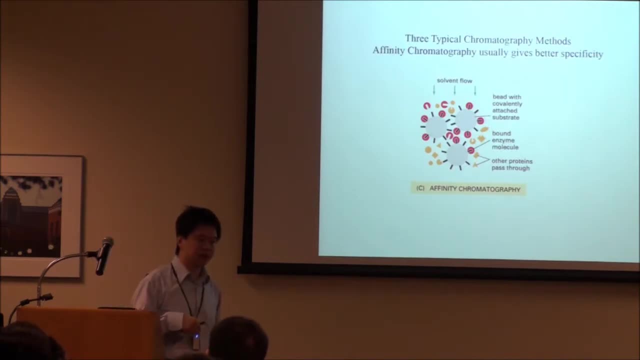 Molecules with similar size will be, you know, trapped in these cavities, right? Most accurate one is antibody-based and this is called affinity chromatography. okay, So if you want to specifically separate one type of molecule, you are interested. 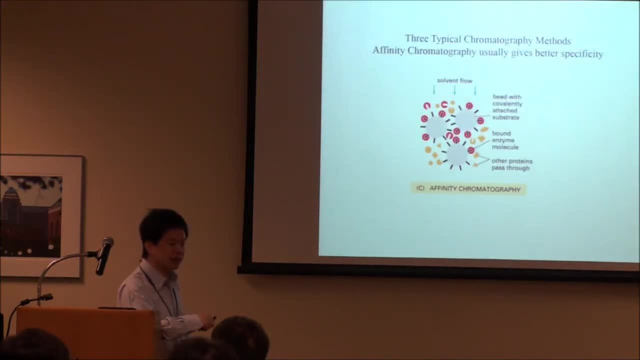 you can code the beads with specific antibody recognizing the protein you are interested. okay, If you go through this column, then the protein you are interested will be trapped on the beads right, Because antibody recognize the protein you are interested. All the other protein. 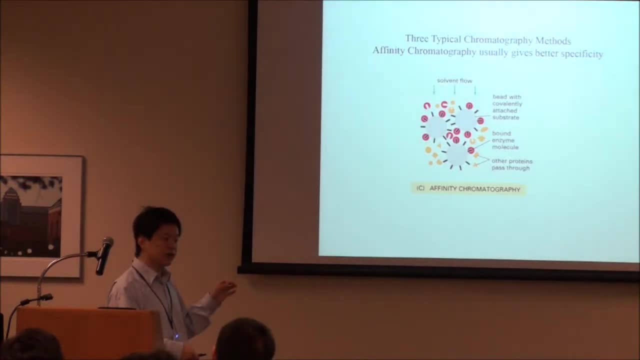 will go through easily, right? So therefore you can collect the protein with high precision using affinity chromatography. okay, But in reality in the cell because so dirty. why we call dirty? Because there are so many different kinds of proteins. 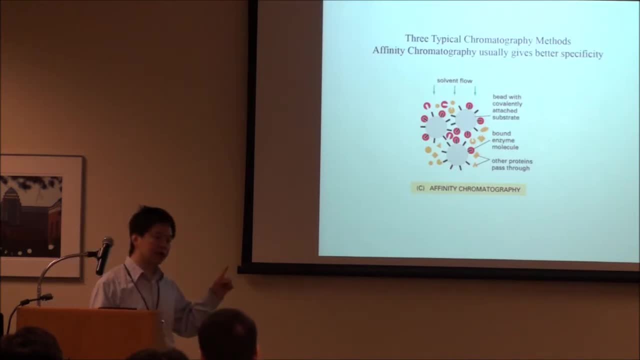 all messed up together, right? Only with one kind of chromatography is not enough to give you the purity you want. Usually, people always combine them together. okay, You go through multiple paths or different types of columns to get the purity you want. 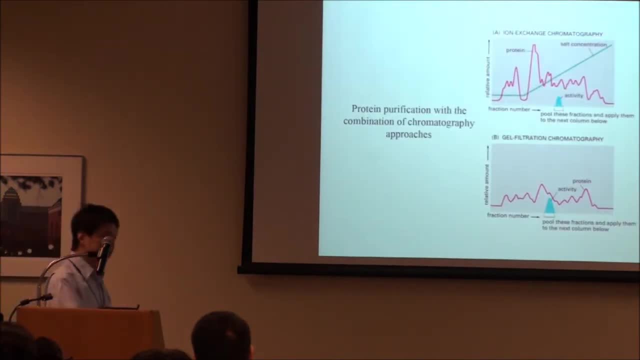 So this is a typical way when you are in the lab if you want to purify a specific protein. how many people already have done that kind of work- Purify protein from cells, okay, Okay, so you must be good already. 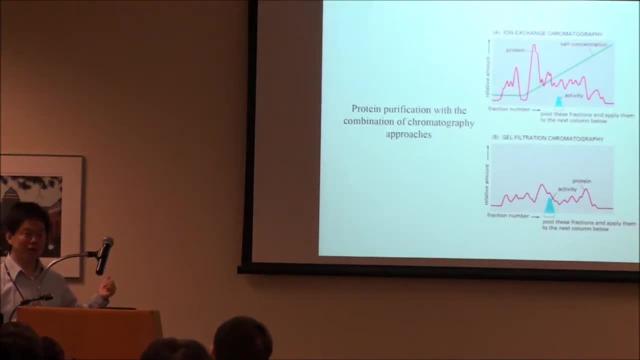 So these are very- you know- basic principles for you. if you want to start some new experiment, you want to purify some new proteins, that's how you do it. okay, First, as we already know, right, You take down. 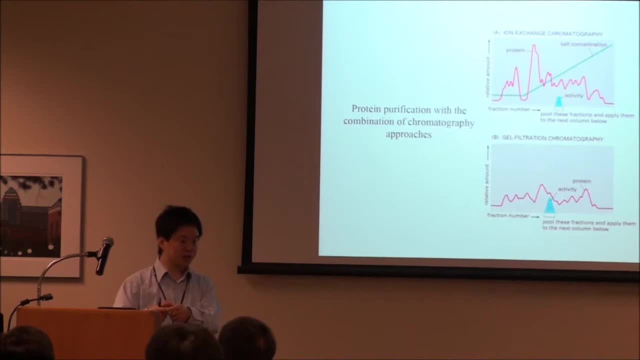 you centrifuge them, right. You already collect different type of the population of the molecules or complex and then you load into the chromatography columns. okay, Usually you will set up three type of columns side by side. okay, The first. usually you go. 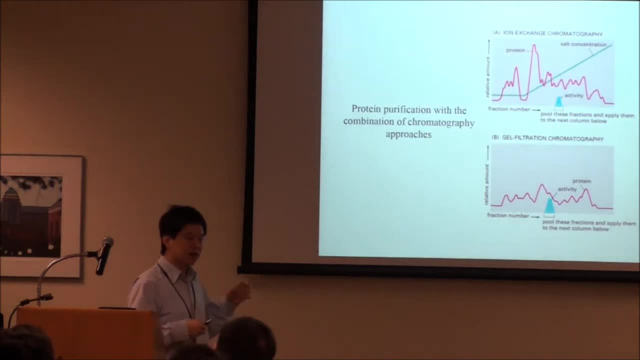 is ion exchange chromatography, okay, The first collect the population of molecule you are interested, based on their charts, okay, So here is the chart. You see the protein go through, okay, And this is the green line represent the concentration of the. 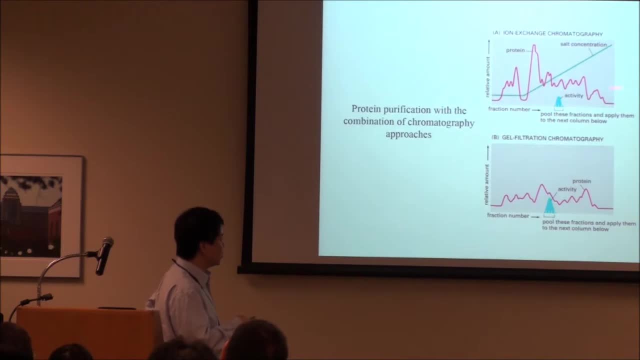 solution you add to the column. okay, And when you add or increase the like salt concentration, more and more protein will be eluted. okay, And this pink, you know profile represent the concentration of different type of the proteins. okay. 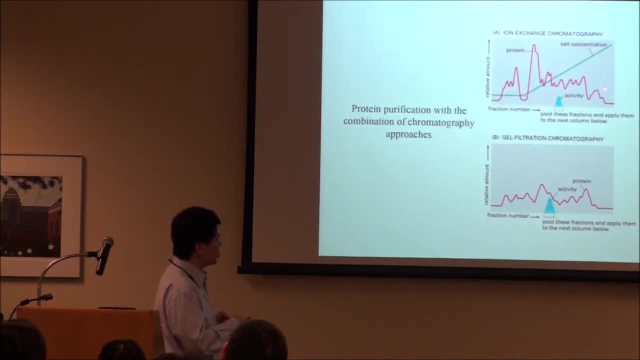 So when you add more and more salt, and eventually all the protein will be eluted. and this is the population of protein. you are interested and this you know. this section of the tube you will collect. okay, So the first purification will be happening. 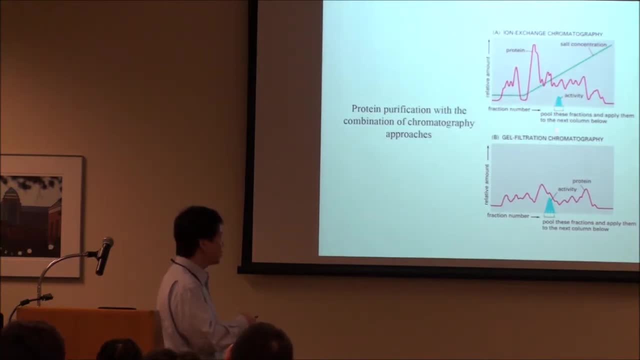 there, Your protein will be part of this population. okay, After you collect this purified, relatively purified protein, you load into a gel filtration chromatography. okay, Run another column, your protein right, The size relatively right, And you can. 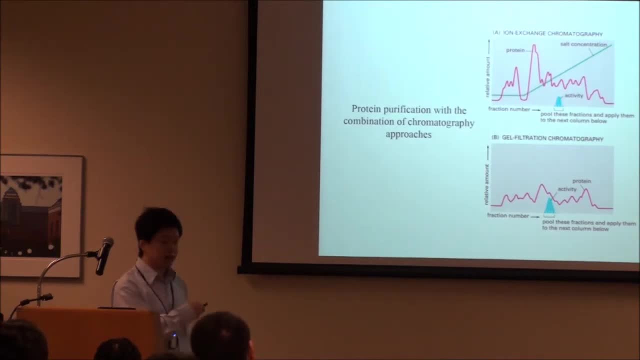 collect this population. similar kind of concept, but based on the size. okay, This is based on charge. After you collect this, this is still not pure. usually, okay, Usually they still contain multiple kinds of proteins all mixed together with similar kind of charge. 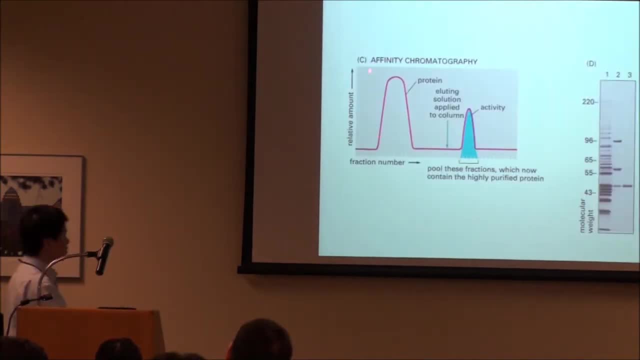 similar kind of size. okay, Now you run into the last chromatography, the beads with antibodies that you are interested, right, And then you elute all the protein which are not bound to the antibody. After you elute all these, then you add: 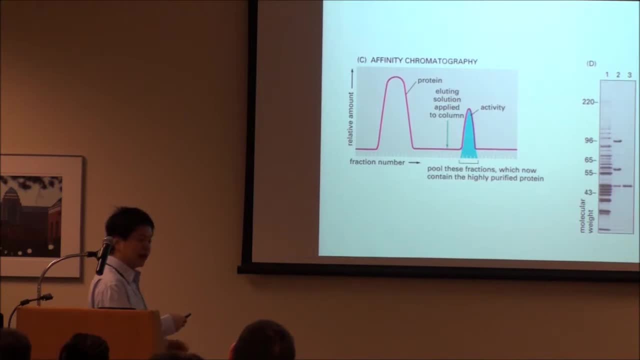 really strong elution buffer and the antibody and the protein you are interested will be decoupled right. The protein will be flowed through and you collect this population. okay, After these three type of columns you will get relatively pure protein, if you are interested. 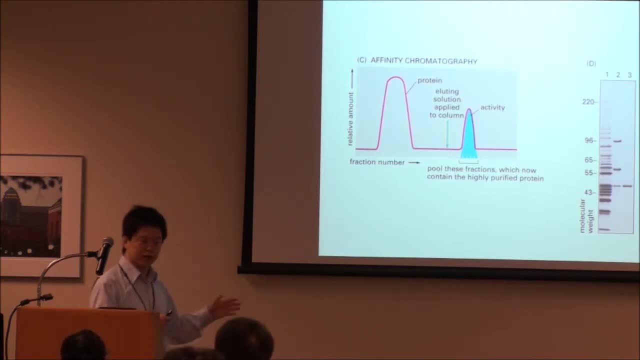 Is it clear so far? Okay, If you go to lab, you want to purify protein. that's usually the way you will design your experiments. okay, And after this purification, usually you will. if you run a gel, you can pretty much see. 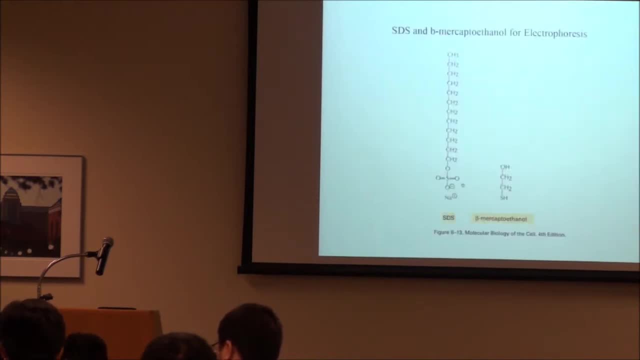 there are only two, three types, Still not completely pure, yet okay, But these are generally depend on enough protein. Whenever you are using- you know chromatography- you usually need to enough. you need to collect enough protein. If the protein 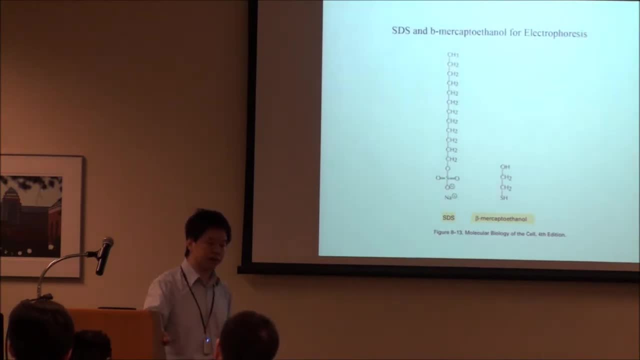 amount is relatively small, then you are not qualified to do chromatography, because chromatography, you know you waste a lot of protein during the purification process. okay, If amount of protein is very, very tiny, then you need to consider other technologies, so-called 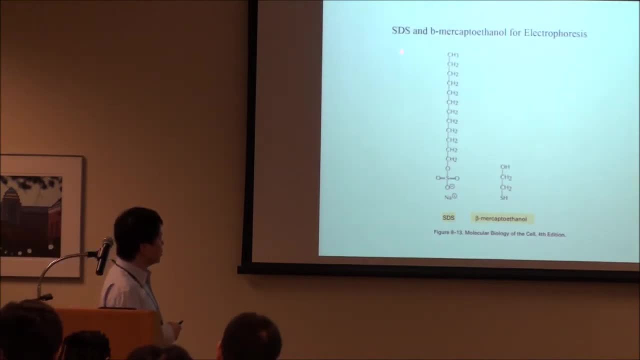 the principle how this SDS or beta, mycapital, ethanol based electrophoresis is designed. Basically. these are the two you know chemicals. They can bind to molecules and separate all the molecules to become relatively monomers. okay, If the protein amount is not. 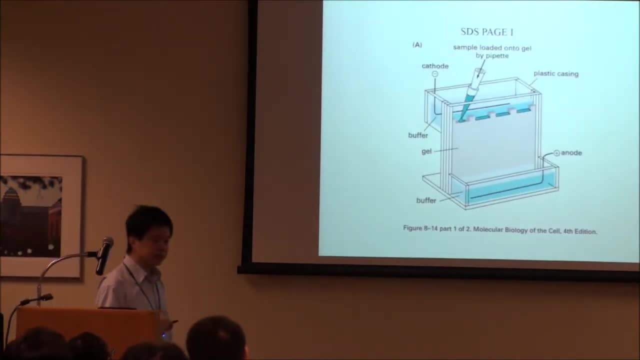 big. you use these so-called SDS PAGE gel. okay, All the proteins, because protein amount is not enough. right? You cannot allow the luxury to run go through the column chromatography, Then you directly run into a gel, okay. 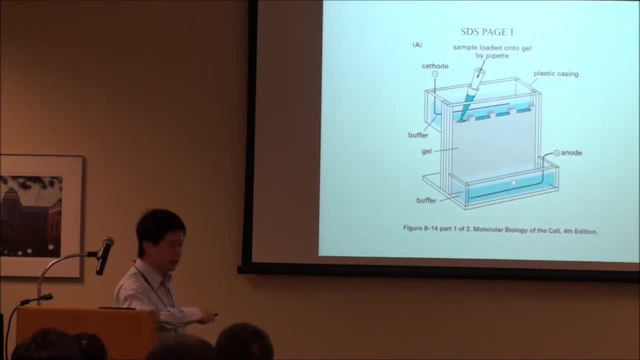 Collect all the proteins. and these gel are connecting two reservoirs: the upper reservoir and lower reservoir. These are serving as buffers and these two reservoirs are connecting to different, you know, electrode field. Okay, Top one will be negative charge and bottom. 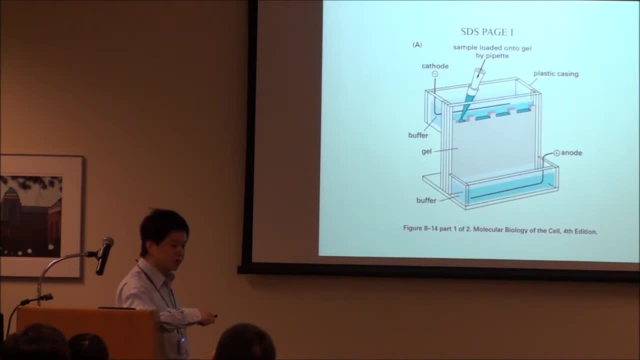 will be positive charge okay. And if you load the protein on these different wells, if you start the electrode field right, the protein will start to run through these gels right. Which direction will they go? They will go down. 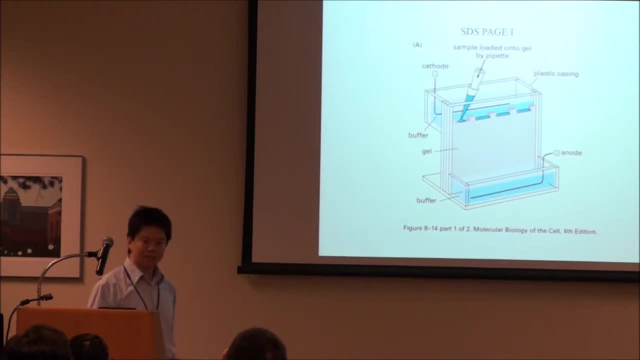 right, Why they will go down Very good. I think I didn't spend enough time here. So you see, these chemicals are really mixed with the proteins, right Molecules. So these chemicals will wrap up the molecule right, And you know. 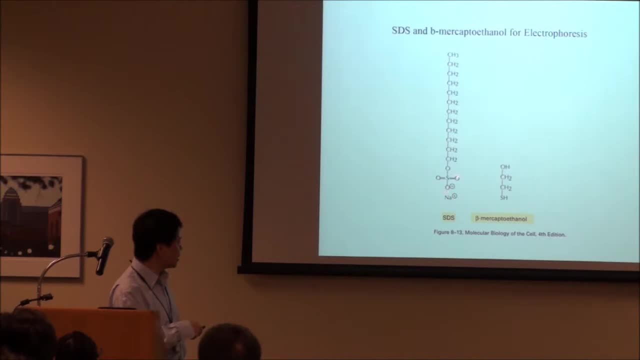 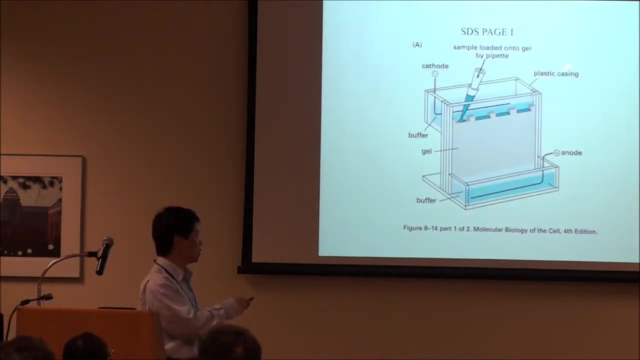 the chemicals, particularly this SDS. it's basically negative charged, right? So you can imagine if this SDS is covering all negative charge covered, is it clear? That's why this protein mixture, together with SDS, will be negative charged If you start the electrode field. 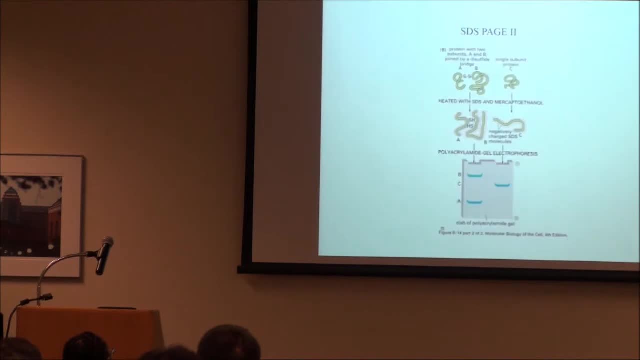 it will start to run down right And you can imagine this SDS treatment for the different molecules. You can imagine these two wells On the left, well right, This running. obviously this is one population protein. this is the second population protein. 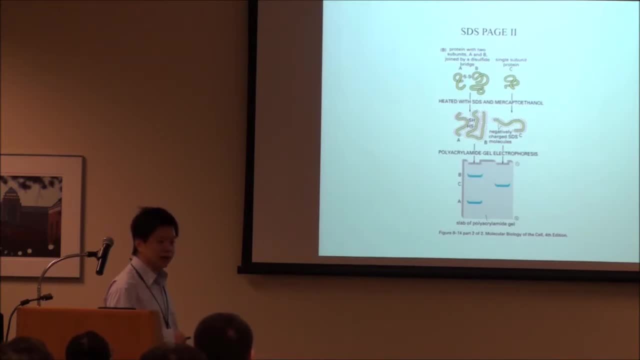 right, These two population proteins. they have different size, right? One runs faster, one runs slower. obviously, right Through this running process, Which one has smaller size? Can you tell The A has smaller size, right? Okay So? 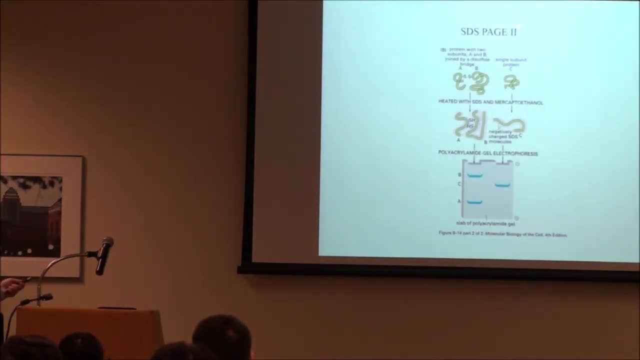 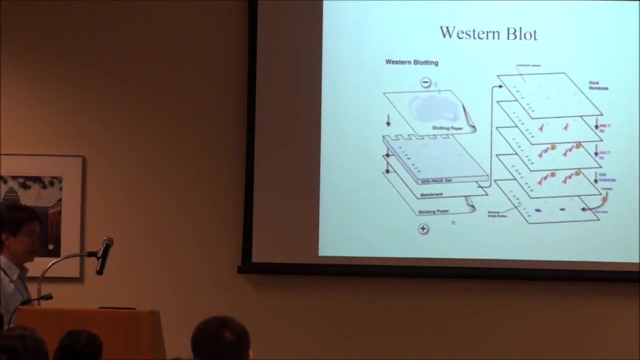 you can using these so-called SDS paid gel to separate different protein populations, right? And then that's typical way people can use antibody to stain the gel to see the protein inside. okay, This is the way how you use antibody, if you're interested. 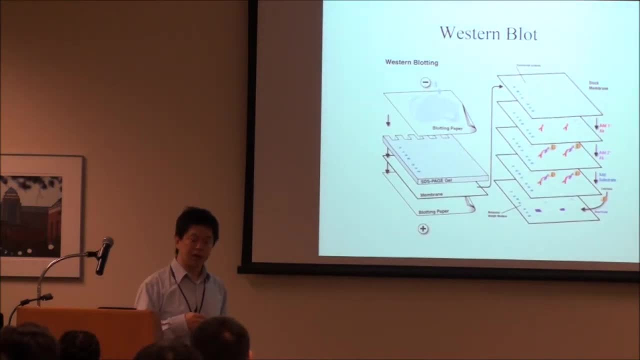 okay, Because, as we mentioned, there are millions type of cells in the cell or molecules in the cell. even after you separate using SDS paid gel, even you look at only one band, there are still multiple populations there possibly. okay, You have to use antibody to confirm. 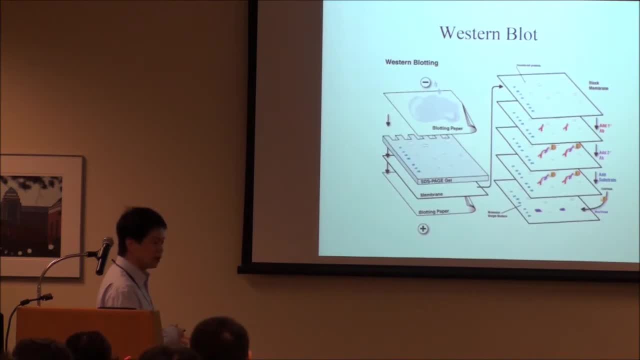 the purity of the protein. and then you add a very, very tight membrane. very tight membrane, protein cannot penetrate, okay. And you attach another two so-called filter papers and usually you also add a sponge on top and on bottom, then apply electrophiled top will be. 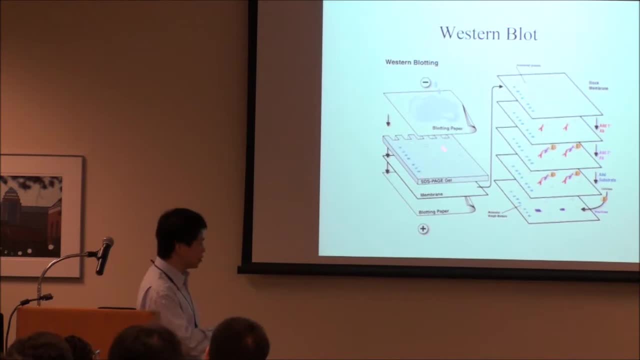 negative, bottom will be positive. if you start the electrophiled, where are they going to move? It depends on the direction of the magnetic field It's electrophiled. top will be negative, bottom will be positive. so protein will be moving. to which direction? Bottom. 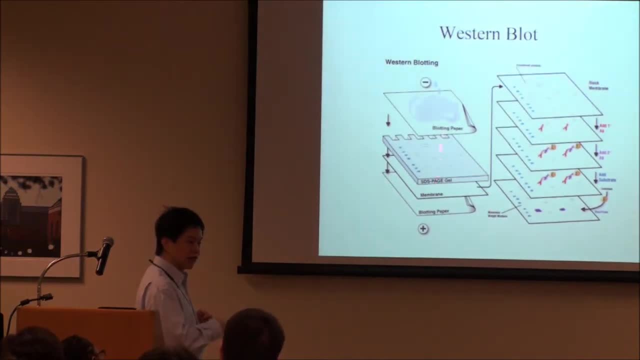 Bottom, exactly. so protein will get out of this gel, start to migrate toward the bottom and stick to this very tight membrane right. to do this experiment, you have to be very, very careful. some students, you know, when they first start this kind of experiment, they made a mistake. 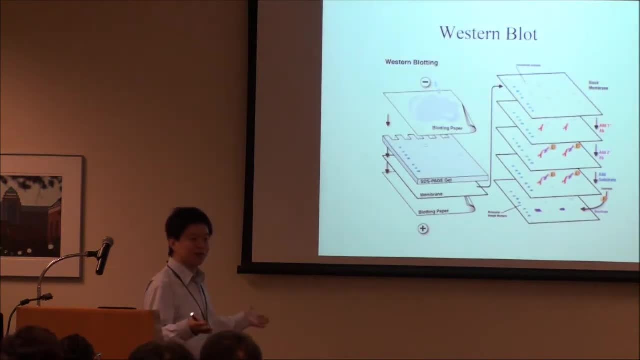 they put the membrane on top, then you can imagine all the protein will be gone, right, because they migrate out and they would stick to the filter papers and getting the solution and all protein will be lost. so this is a very, you know, very, very important step. 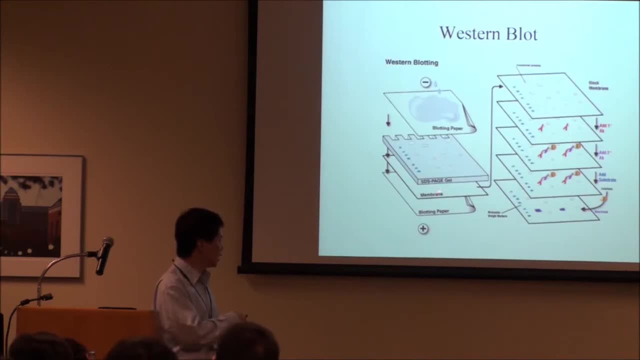 you have to make sure the membrane is on the positive side of the gel and stick to the membrane, okay. after protein is already collected right on the membrane, you can take out this membrane and add some antibody to it. but usually still you have multiple steps. 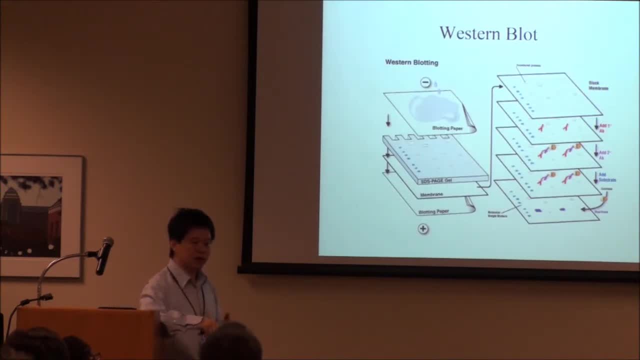 one is you first so called block membrane. you basically add the BSA or you know non, you know fat, dry milk, to coat this membrane, so that when you add the BSA, okay, then you add the primary antibody, we call it. this primary antibody will specifically: 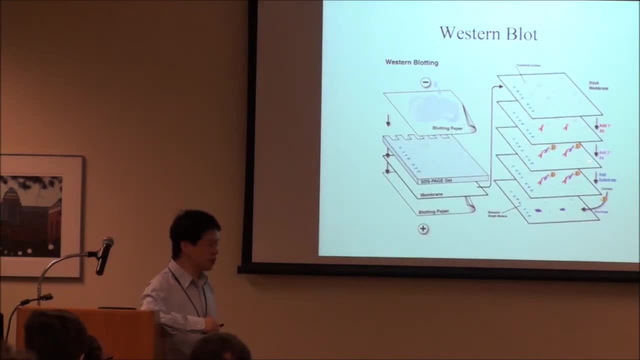 recognize the protein you are interested, okay. and then you add the secondary antibody which will recognize this primary antibody, with some kind of enzymes attached, okay. and then if you add some so called substrate with chemo, chemo luminescence, will cause some chemo luminescence. 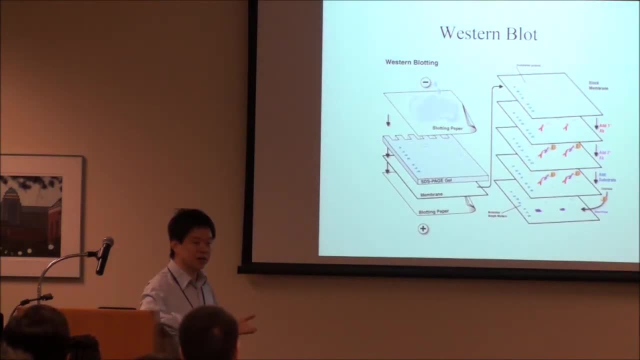 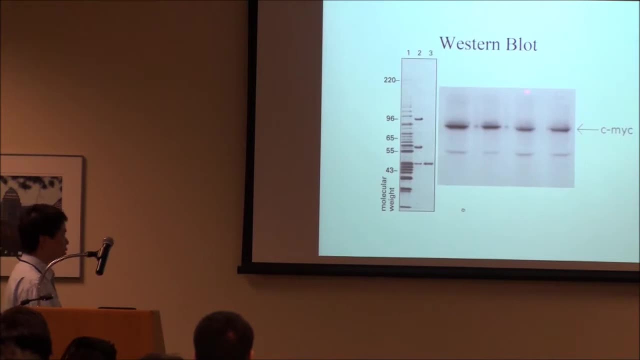 reaction. you will see the luminescence color coming out. okay, so you can imagine this will be the typical western law after antibodies, you know, staining. you can specifically see the protein. you are interested. they are in this position. okay, the reason why you can see. 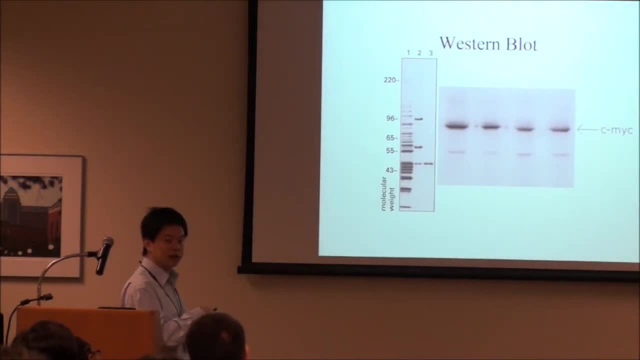 the color is because the primary antibody and the secondary antibody has the enzyme to cause the reaction with the substrate, to cause chemo luminescence reaction. for you to see the color is it clear so far now? if you have enough protein, you can use chromatography. 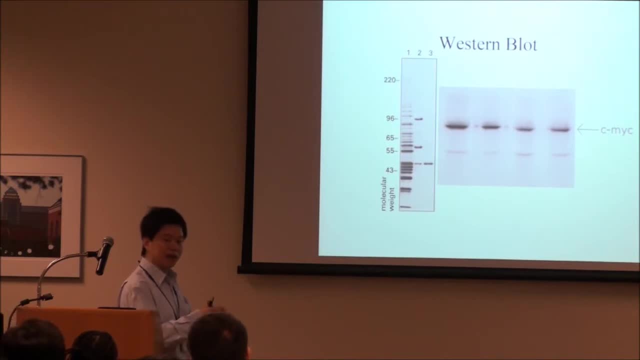 right to purify different protein populations. if you don't have enough protein, a little tiny amount of protein you run. you can recognize these proteins. okay, any questions so far. can you separate multiple components based on different colors in the chemo luminescence? 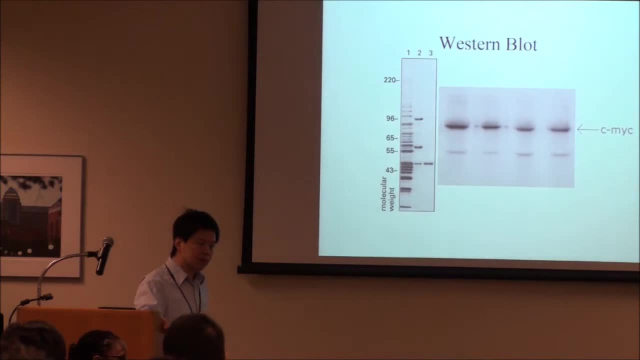 process for chemo luminescence will be difficult in general right now. so it's only one color. yeah, for this traditional, you know biochemical assay. yes, it's usually just one protein. you can see you can create different multicolor. you know western blood, but that's. 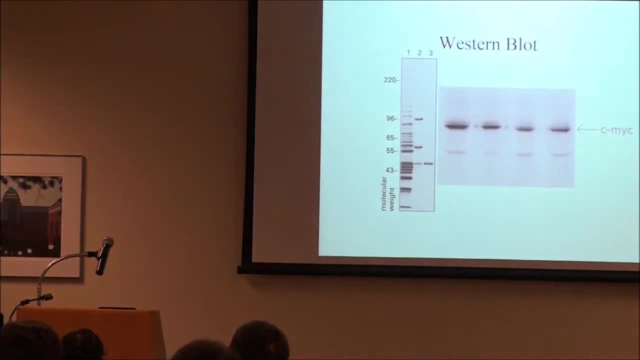 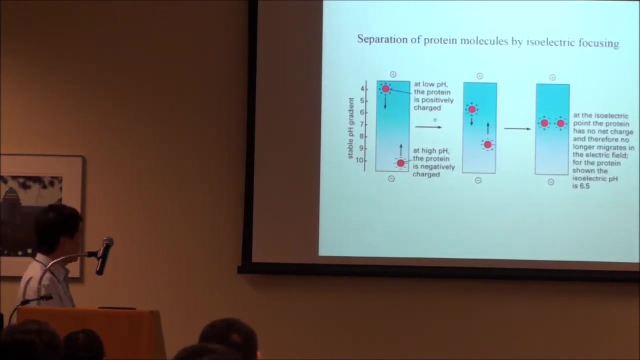 like to renew. okay, so obviously you can imagine, you know, in this kind of SDS page: okay, most of the time the separation is based on their size, right, and you use antibody to recognize this specific population, to contain multiple population or the proteins. okay, so people engineer. 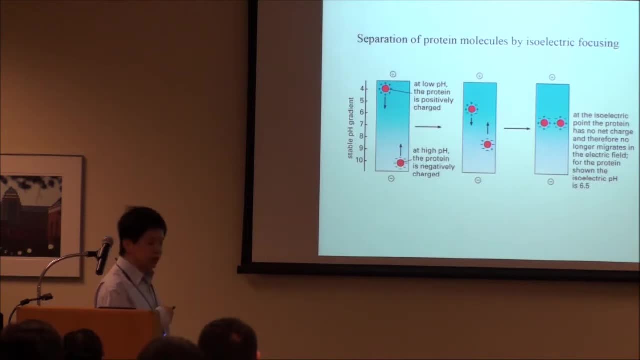 another way using so called, you know, isoelectro electric focusing, before you use SDS and separation based on size. so this concept is isoelectro electric focusing mainly is, if you run this molecule in this solution or in this gel, okay, and if you apply electrofield. 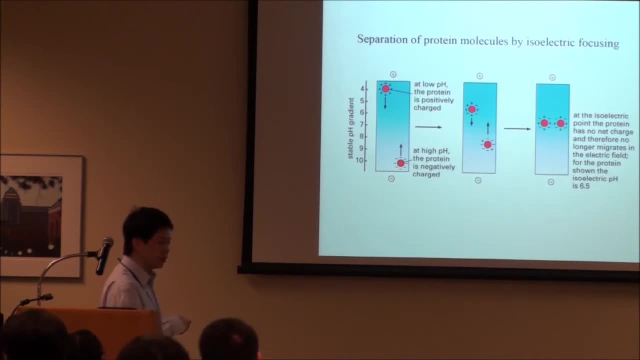 like positive on top, negative on on the bottom- this negative protein with different charges- for example, this protein at low pH, will have positive charge. this protein, the same protein, at high pH, will have negative charge. right. so obviously, if you apply this electrofield, they will start to move. 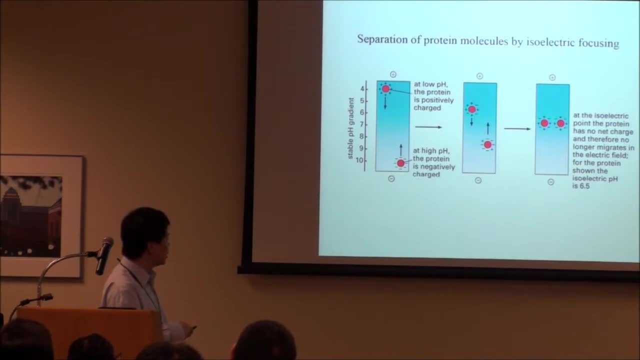 right, this guy will go this up, this guy will go down, until pH they reach equilibrium. they will no longer move, no matter what kind of charge, no matter, no matter what kind of electrofield you apply. is it clear? because they reach equilibrium at certain specific pH. 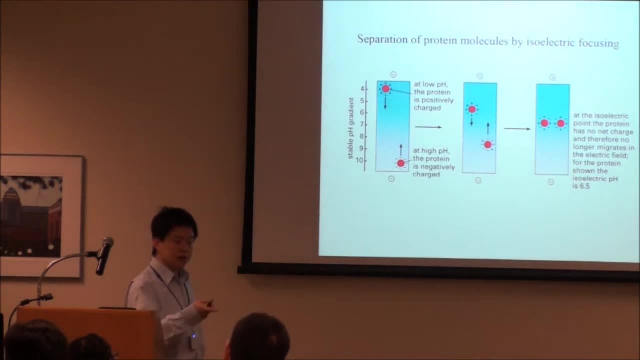 is it clear? so this, the medium, has different pH. so what is acid in the base? yeah, sorry, this is not medium, it's gel in the medium. you cannot create this. you know gradient easily because it's diffused easily, but in the gel you can create the pH. 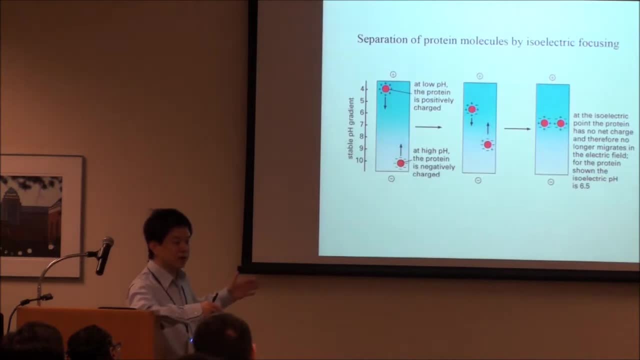 different pH. you can maintain this pH and you put the drops, for example the protein, on both sides. yeah, yeah, you can direct add, you know, load onto this. actually, one side will be okay, even you know, because if you're on this side they will move down if you're at this side. 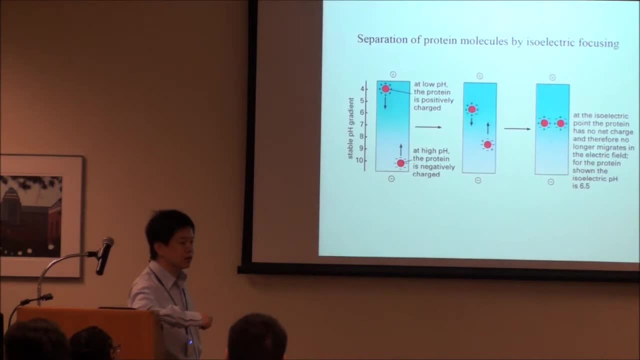 they will move up, so you don't need to have on both sides. you don't need to. they will always go to the same position wherever you load, because they only can stay into the equilibrium side. okay, so this can is another way to separate proteins, right, different proteins. 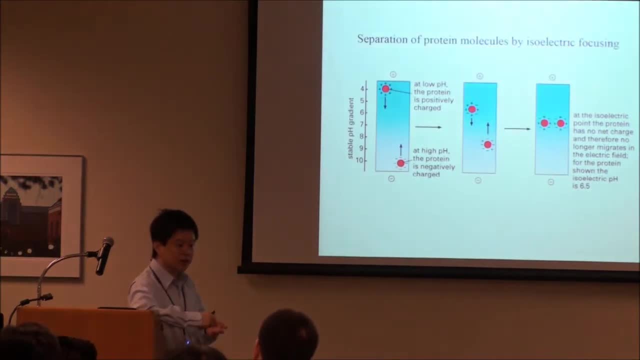 they will go to different equilibrium right, because their native charge will be different. is it clear? so you can combine this with SDS page? you first do this isoelectric focusing to separate the proteins- native protein- based on their charge. then you add SDS and separate on another direction. 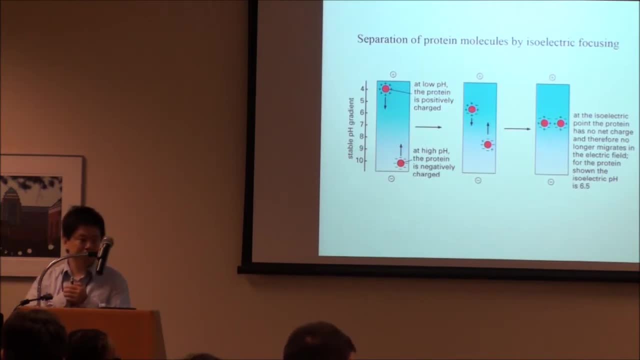 okay, question: in this process, does the size of the particles change or is it isoelectric? in this case, no size will be important because this is a native protein based on their charge, and then you can use SDS exactly after you first do this. okay, based on this pH gradient. 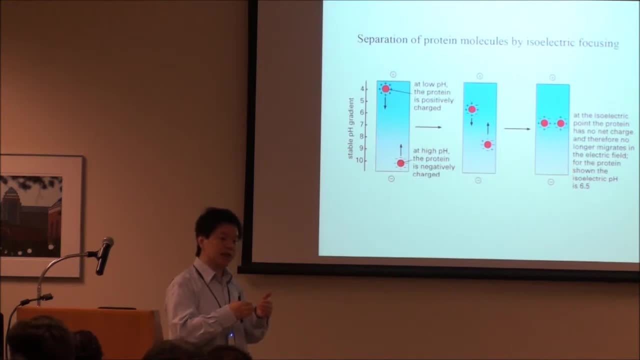 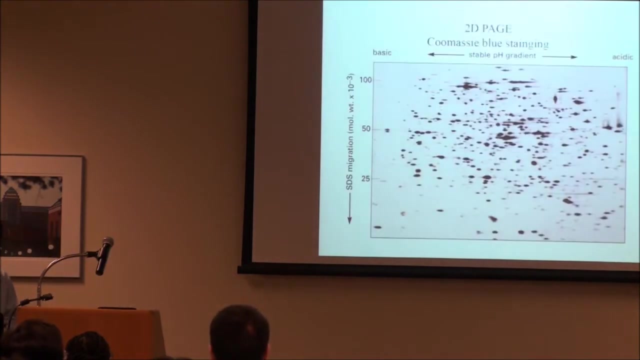 to separate them in terms of their charge. now you use SDS. add SDS along the SDS page. you know system to separate them based on size. so basically you have two ways to separate them, right, that's so called 2D gel. okay, you can imagine you first. 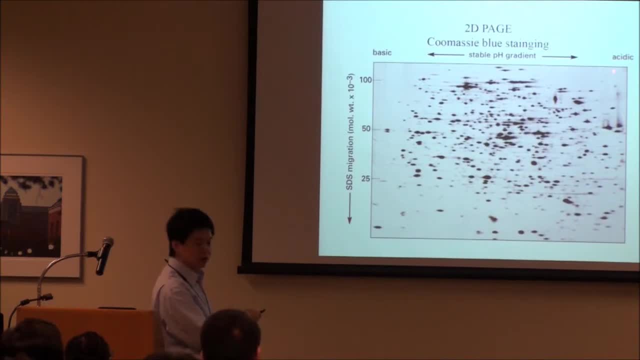 do this right on the y, on the x direction. you have very large gel on the x direction. you create pH gradient so the protein is separated on the x direction. after this is done, you start to apply SDS and run the SDS page. electrophoresis on the y. 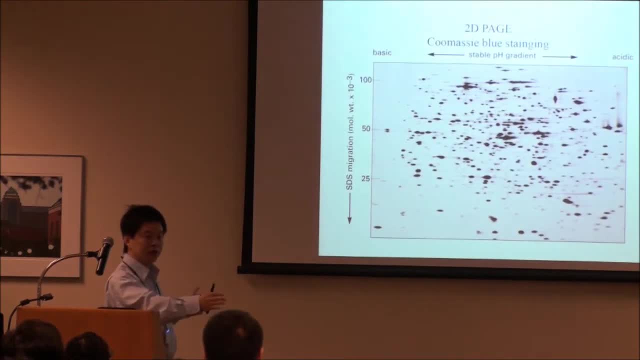 direction? is it clear? you first do this? okay, charge will help you to separate different molecules based on their charge. but still, at each charge there are multiple proteins together. right now you separate on the y. now you can see this plot. each dot will contain relatively purified protein. 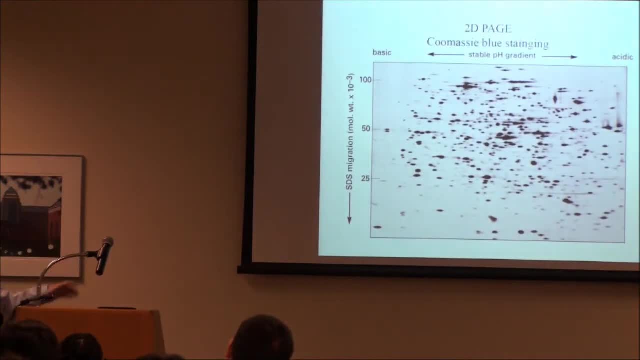 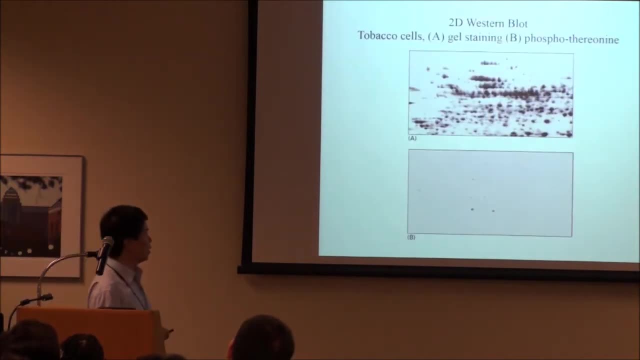 populations. so far, so good. this is purer, right, they're only using one, okay. and then you know, for example, this one: you know typical experiment: if you have tobacco cell, you just directly do this 2D gel and then you can use a western blower. 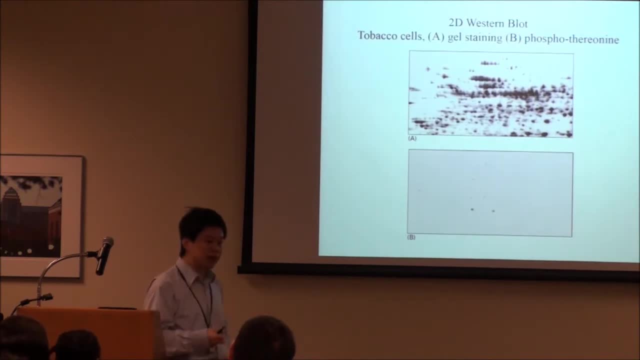 as we mentioned right using antibody. for example, if, in this case, you are particularly interested in protein, which are serine, threonine, phosphorylated, you can add antibody against phosphorylated serine and threonine. okay on the protein and you can see there are multiple. 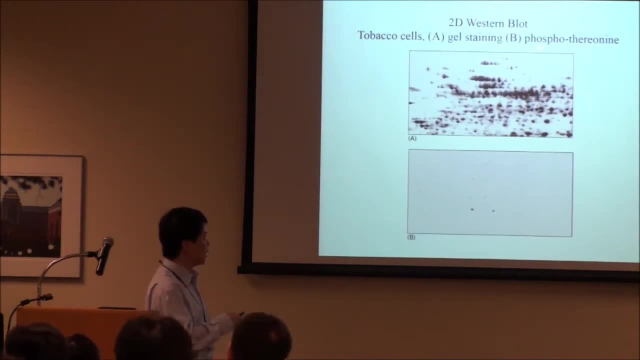 dots here, here, here, here right, the bottom gel is the protein which are serine phosphorylated. you can see, among these millions of- I wouldn't say millions, maybe thousands- of different kind of proteins, there's only limited, you know, protein which are serine phosphorylated. 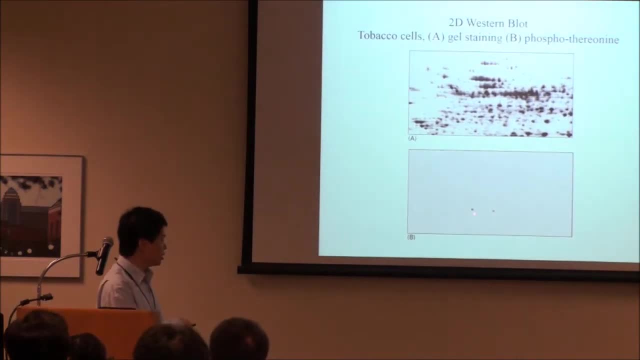 is it clear. so each dot, if you can match. there you can see this population. the protein are serine phosphorylated. okay, you really can. you know, know what kind of protein? actually, you don't know what kind of protein yet, you just know this size and this. 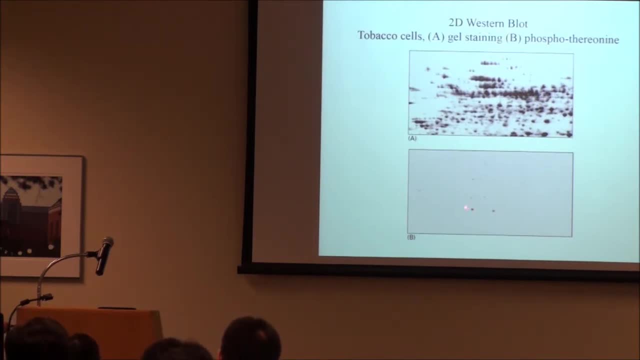 electro. you know, property of the molecule is serine phosphorylated, right? you still don't know which protein exactly it is right, you don't know yet right now. how do you know it? how do you know it if you already do that and you know there are like 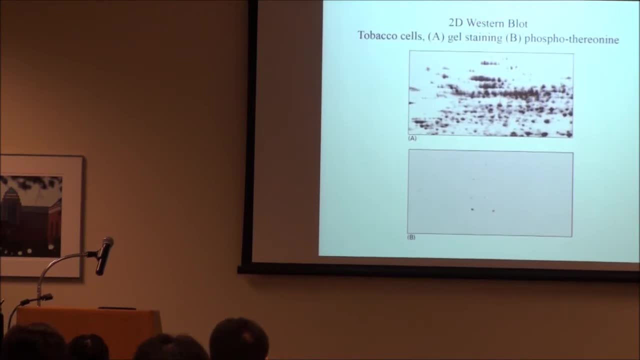 five or six molecules are serine phosphorylated and you want to know which protein are they exactly. do you know how to do that? how to find them? use antibody? yes, you already use antibody and you already find out. okay, these proteins are serine phosphorylated. 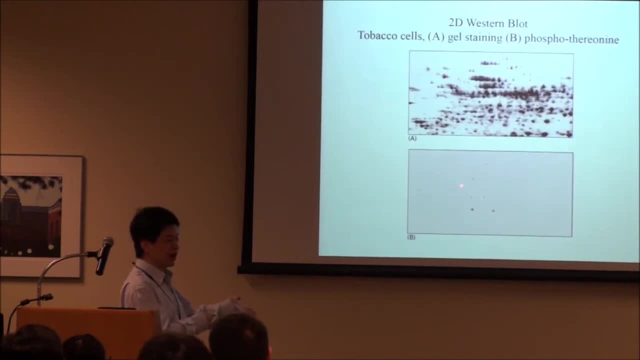 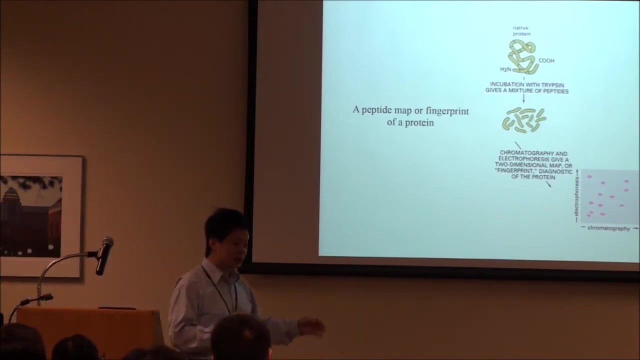 but you don't know which antibody you should use. right, because you don't know what are they. how do you find out exactly? that's the exactly the way you should do. so the principle for mass spec is very simple. basically, you have a protein, right, you can. 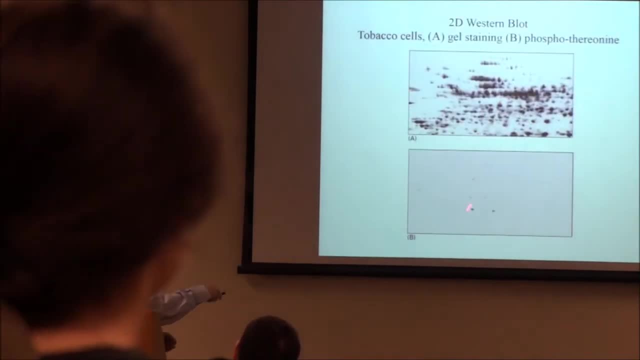 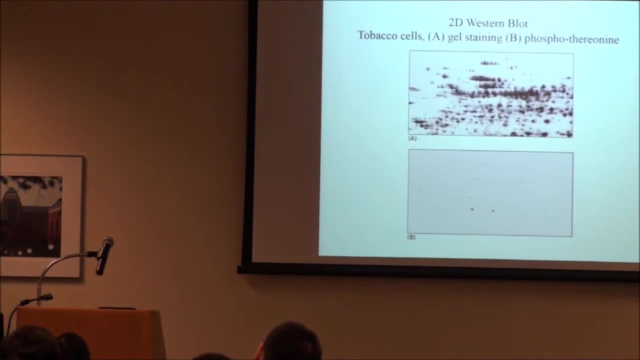 you know, for example, in this gel, you can basically, if you already run all this and you can just cut out the protein from this spot, right, and you can chop this protein using enzymes. these enzymes, a lot of time they will recognize lysine in the protein, so they can be. 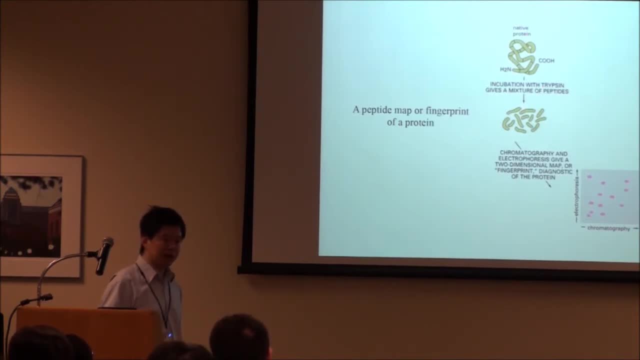 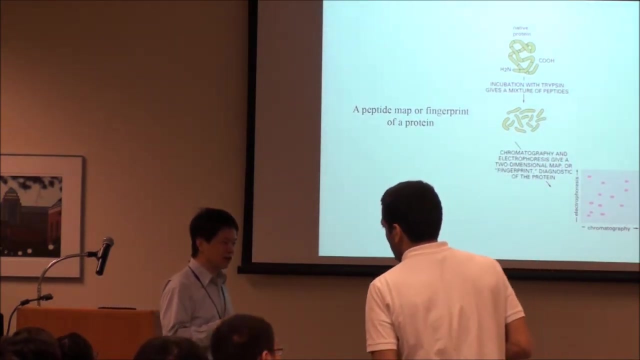 chopped into like multiple pieces, okay, and if you run like 2D gel or whatever, you can create a profile, okay of this specific protein. okay, and the lucky thing is we are living in a modern society, right. so there's millions of you know. work has been done. 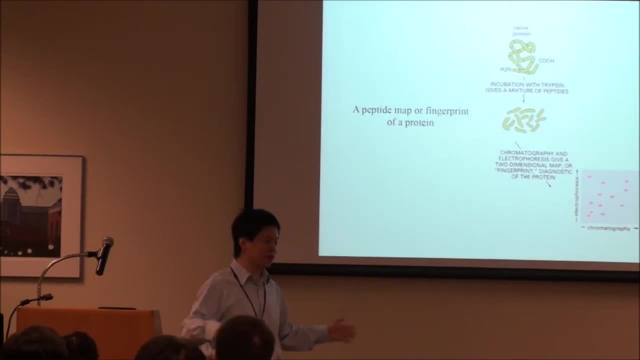 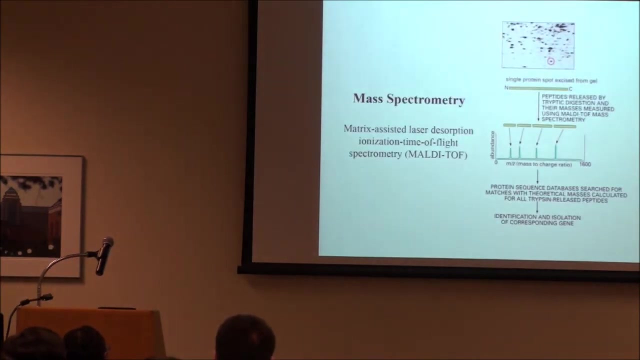 people already chop all these proteins and already create a library, so they know exactly which protein has different. you know which protein has different kind of features. is it clear now you have multi right mass spectrum. okay, you have run this 3D gel and this dot you already? 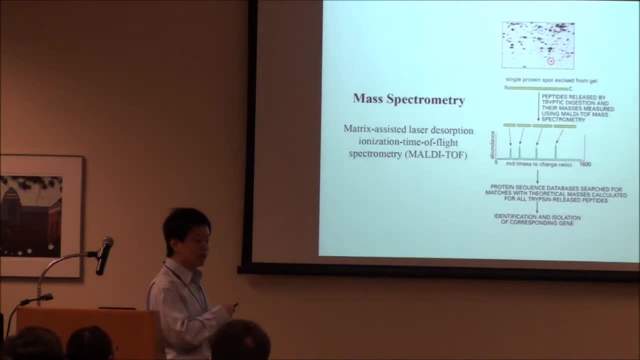 identified. for example, this is phosphocyrinine modified right and you want to know the protein. you directly cut this protein out. you know in the gel you can cut it out right and chop it and you run mass spectrum to find out abundance of the different pieces. 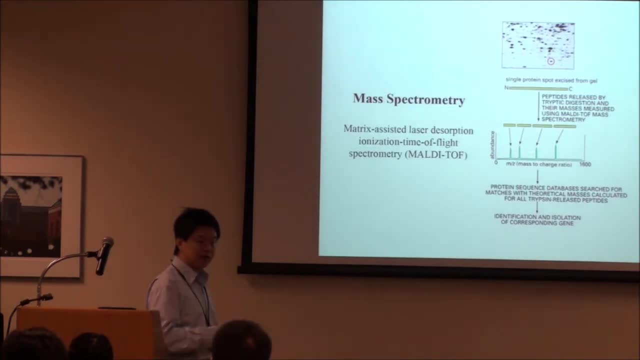 okay, you will get the profile. is it clear? after you got this profile, you input this profile into a library and screen to see whether this profile match an existing profile protein. just like you know fingerprints right, if somebody got caught, they will get the fingerprint through the library. 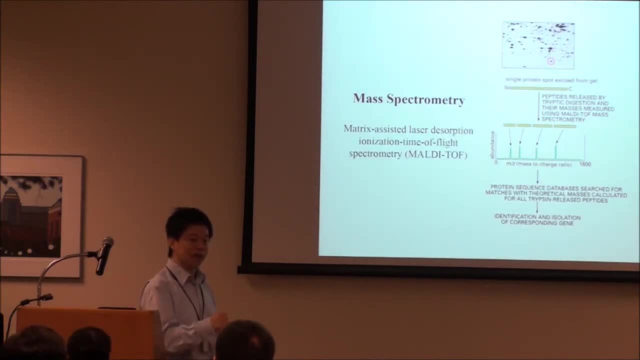 right to see whether it match to an existing fingerprint and they will know this fingerprint belong to this specific person in the library. is it clear? same thing: you run, you know, cut this protein out, chop it up, become multiple, you know, small pieces, you create a profile, right. 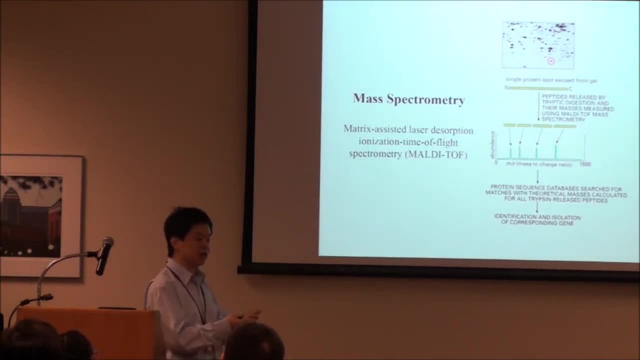 and this profile will be key in into a library and start the screen and to see whether it match to an existing protein. okay, so this protein already has been chopped and create profile. right, if these two profile match, you know this protein. you can know the identity of this protein. 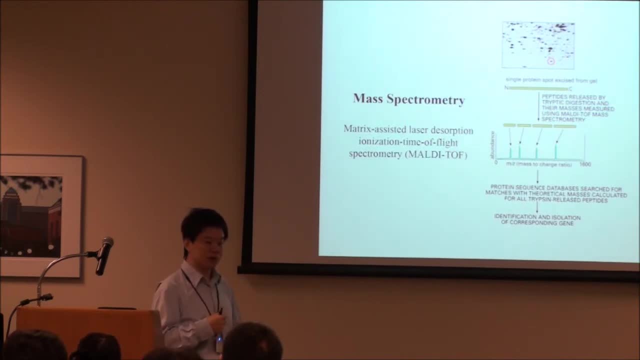 in the library. okay, the assumption is all the protein in the cell has been already, you know, purified and chopped and create this profile there, right, is it clear to you? okay, right now it's pretty much every single protein you know in the cells has been already created. 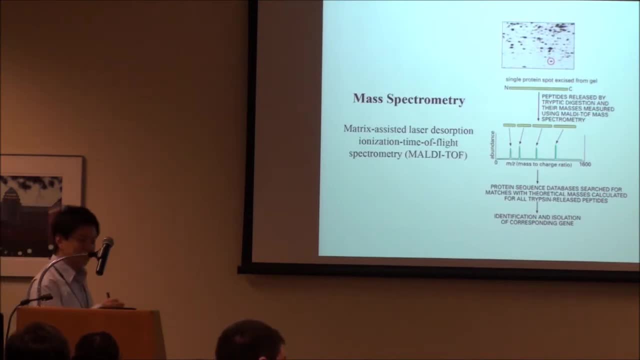 in terms of their profile. right, when you say that you're using enzymes to chop this protein, you're talking about proteins separating. so is this one single type of molecule, now that you're breaking into sub components, or are they different molecules that you separate using enzymes and then you 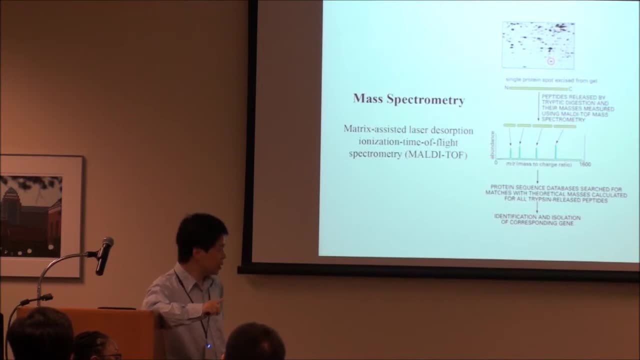 run them. run them through the mass spectrum- very good point. so I'm assuming you, after you go through this 2D right gel, if you just directly cut out this spot, it's only one single type of protein and you just chop it into different fragments like peptides. 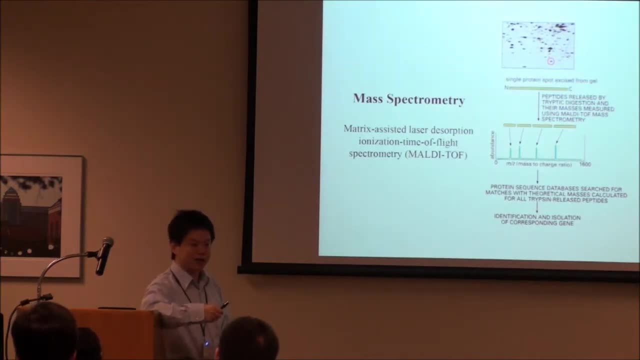 right and run the profile and you match it. but of course it's just ideal case, right? sometimes, even if you cut one spot, there are multiple proteins there. okay, but still you can cut it using these protease, cut into different peptides and run this profile and you can. 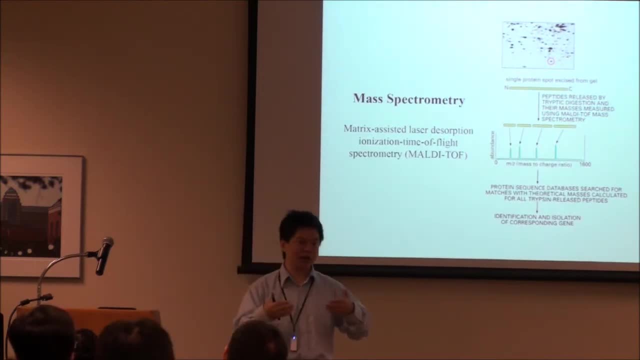 you know this. I don't know how many have already pre-experienced. you know, in terms of how to match profiles, for example, this: you know the protein in the library. you can easily find out as well. of course, the ideal case is okay. this spot only has one. 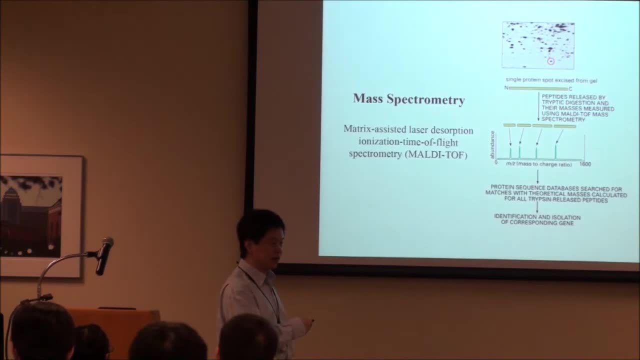 single type of protein, then your job will be very easy. right? you create this profile, run the library, match. okay, you know the identity of this protein right away. right? but other times, this spot, run the library, you find out none of them match. but if you do a little bit more, 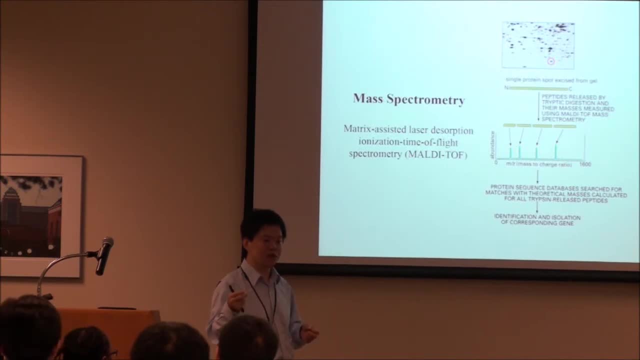 investigation you can easily find out. actually, if you combine two protein profile together in the library, it match your profile. then you know this spot contain two known protein in the library. is it clear? of course this probably require you know a real analysis between these profiles and how that matches. 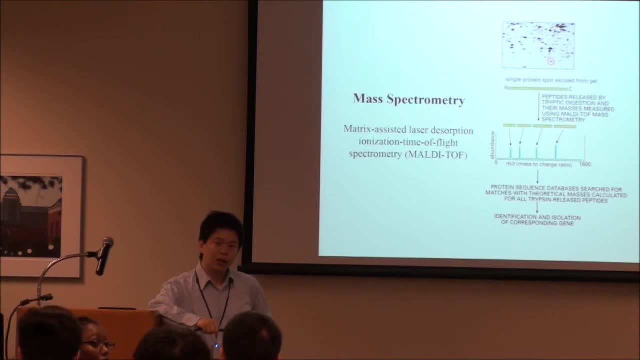 another type of protein? that's unlikely because you know all these- let's assume all the library proteins. right, they are single proteins. people already purified and create this library. okay, any questions so far. so I guess after this you are really a master, right, you can identify proteins. 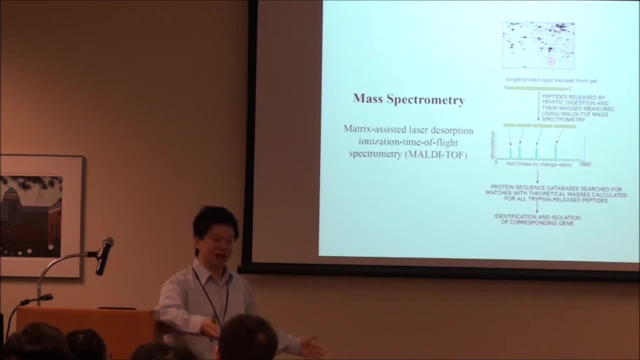 purified cells. right, and you can identify whatever protein you are interested. right if you combine all these together. right, if protein is large, you can use chromography to collect the pure protein population. if protein you can obtain is only small, you can use. you know, SDS page and 2D. 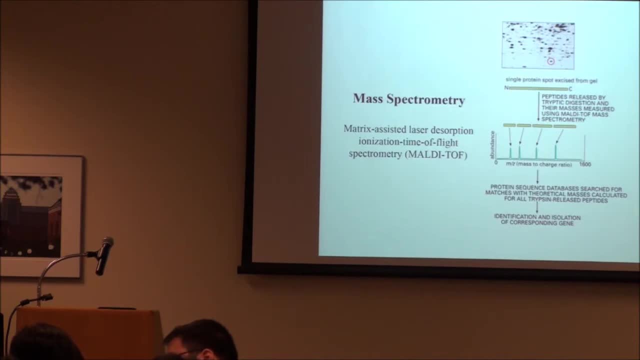 gel separation to identify these proteins, right, because transferring that onto a membrane is probably going to be very difficult. okay, yeah, that's a very good point, very, very good point. so, in general, if you are really doing that kind of you know study, right, you don't do it. 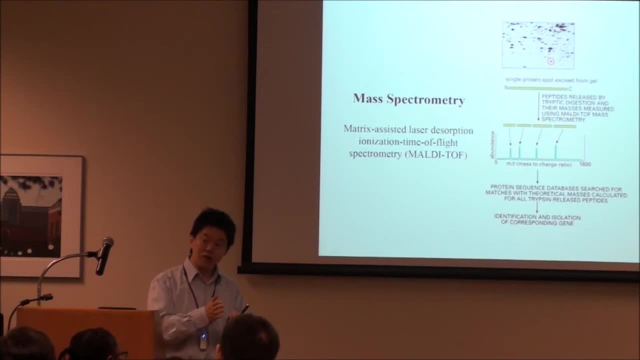 just at once. okay, what you do is- you know you can not. you don't transfer everything to the membrane. still, the majority will be left in the gel in the right ear. you can do it in the lab. you can run this western to transfer a small portion. 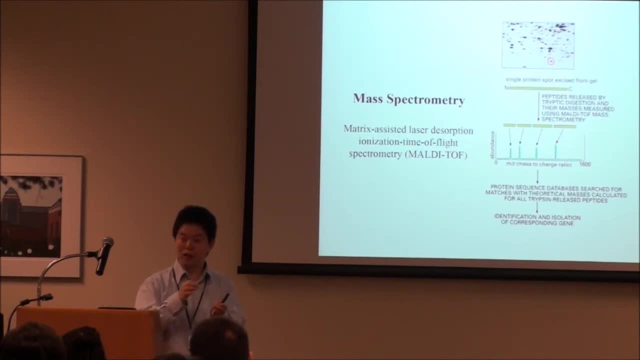 of the protein to the membrane and you stand right and identify this spot using antibody and you match this membrane to the gel back again and cut out the spot in the gel. okay, so actually the purification, all the protein purification, is still from the gel, not on the membrane. 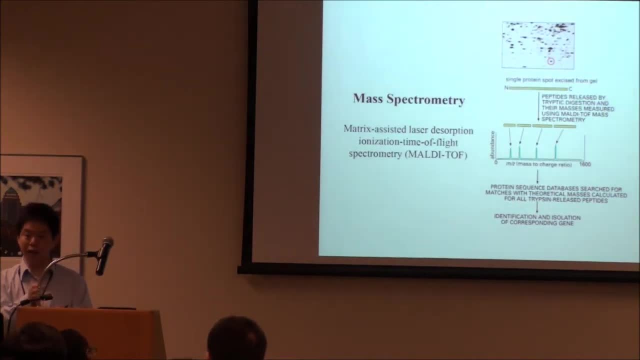 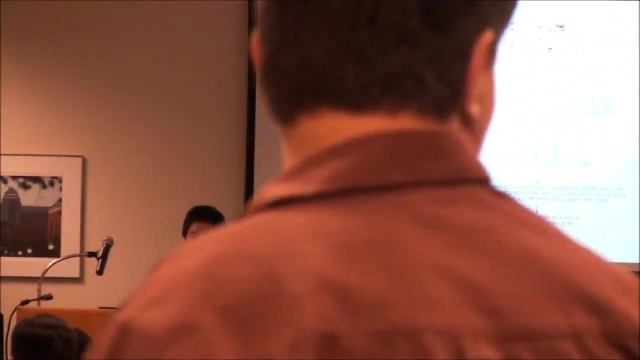 okay to find out or identify the spot where the protein is localized in the gel. yeah, that's a very good point. in reality, you have to. you know, probably you have to collect anything, spot, right. you can run another gel again to separate, right. you know, most of the time 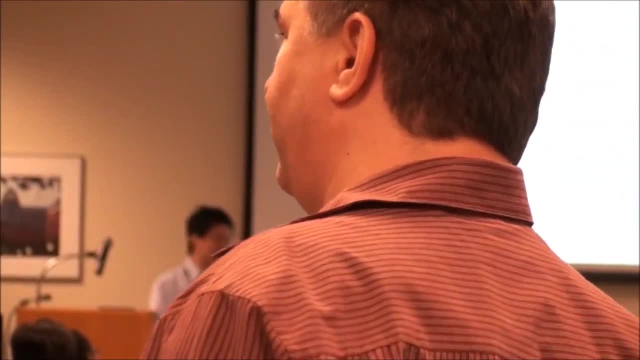 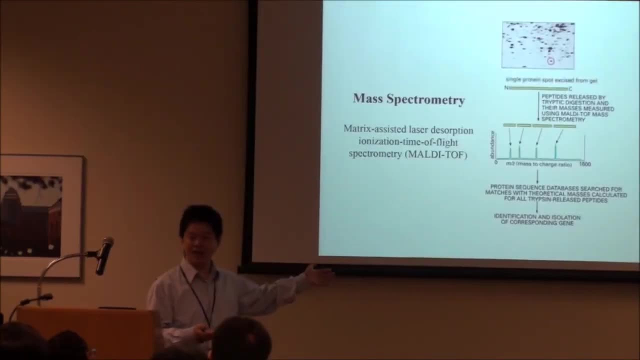 you know when we are getting to the lab. that's why people two or three years one paper right, not like two or three weeks of paper, mainly because the reality of these protein purities right. so, for example, if you are particularly interested in protein in this corner, 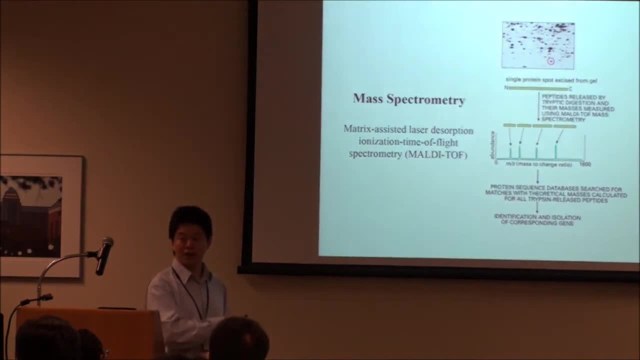 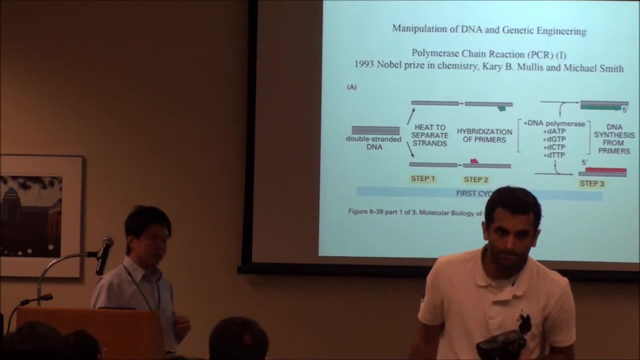 yes, you have to cut it out, run another gel again to separate further and of course it will be purer, right, because you discard all the rest of protein. okay, so this you pretty much know: the cell and the proteins, and because the revolution of molecular cell biology. 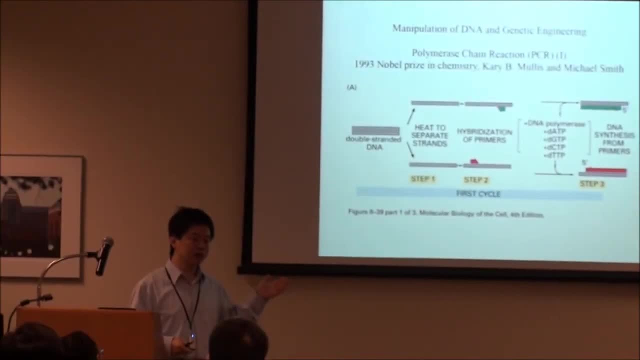 and now they can also provide very, you know- powerful tools for you to manipulate cells. okay, not only you can directly analyze and discover what's going on in the cell, but then these manipulation can provide you a lot of power to identify certain specific functions of molecules. okay, 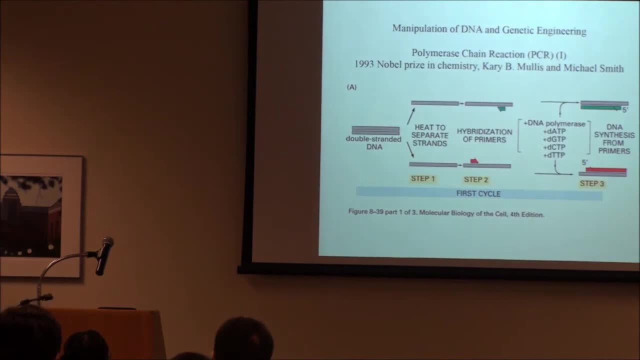 which I'm going to introduce some basic principles- I think most of them you probably are already clear- such as like PCR, polymer chain reaction. how many of you already know this? many of you right? okay, so this is basically you know. I think Nobel probably also added the. 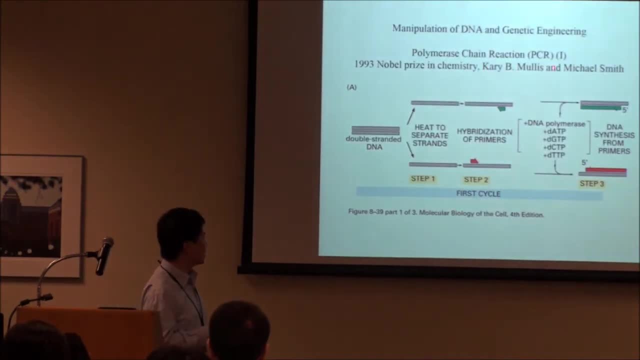 technology right in 1993, Nobel Prize, and this is actually the main inventor. you know Morles, he's a very interesting guy, you know he's in San Diego, you know, basically really a playboy. you know type of person. you know surfing is a major job of his. 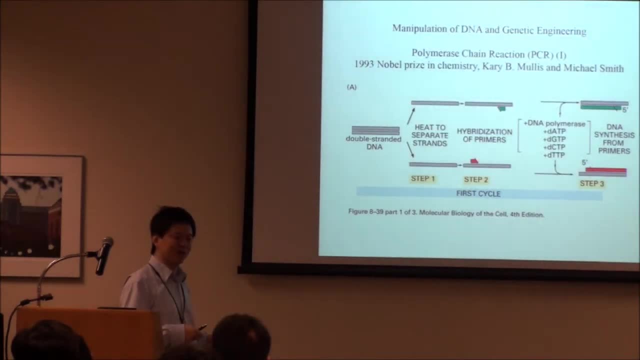 you know life and actually when the Nobel Prize was announced, he was also, you know, on the board, you know surfing. so anyway, the first thing is DNA. okay, before the PCR is generated, people always have difficulty because we all know whenever or whatever you are doing, the technology. 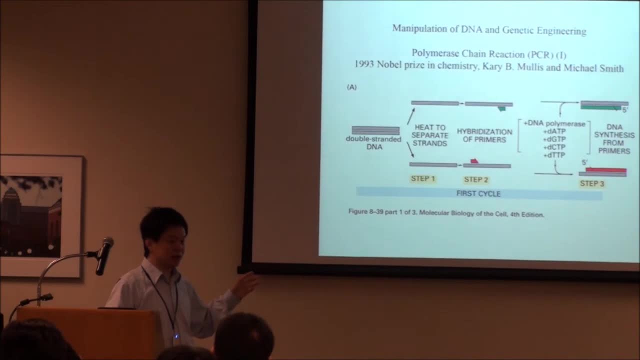 amount is always the key. right amount is always the key. if you don't have enough amount of protein or enough DNA, it's always difficult for you to do anything in general. so you need to have the knowledge to amplify DNA segments, whichever you want. okay, the idea is: 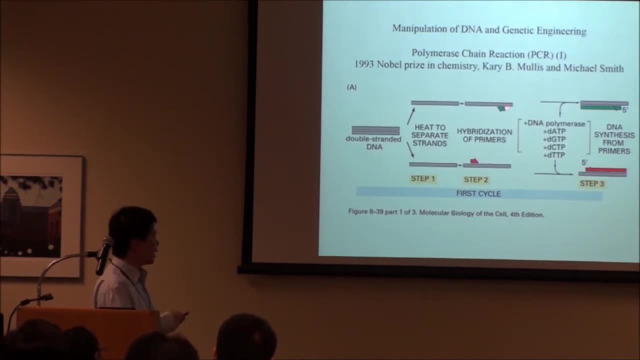 you have a DNA double strain. you know that right. if you want to amplify a specific section in the middle, you can design so called a primer, a small short piece of DNA. they can be matching to the these two sides, okay, and use high temperature to separate this DNA template. 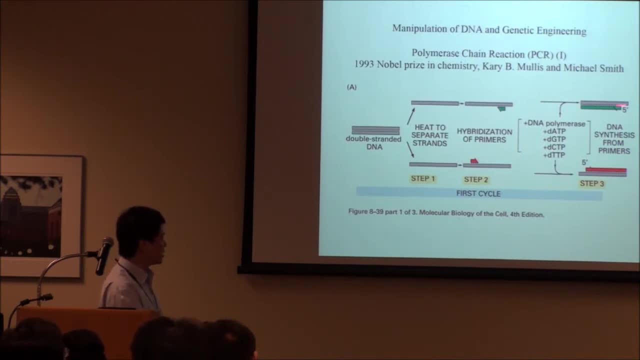 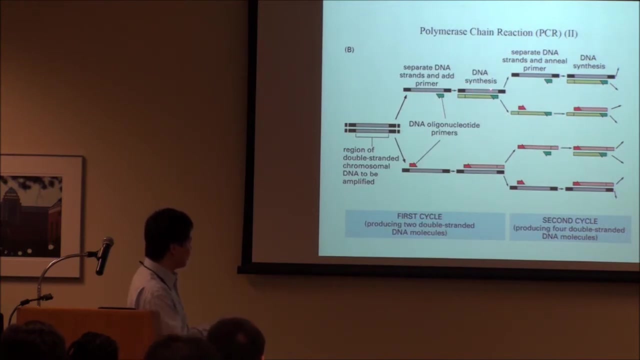 and ATP, GDP, CTP, whatever- and synthesize the protein, new DNAs- okay, this is so called first cycle. you can repeat this cycle- okay, first cycle- and that second cycle. after you synthesize from this first cycle, you separate them again and do the second cycle and you can see. 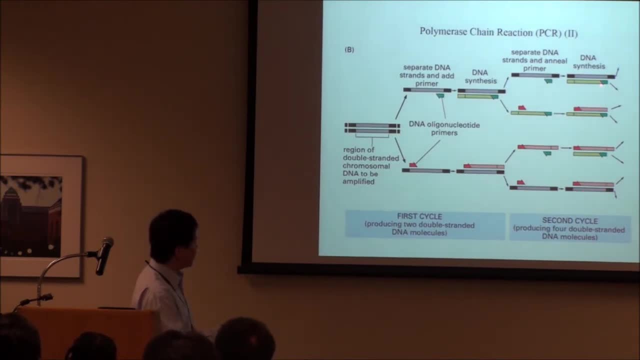 already this DNA template, this black thing. you can see already this, this and this and this. they become linear, increased. second cycle: you have four copies and the segment which are you are specifically interested, this segment and that segment which is encompassed by a section. you designed only have two copies. 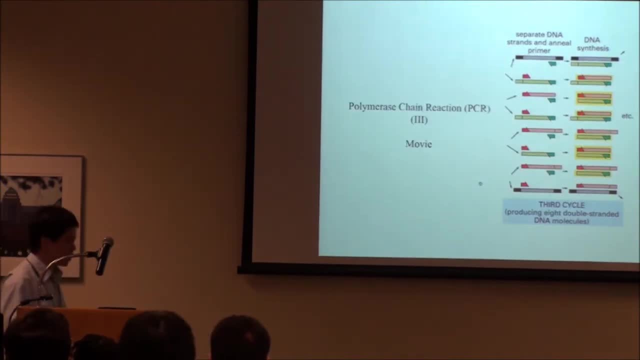 at the second cycle, okay, magic happen. in the third cycle you do the same thing again. okay, you will see. after third cycle: okay, the DNA template, the parental DNA template, still remain. two, right, and this segment which has some kind of one side over here. one, two, three. 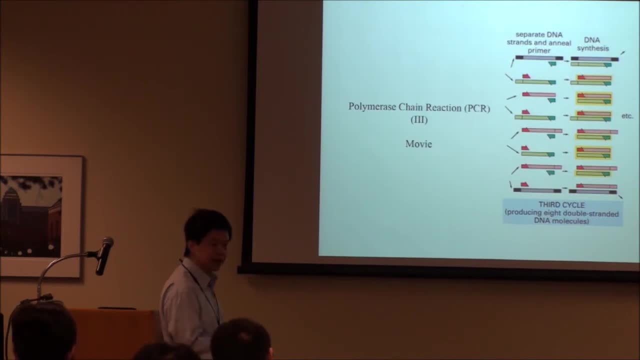 four, five, six, linear increase right. third cycle: two times three, six, right. and look at this segment which you are interested. yellow highlighted. you know this: one, two, three, four, five, six, seven, eight- it's already eight. okay, this same magic will happen if you run another cycle, this segment. 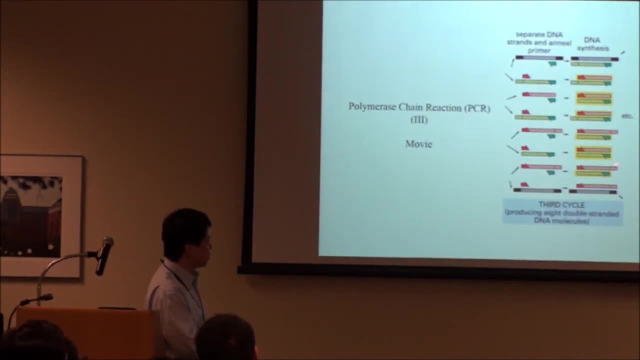 will exponentially increase. okay, and this segment with like little one side over here will increase linearly and the parental DNA will stay the same. so if you can imagine, if you run like thirty cycles, what's the majority of the DNA you will generate? exactly. so this you know. 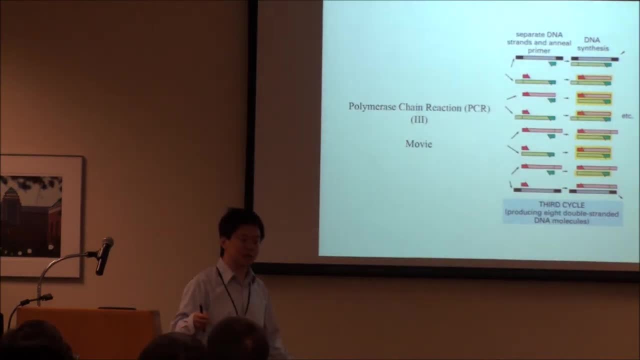 type of DNA will be exponentially increased for thirty times. right? so after you finish the thirty cycle of the PCR, the most majority of the DNA you collect this. other things are really negligible, right, because this will be linear increase. not much, right? this will remain the same, okay. 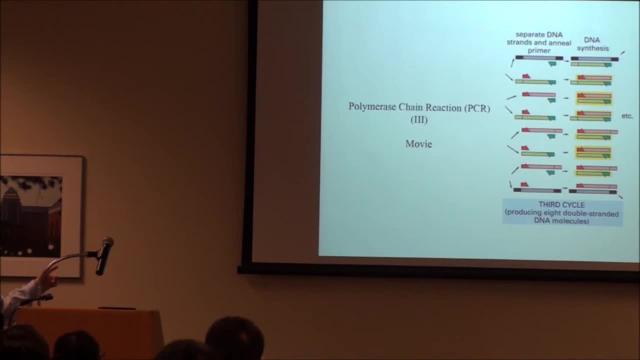 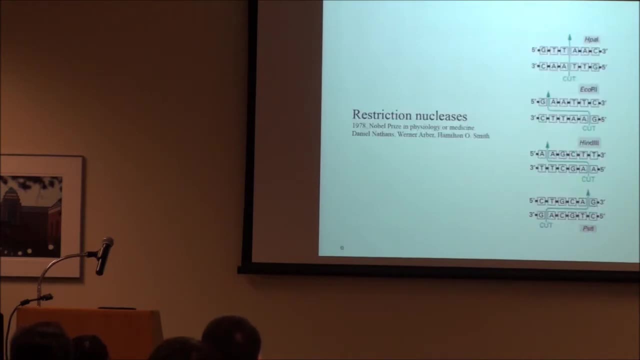 so PCR can allow you to amplify the development. okay, in a short time with large quantity, is it clear? okay, so this is the PCR which will allow us to collect enough for DNA. another technology is so called restriction nucleus. okay, so this is also Nobel Prize 1978. 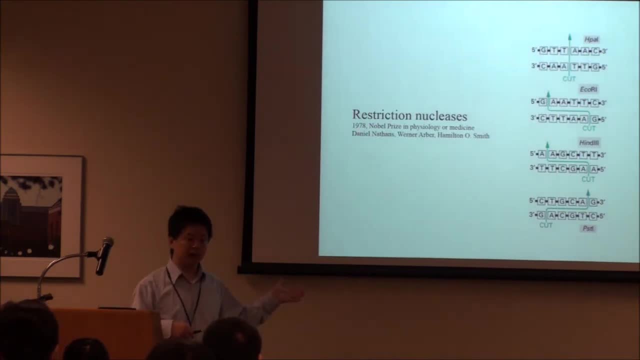 also provides a huge power for the molecular biology revolution. basically, the principle is they found out this specific enzyme which can cut the DNA. but the good thing is, each enzyme will cut and leave a very unique interface between cutting site. it's just like in Legoland, right? 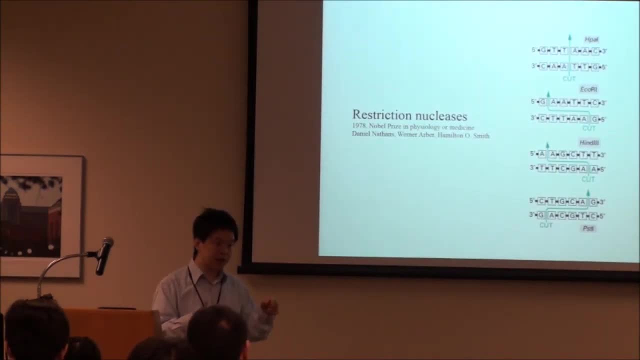 or a puzzle, right, it creates specific, you know, interface. that's how you can piece the puzzle together again. right, because they have unique interface. each enzyme have their own unique interface. okay, you can imagine, after you cut, only this specific site can be, you know, pieced together. 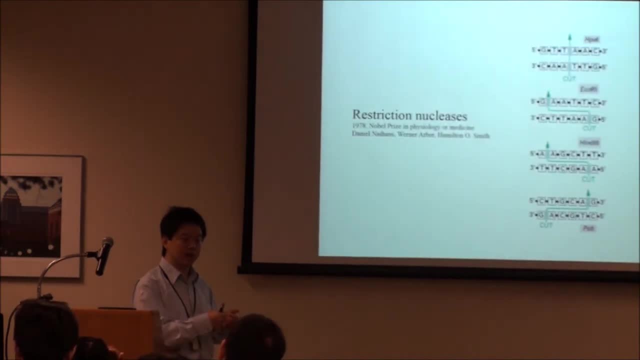 so if you use the same enzyme to cut two DNA fragments, pieced them together, you can connect two different DNA together. right, because they have the same interface. okay, and these there are different enzyme. you know DNA enzymes which can help to join the DNA together. this is not. 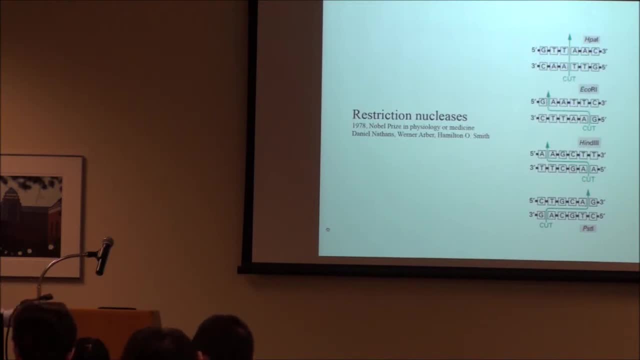 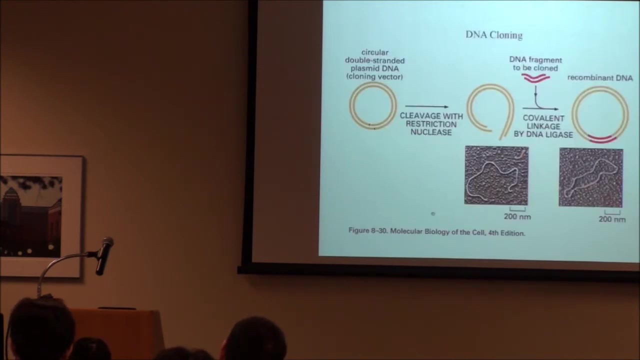 as important as these. you know nuclear specific cutting site, but these also provide power for you to, after you cut, you can join them. okay, if they are cut by the same DNA restriction nucleus. okay, now, with all these together, you know you can create enough of DNA. then you can. 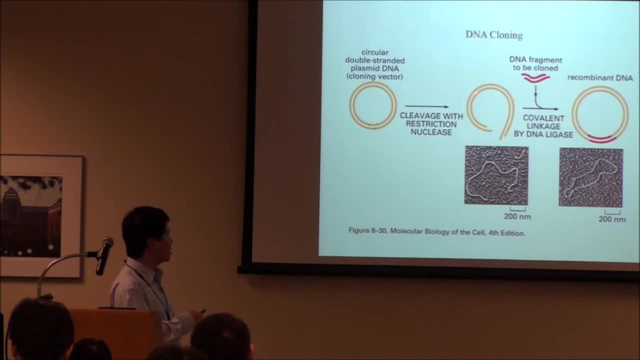 insert them into. you know so called circular double strand DNA and this DNA can be put into for things. for example, you have circular DNA. you can insert a DNA fragment using PCR to amplify, cut with restriction nucleus right and if you cut using same restriction nucleus they will have. 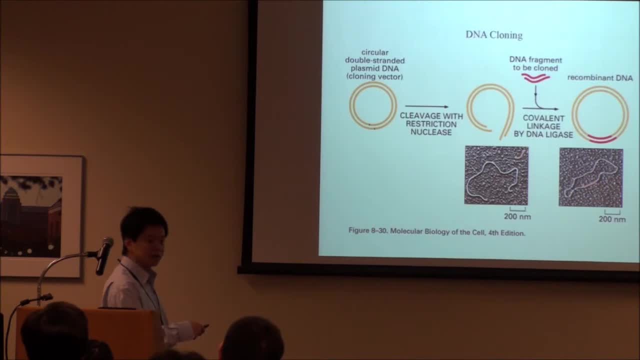 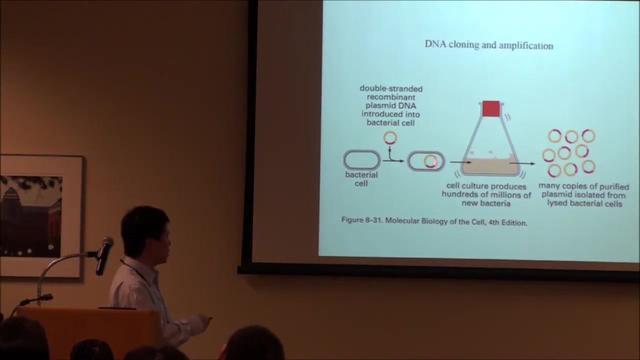 same site so that you can perfectly match and using DNA ligase to put them together. is it clear? have to use the same restriction nucleus. if you use different one, you cannot insert. okay, now, engineered plasmid or DNA you can put into bacteria. bacteria continue to grow. 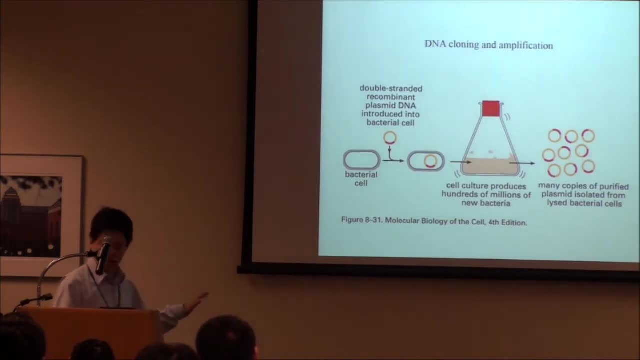 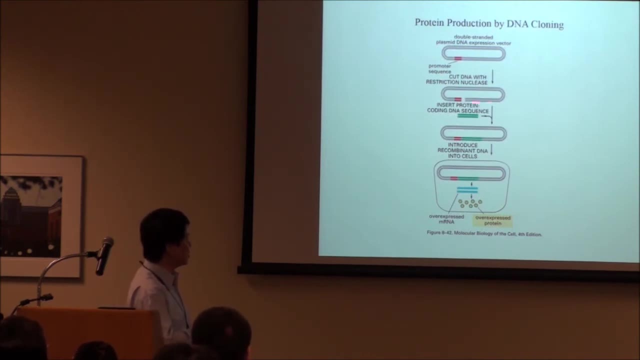 and amplify the DNA. now you got tons of DNAs right, but that's not about it. there are some other things you can also, you know, enjoy. basically, after you engineer these DNAs, okay, you can put into bacteria. they will not only amplify DNA, they can also. 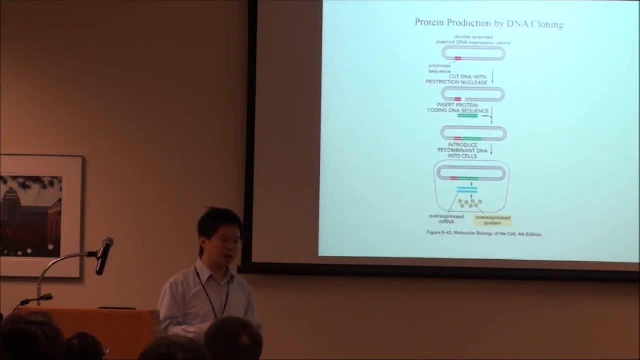 allow you to acknowledge, you can pretty much engineer and create large quantity of protein whatever you want, because all the protein are controlled by gene sequence. right, if you know the gene sequencing, using PCR to create the DNA insert into this plasmid, you can create the protein you want. 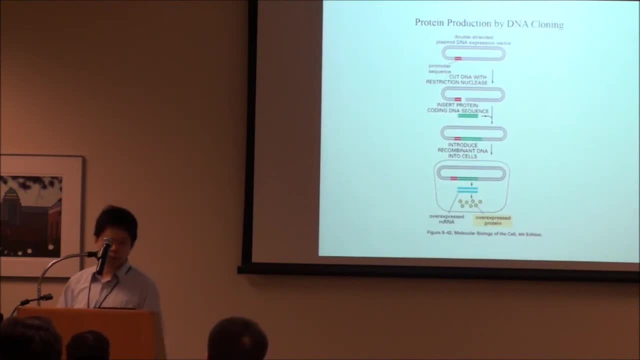 with high purity and large quantity. is it clear? how do you think the DNA inside the bacteria is like diffusing? how? that's a very good point. so this is so a transformation. you know, I didn't in detail describe this here, but in general you have bacteria. 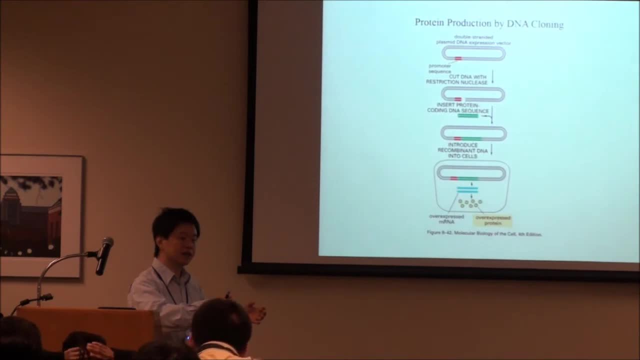 right, you mix them together with the DNA you already create. right, and usually people do a so called heat shock, so the membrane or the bacteria become permeable and the DNA will diffuse inside the bacteria. okay, and start to, you know, incorporate into bacteria system and amplify DNA. 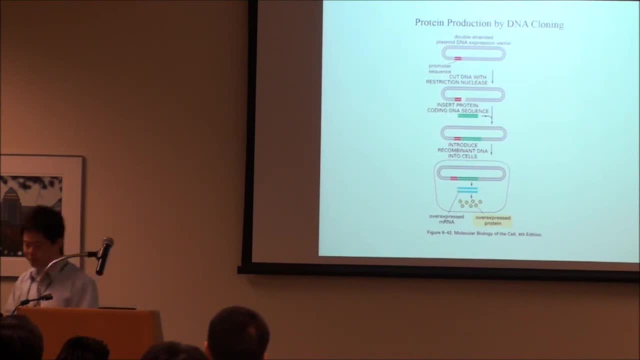 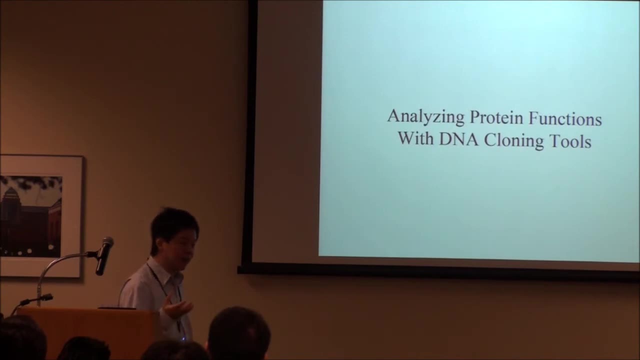 and the protein you want. okay, now you know the DNA technology. you can use DNA technology to manipulate the genes right to create protein you want. okay, what kind of wonderful things you can do with this technology. I want to introduce a couple, and then I should be done. 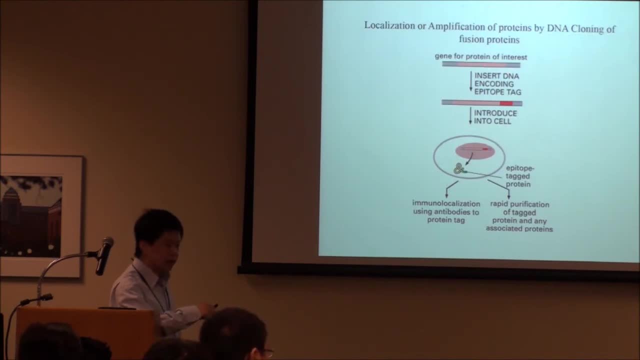 one first thing is, for example, if you have a protein, you know it, you know the gene sequence, but you don't have antibody available for it. because antibody you know, you have to rely on a company right to create antibodies, right, if there's no such antibody available. 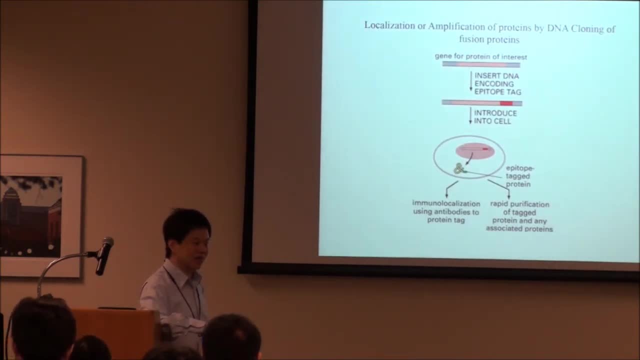 what I'm going to do. of course you can say, oh, I will just generate antibody, that you know. I can assuredly tell you that's painful, you know. okay, then genetic engineering can help you. okay, to amplify or purify this kind of protein in your lab. 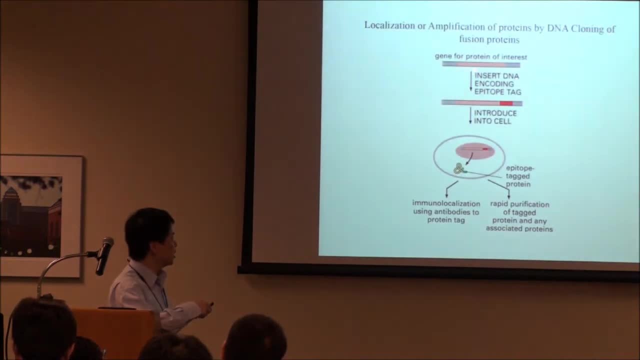 okay, the way is you can easily engineer the gene sequence, because that's you know. you can easily, you know, download from the PubMed and then insert a known- okay- gene sequence which can create a very cheap peptide which can be used to generate antibodies, for example his tag. 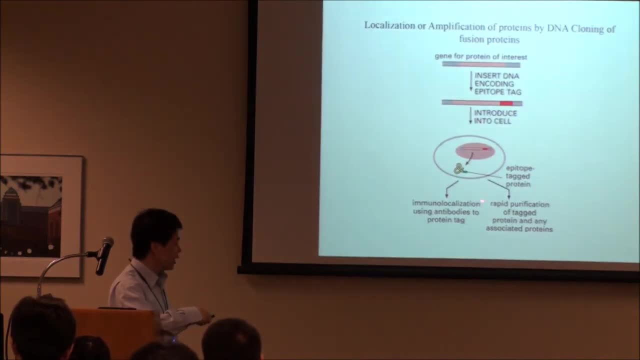 or flag tag, okay. then you put these two together, okay, and then put into bacteria and produce the protein. so this protein has the protein you are interested. also has the epi tag. epitope tag, peptide. okay, now you don't need to generate antibody, you can direct. 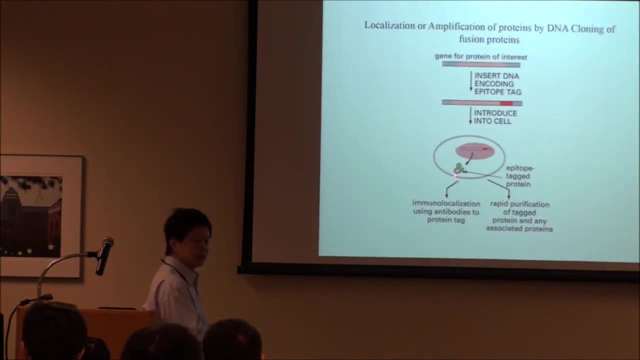 all the antibody from commercial available. you know you will pull down this whole protein out. right, you can put the beads onto antibody. the antibody will bind to this hybridized protein and pull out this protein. you can analyze the function of this protein. is it clear? you don't need 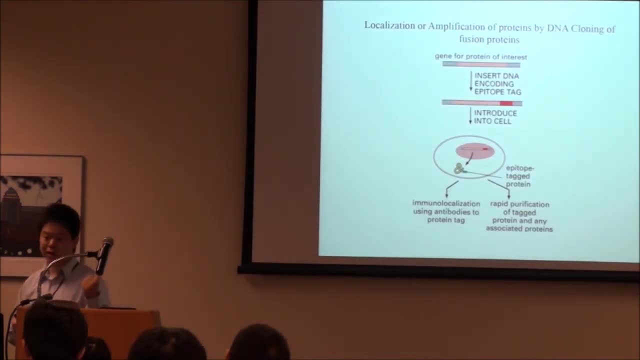 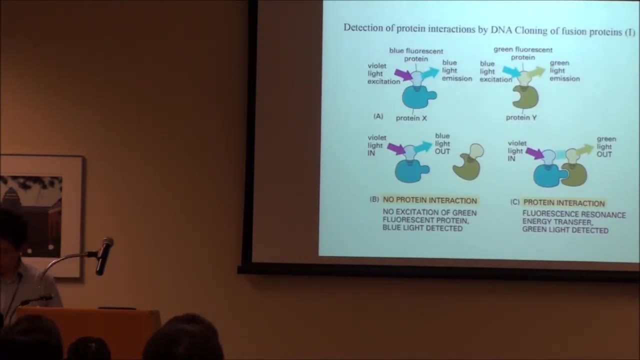 to create antibody in your lab. okay, that's one way or really help you a lot, right? another way is if you want to study the protein, for example, you want to know whether protein A or protein B are intact. in this case, protein X and protein Y are intact. 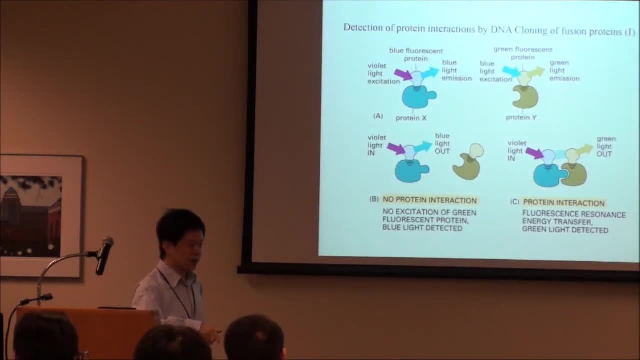 into each other in the cell. how do you do it? you know you cannot directly use antibody, right, because current microscope resolution is 200 nanometer, right, and the protein obviously are much smaller than that. if you use two color antibody to label to each other, right? it's just like. 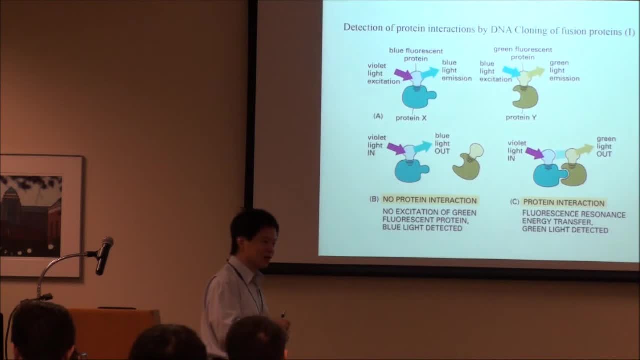 two protein or two person in the building doesn't mean they are in the same room, okay, so I have limited time. I will just quickly go through. what you can do using genetic engineering is you can using DNA, like encoding a blue frozen protein together, so create a hybridized protein. 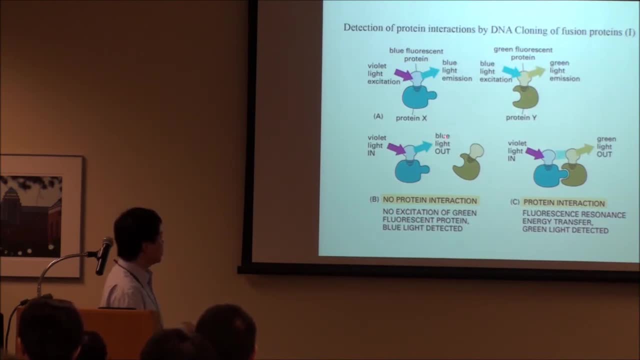 and this is a green frozen protein hybridized together and these two proteins you can put in the cell. if these two proteins, XY, doesn't interact to each other, you excite this blue frozen protein. you will see a blue color only after this XY interacting to each other. 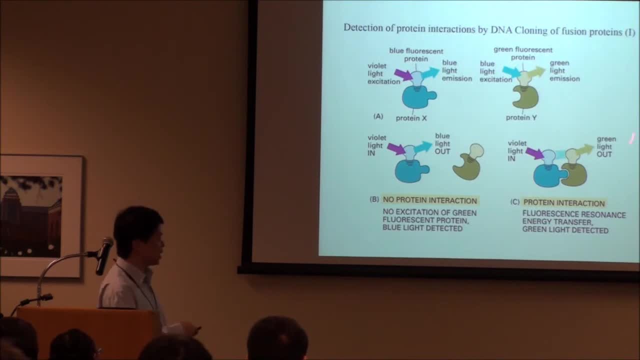 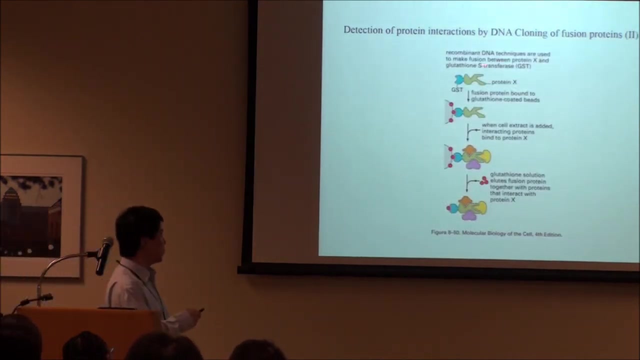 exciting your blue frozen protein. you will see a green color out. okay, if you see a green color out, you know these two proteins are interacting to each other. if you see a blue color out, you know these proteins are not interacting to each other. very simple, right genetic engineering. 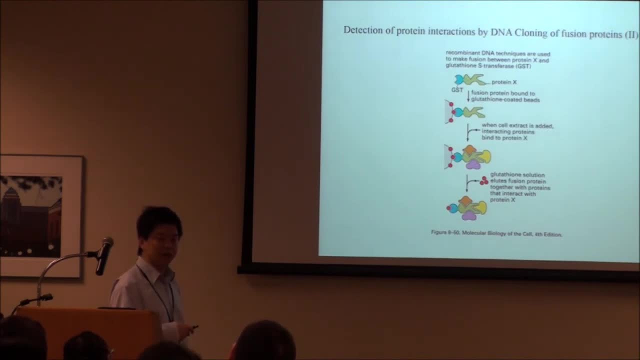 can help you to do that. you have antibody available for it and you want to study the protein interacting with this protein X. how do you do it? genetic engineering can help you to do that. you fuse a GST tag to a protein X- okay, and there are antibody available. 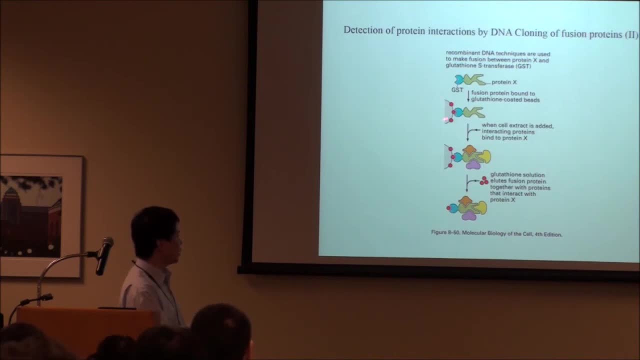 direct against GST and these beads and antibody can bind to this and pull down this protein. right, and there are a lot of proteins, of course, associated with protein X already and when you pull down this whole thing, the protein associated with protein X also being pulled down by this protein. 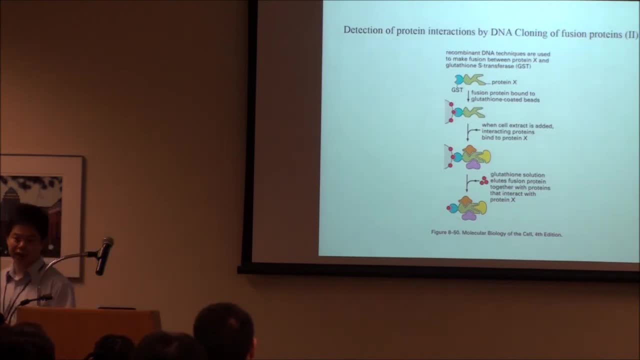 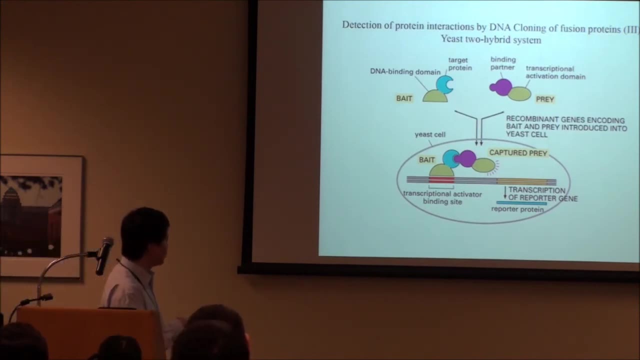 associated with protein X, although you don't have antibody against protein X, okay. or if you want to study a protein interacting, you can also using, you know, so called yeast two hybrid system. okay, again, these bait and play are the protein which controlling the gene regulation? okay, and this protein. 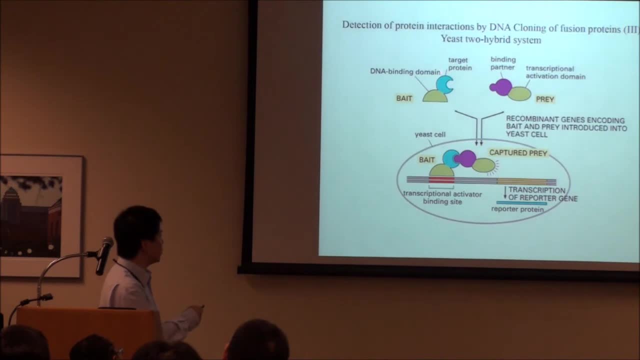 let's say X and Y. you want to know whether they are. you can create this using genetic engineering. create these two hybrid protein. this bait will bind to DNA and this play will start to. you know, regulate the gene expression only when these two proteins interact with each other. 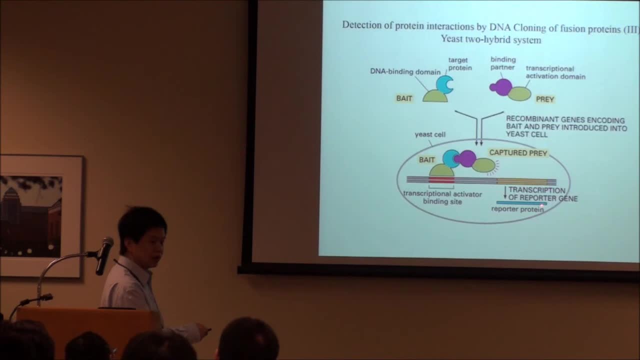 they will be functional to create protein. okay, colored protein, for example, you can generate. if they don't interact with each other, they will not create this reporter protein. another case: right, you can use genetic engineering to help you to study whether these two proteins interact with each other. 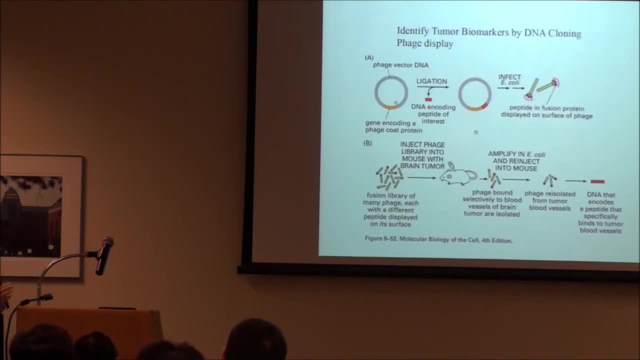 okay, I think last case I think the most wonderful. you know, application in genetic engineering is so called phage spray. okay, for example, if you have a specific tumor or cancer you want to detect or you want to inhibit, how do you do it? now, people can help you. 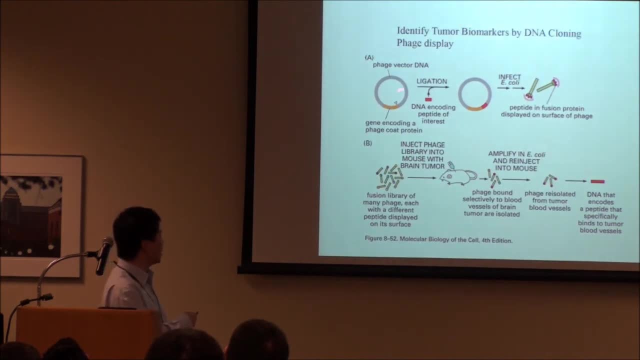 do that, you first using genetic engineering to create a library of the genes. okay, people can do that. so the different genes encoding different peptides and they can be expressed into, for example, Ecoli or yeast. they will be on the surface. so Ecoli, yeast, okay. 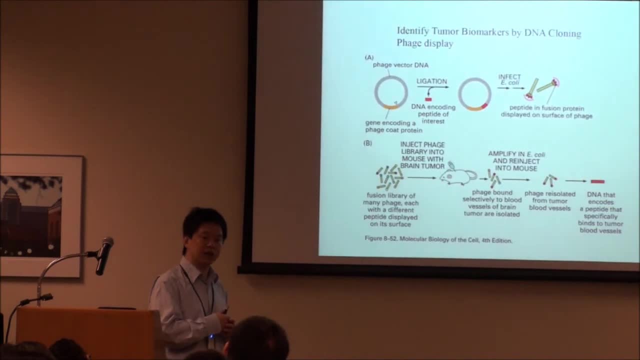 so you can imagine, if you create a library of the DNA, you can create a library of yeast or bacteria. each single bacteria or single yeast contain a different peptide. on the surface is it clear? millions of peptides you create. now you inject into mice. okay, only these bacteria. 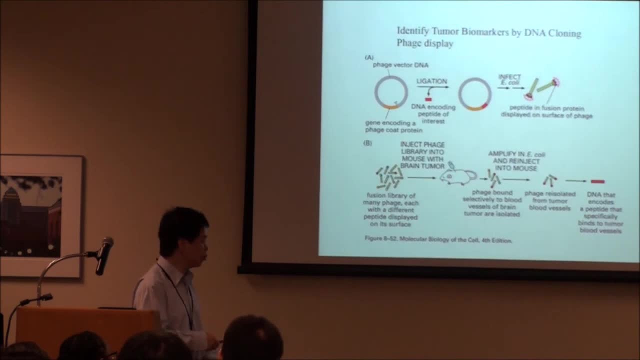 or yeast express. the intacting peptide will stay in the tumor. all the other yeast or bacteria will be washed away in the body right, if they don't intact with the tumor. is it clear now you harvest the tumor, you can. you can extract the bacterial yeast, you know. 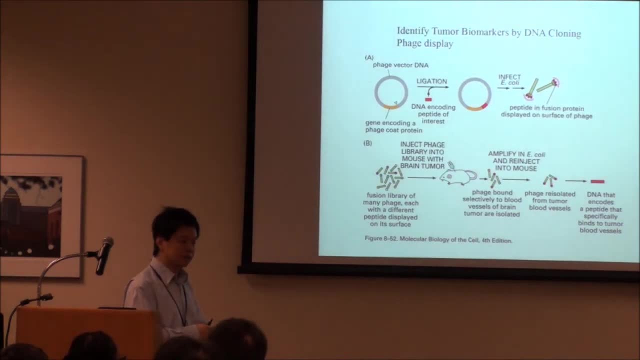 these bacterial yeast, they intact with the tumor, which means the peptide on the surface of this bacterial yeast are intacting with the tumor. okay, and if this tumor become shrink, you know this peptide can specific inhibit tumor shrinking. okay, and you know what kind of gene encoding these peptides?